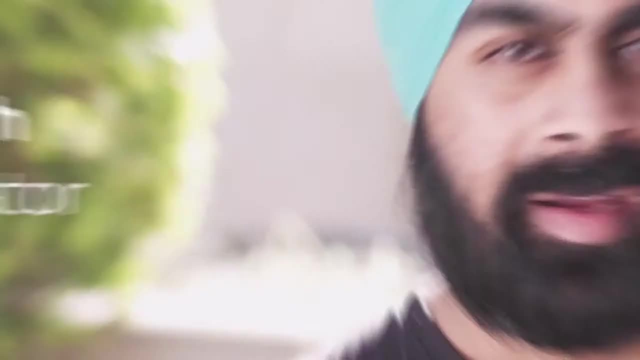 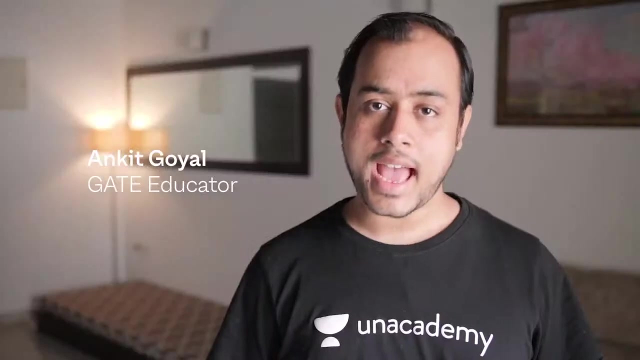 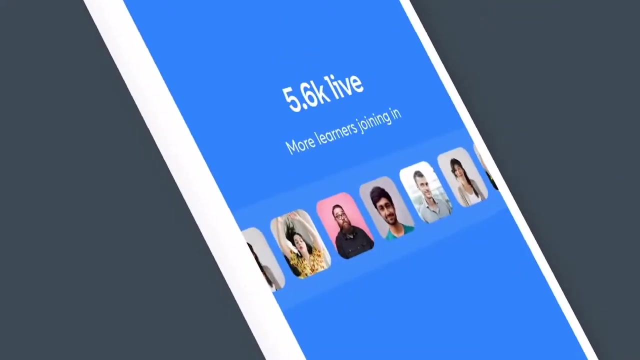 A challenging GATE contest engineered to give you an experience like none other, Where you put your knowledge to test and battle it out with the best to bring out the best in you. An Academy Comeback is the most competitive gamified contest for GATE till date. 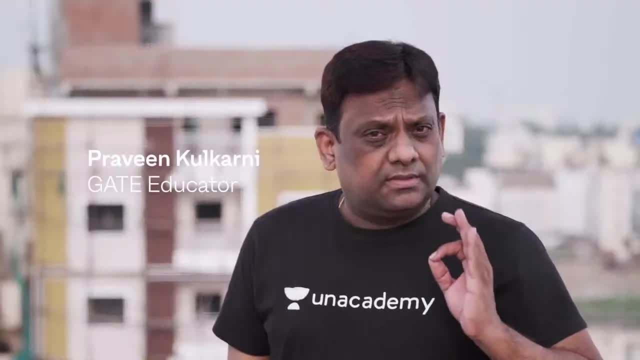 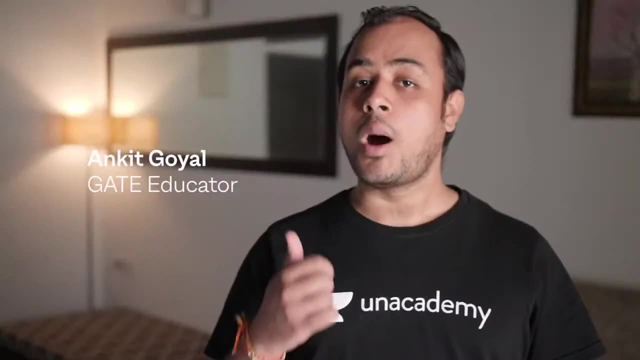 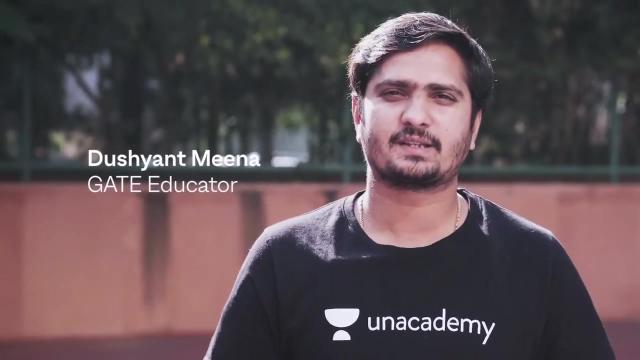 With the best of the questions by best educators, With detailed video solutions from top educators right after each contest. Combat live with peers to get real-time rankings and win big. Participate in every contest to improve your ratings, Challenging contests every fortnight or alternate Sunday. 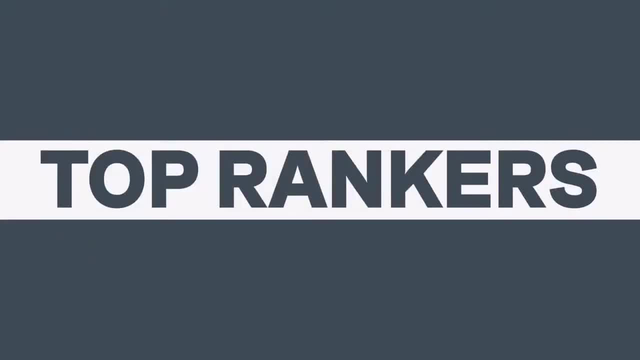 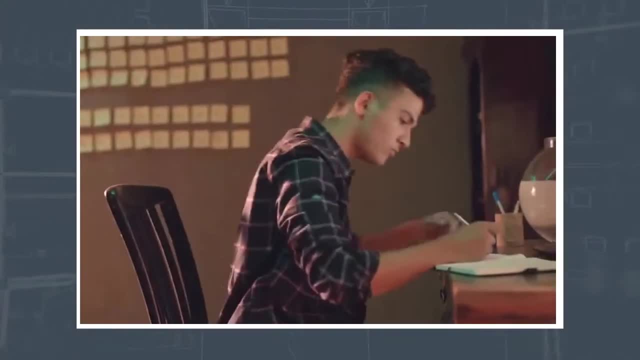 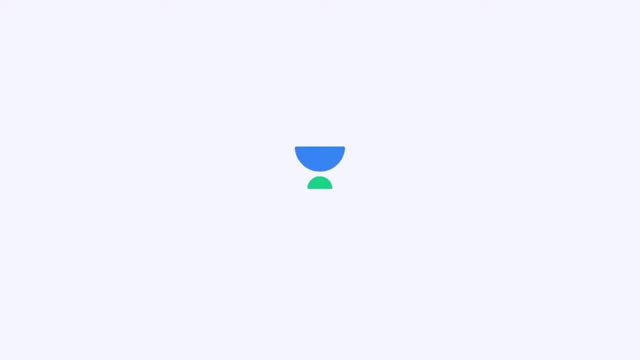 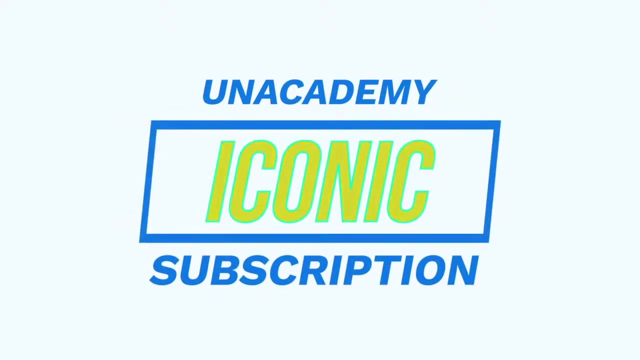 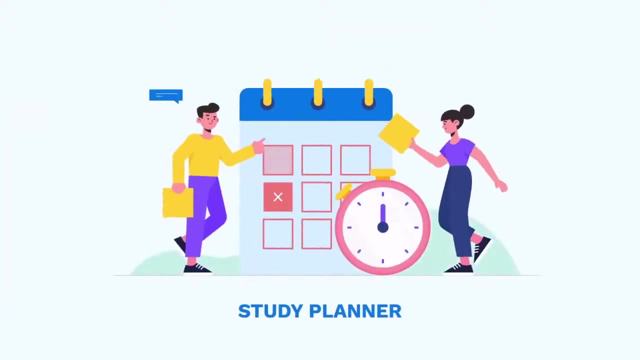 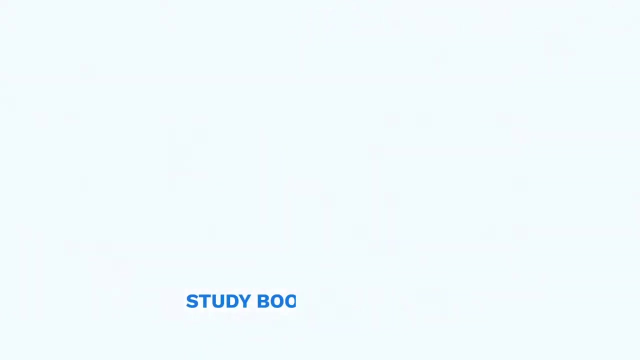 Live ranking after every question. Big rewards for top rankers. Your passion to crack GATE deserves this. Your hard work towards your dream deserves this. Fuel your inner fire for the ultimate GATE challenge: An Academy Combat Register now To participate in the GATE's contest. contact us at miclm wwweukiaacuk. 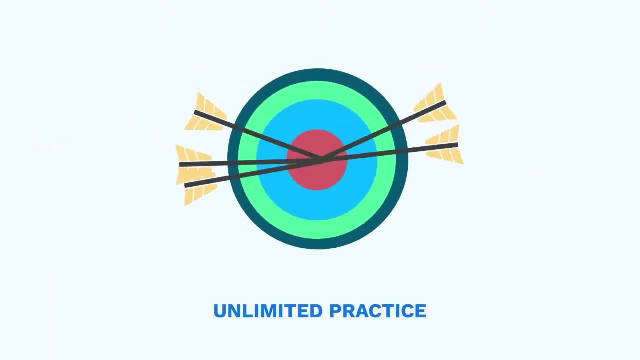 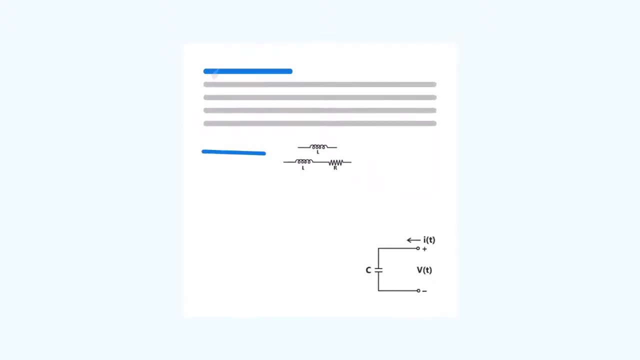 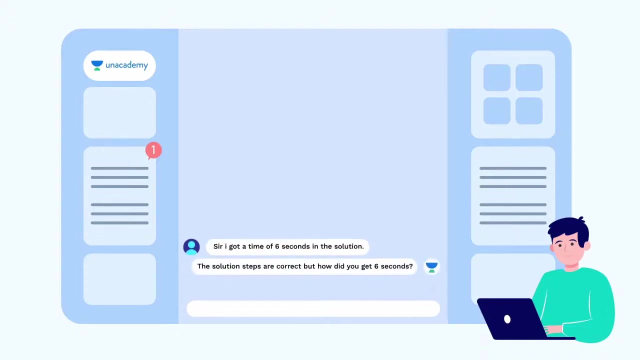 To become an Academy GATE. participant at a unofficial GATE contest ą To game, To win, To form the players, To educate them, To improve your skills in GATE competition, To invest in GATE, To know the GATE. 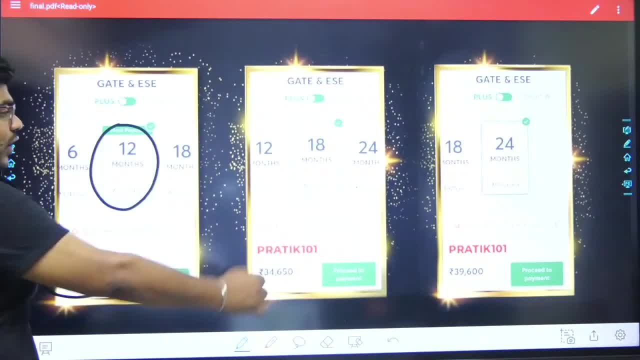 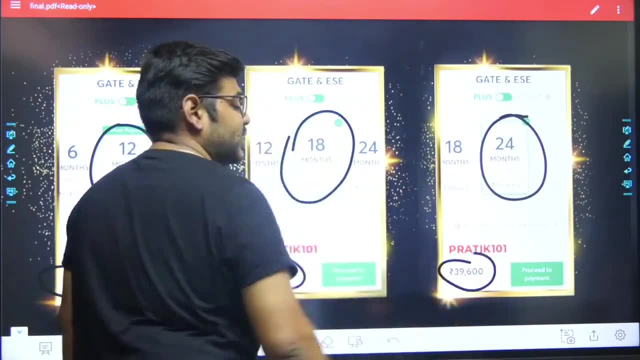 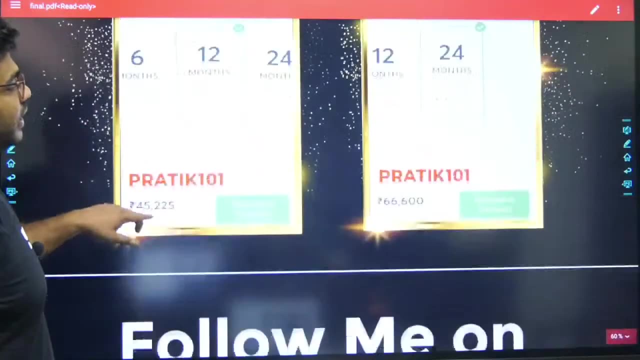 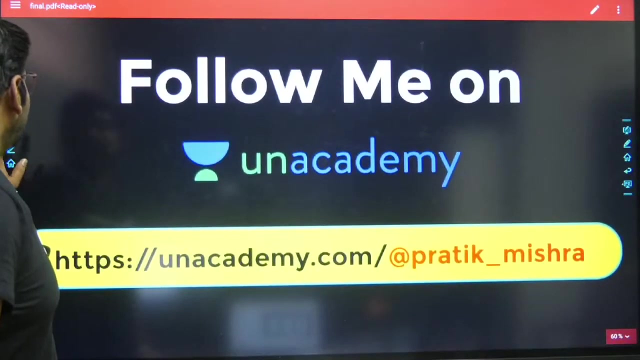 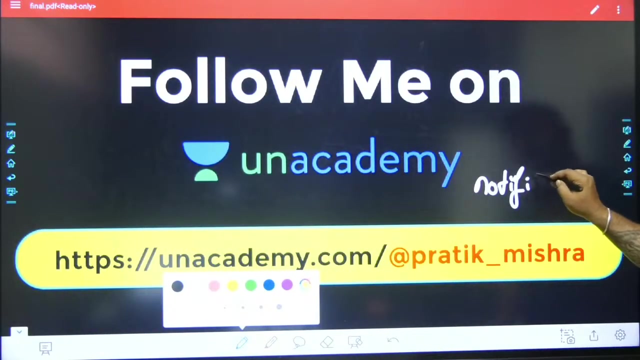 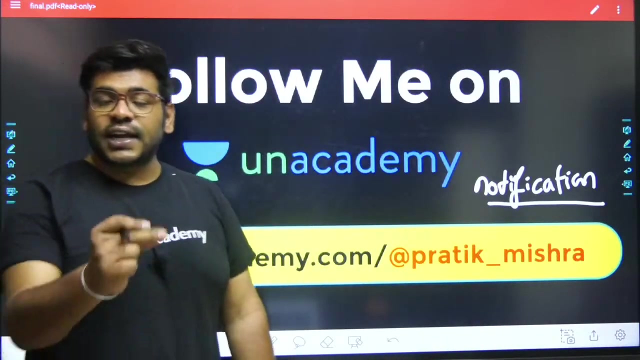 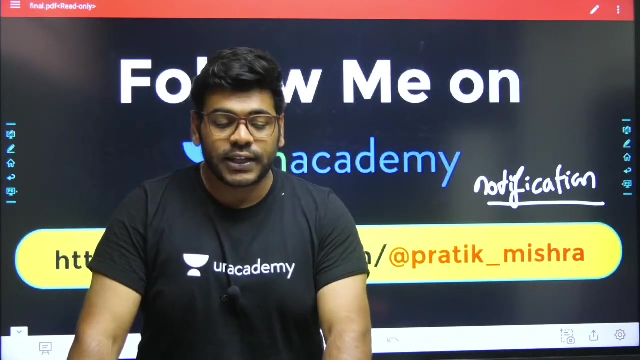 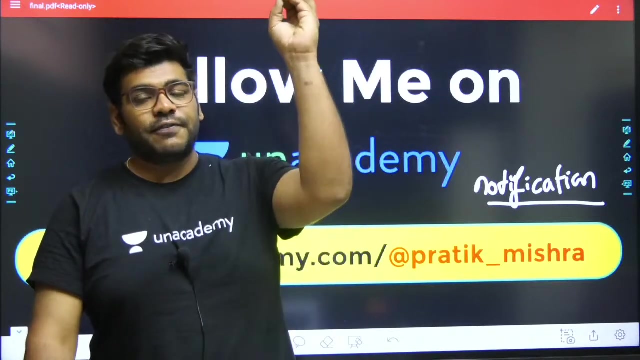 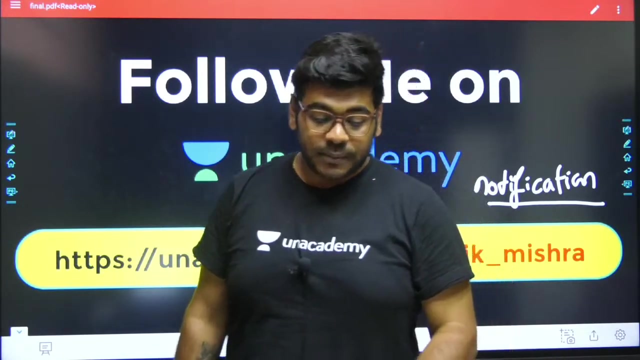 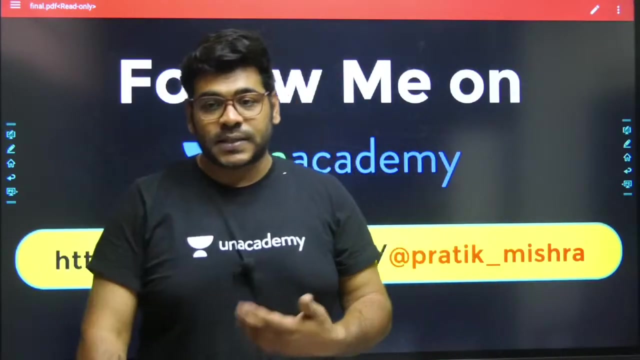 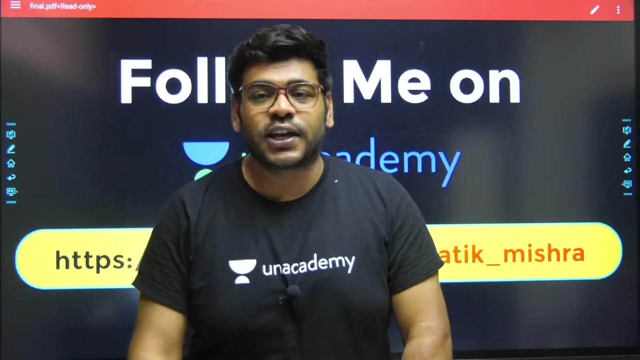 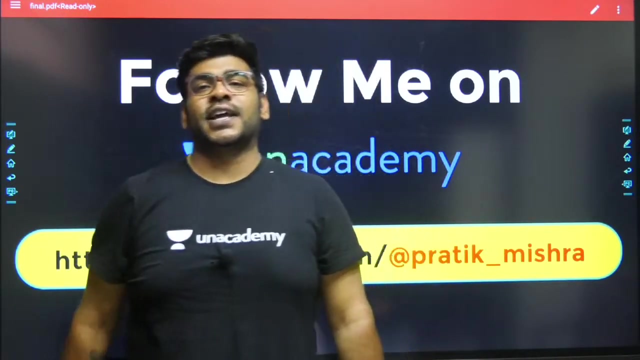 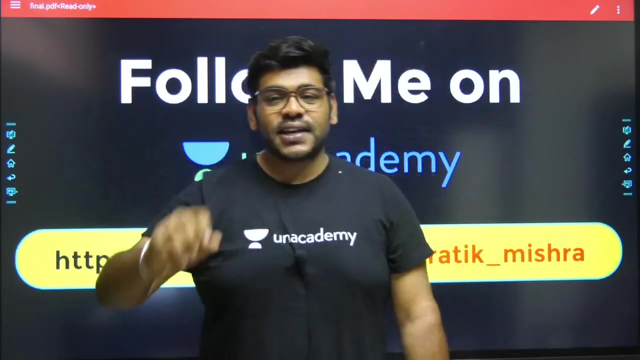 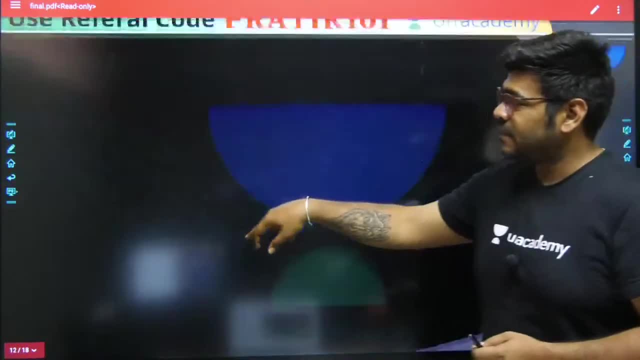 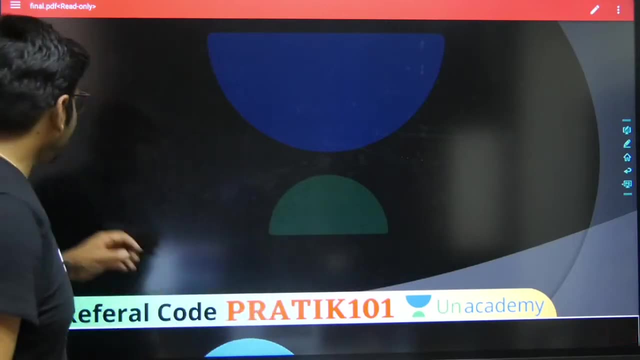 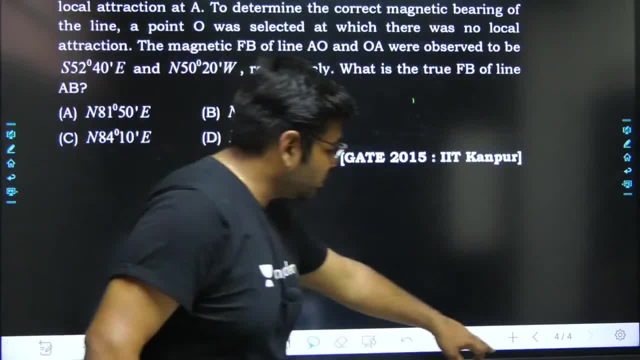 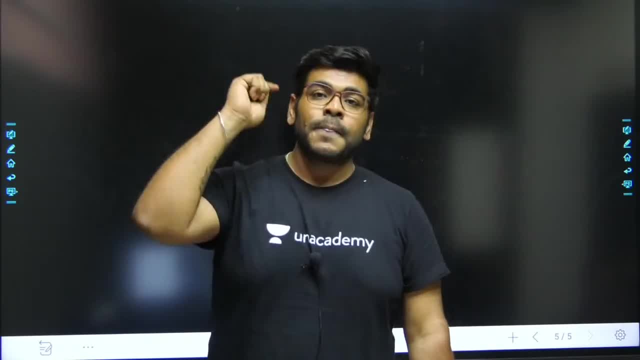 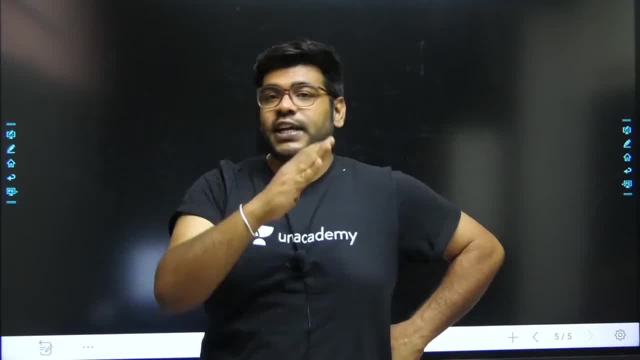 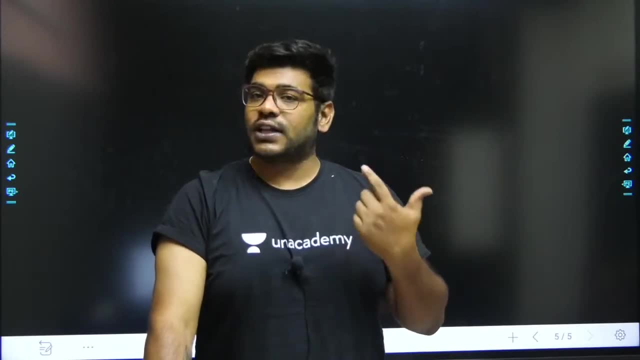 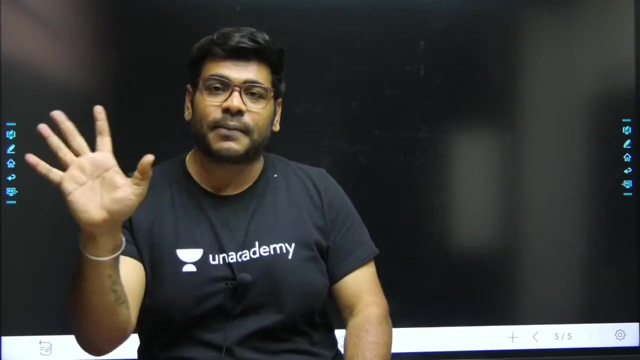 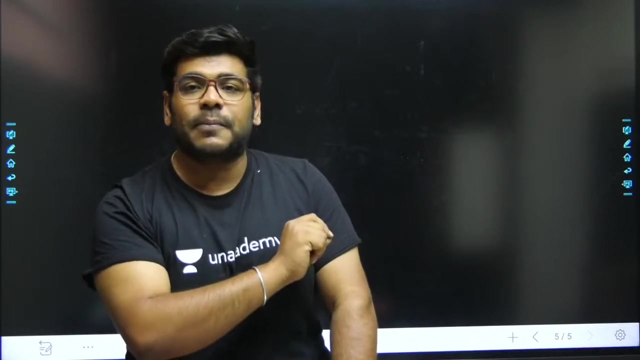 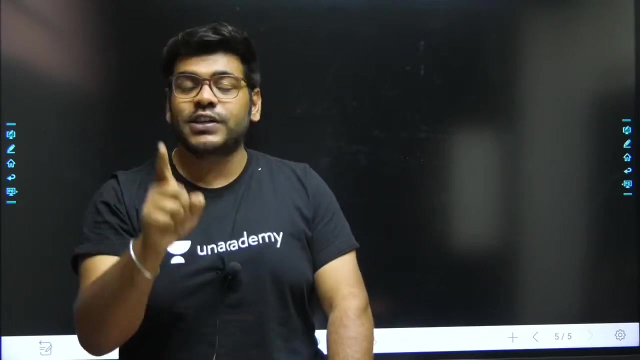 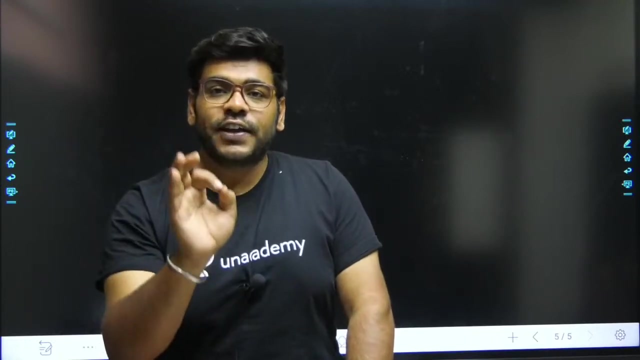 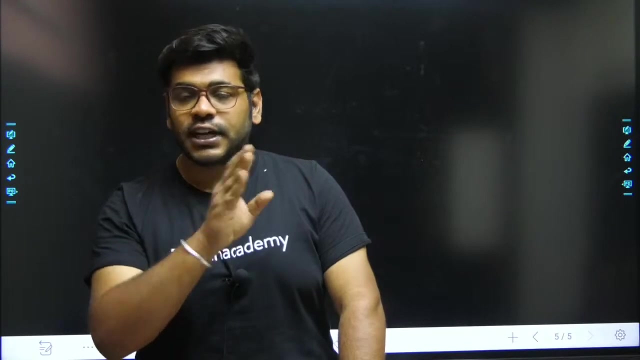 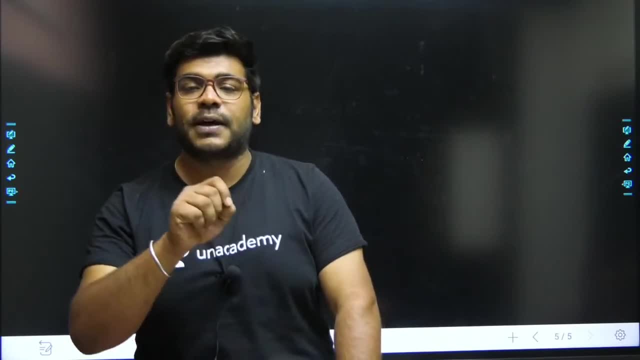 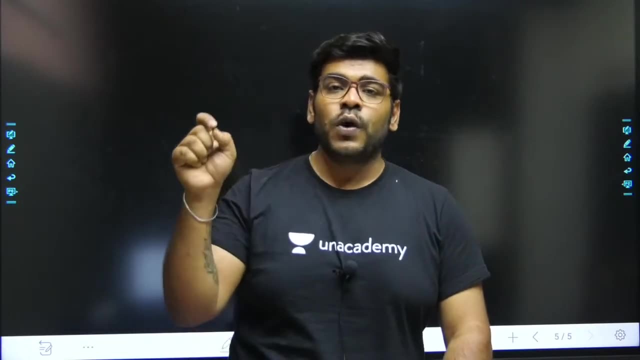 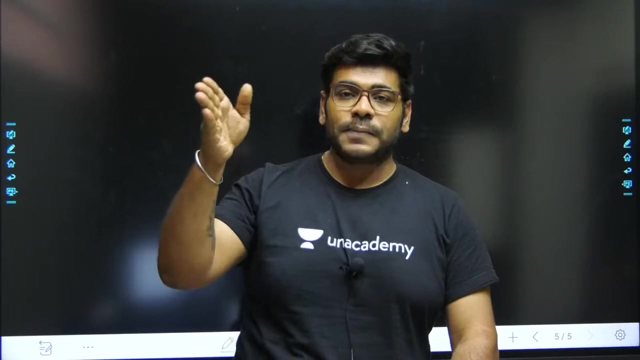 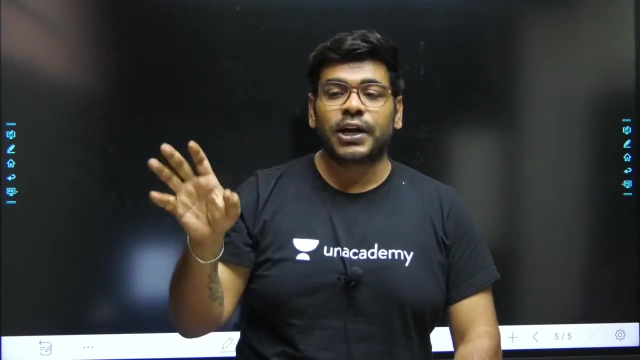 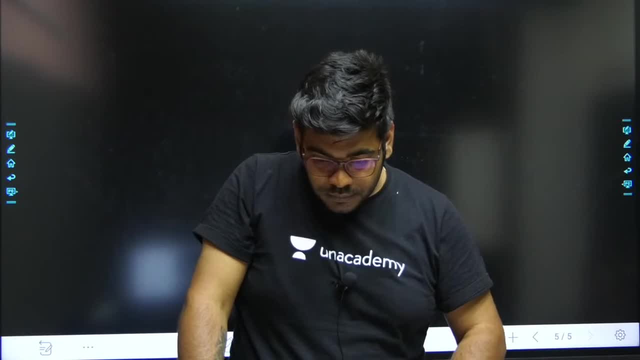 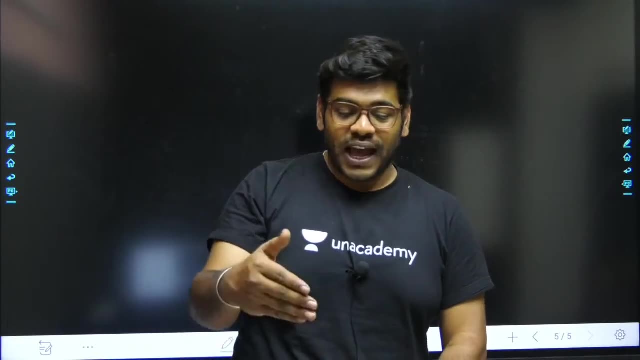 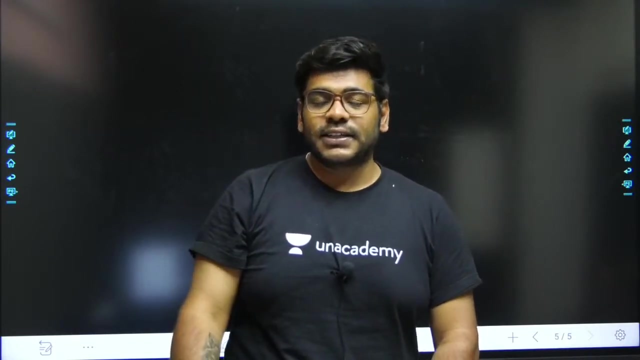 Okay, so what are you doing here? so what are you doing here? so what are you doing here? Okay, so what was I talking about? I was talking about the green shield model. I had said in the green shield model that if any green shield model is called from you, it tells you that. 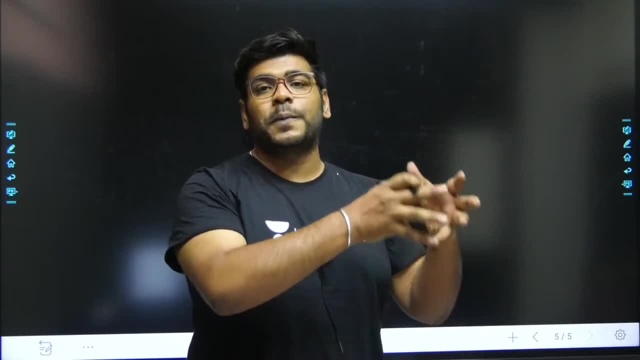 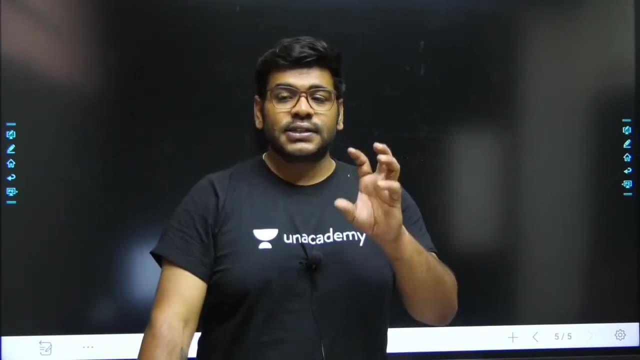 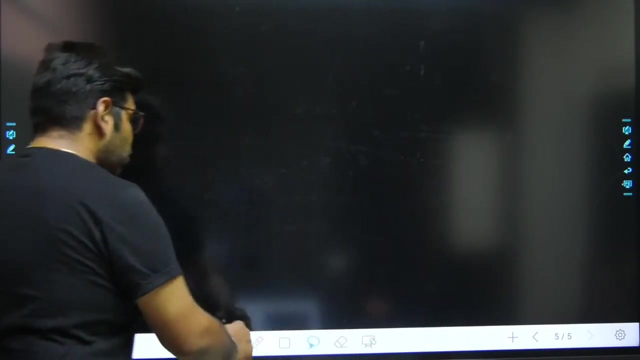 the variation of velocity is linear, or if anyone tells you that it is a negatively sloped straight line. So in all three cases it would be like this. so in all these cases, okay. so when I say Qめxlinear velocity variation, I said This is Vsf by 2 multiplied by Kj by 2.. 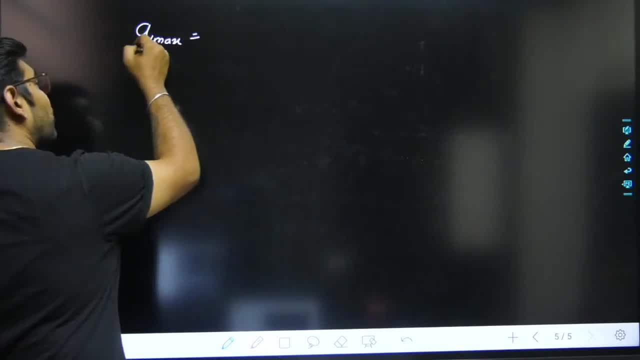 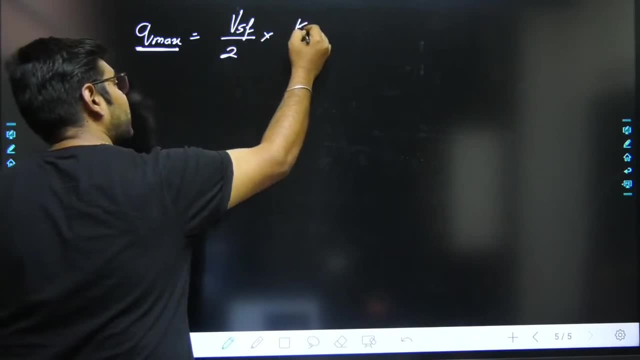 So, from here, when I talked about the Q makeup value or the linear velocity, so I said: When we talked about Qmax, so we said that it is Vsf2 multiplied by Kj by 2.. So I had said that it is Vsf2 multiplied by Kj2 multiplied by Kj. 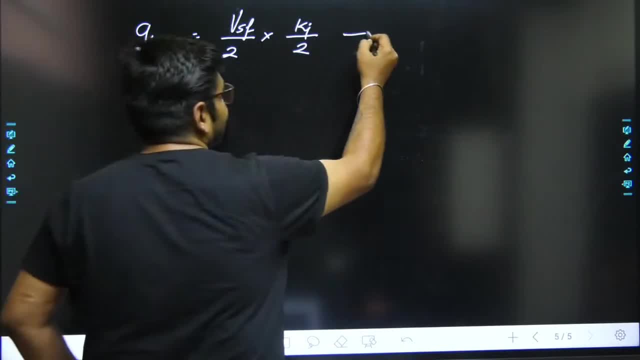 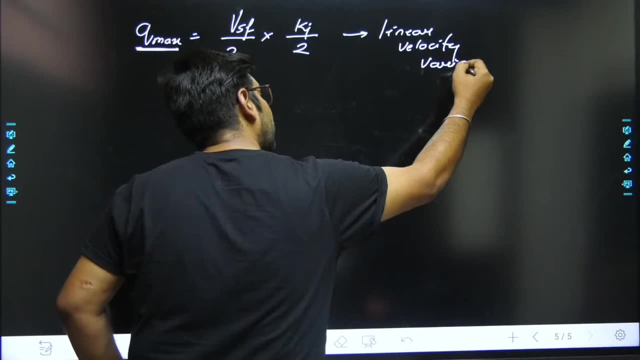 Alright. So that was that Alright by 2 multiplied by kj, by 2, for which I have said: whenever you talk about linear velocity variation, Means whenever you talk about linear velocity variation, then talk about this only okay, Means we talk about next. so when we talk about next, then I said next what I am talking. 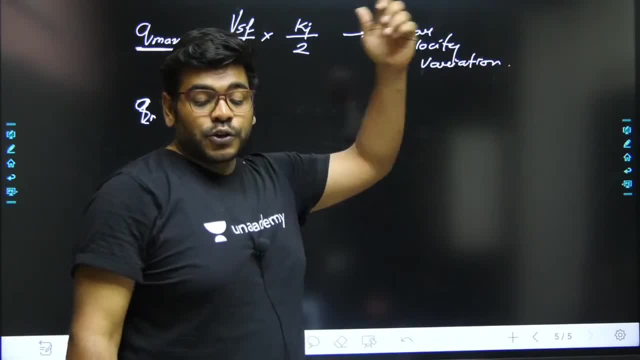 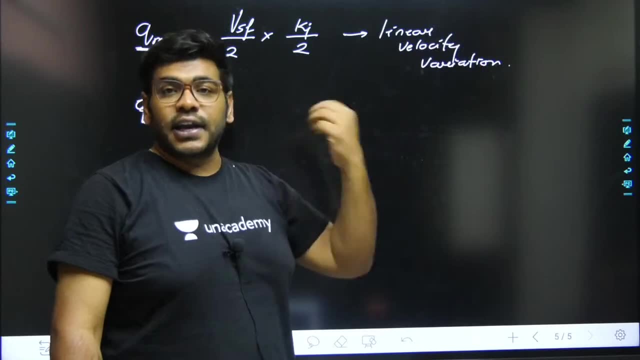 about is that this is green shield model. this is linear velocity variation. so next, you saw, it is logarithmic variation. next, we talked about logarithmic variation and we used to call logarithmic variation as Greenberg model, and when we used to talk about Greenberg, 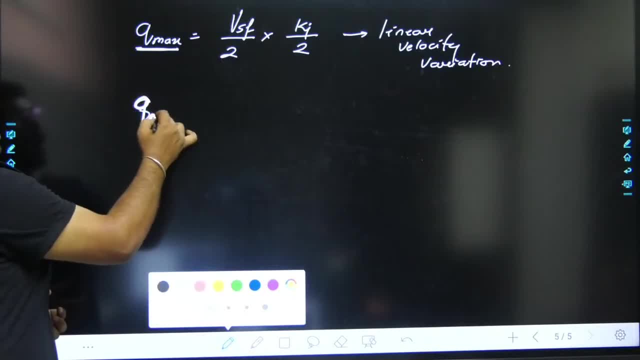 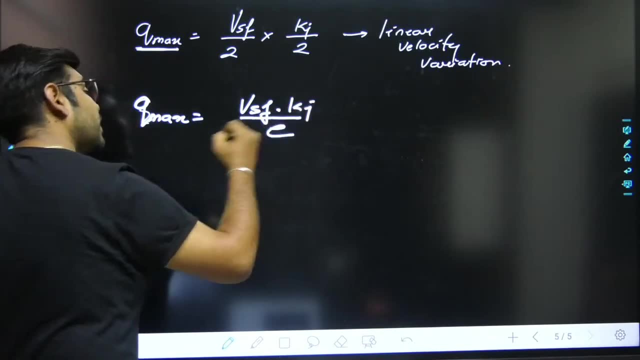 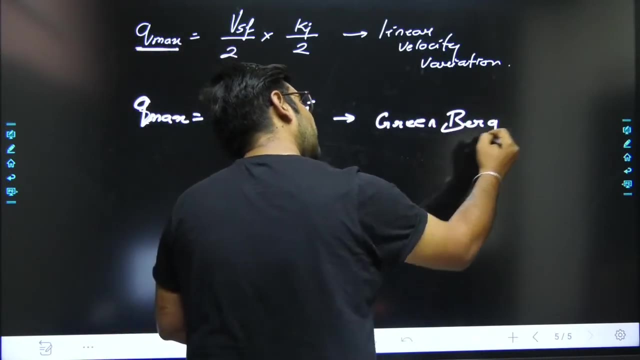 model and when we talk about Greenberg model there, Balv面, So you used to say it is equal to Vs f into KJ by e and according to whom we used to talk, You used to call Greenberg model this, and this was the same thing you used to call Greenberg model or logarithmic variation. 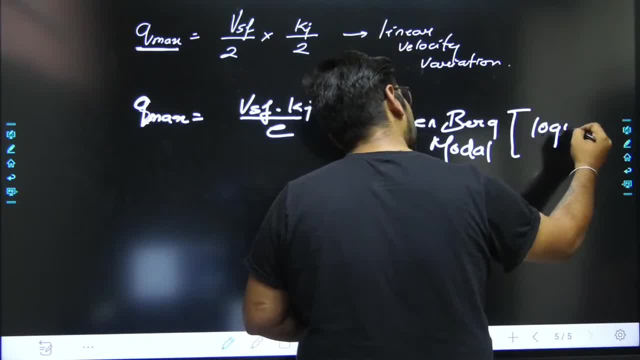 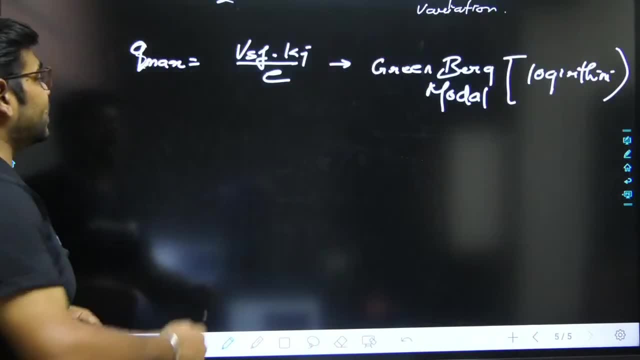 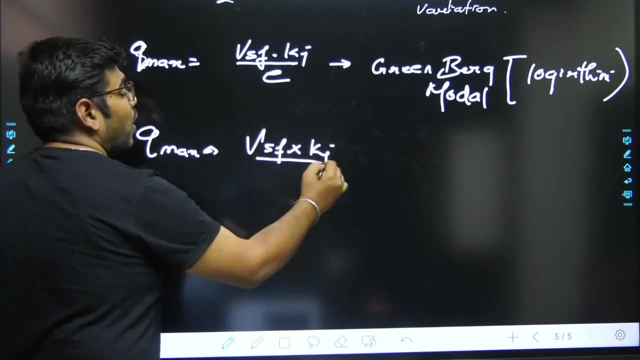 you used to call velocity og Down roll I was talking about. next, you saw Qmax and you saw the value of Qmax Vsf into Kj by E and for whom I said Qmax. I told you about this Underwood's model. I told you about this Underwood's model. 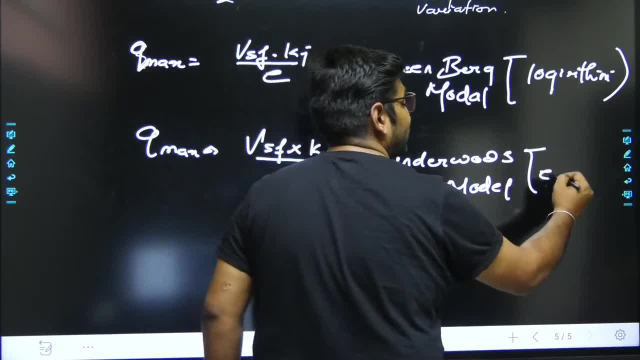 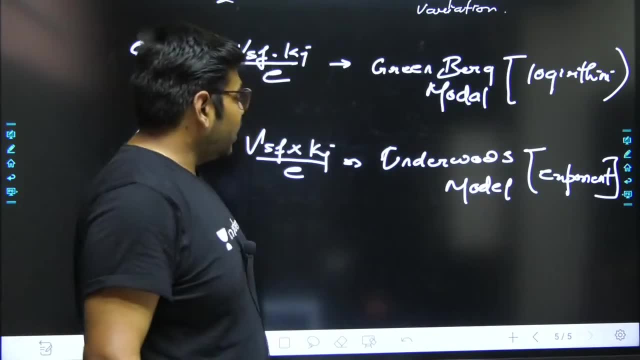 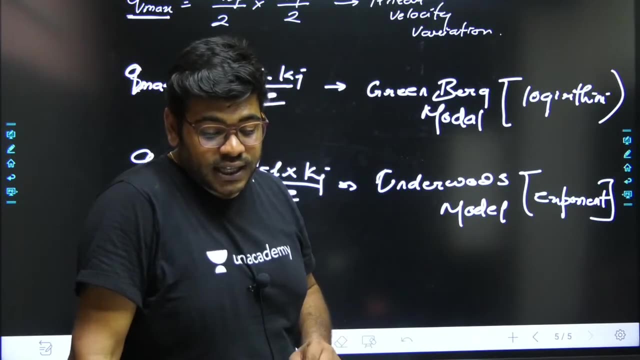 I told you about this Underwood's model, or you said that I talked about it exponentially. you talked about exponential velocity variations. what are you talking about? Vsf, Vsf. you have not seen yesterday's lecture, Pranao. if you have not seen yesterday's lecture, then you will not understand what is Vsf. 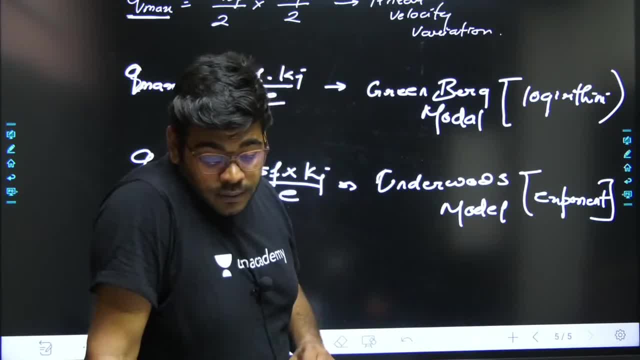 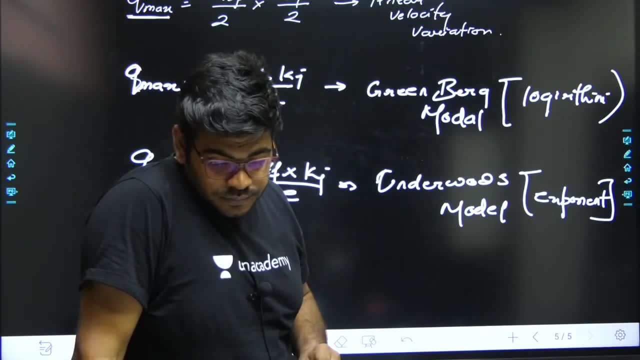 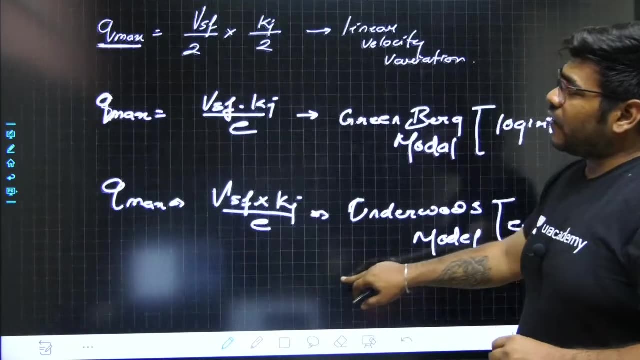 and to tell Vsf completely is not possible. ok, ok, come, let's talk. come, let's talk Pranao. once you see yesterday's lecture, you will understand what is Vsf Pranao. if you will see once, then you will understand yesterday's lecture. 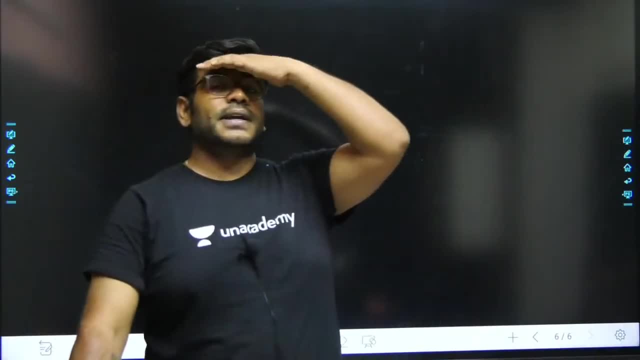 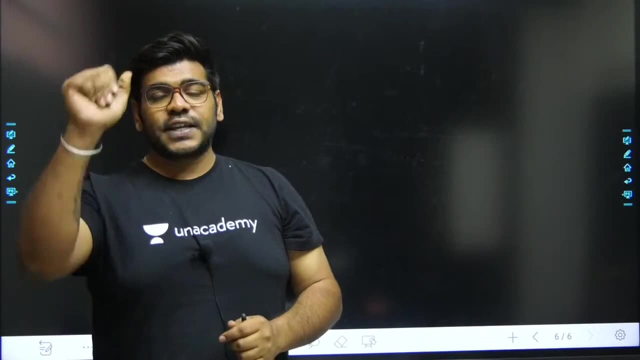 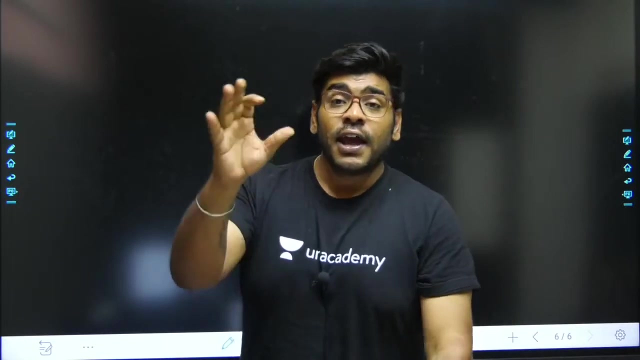 If you are talking about graphs, then where is Dilkhush? Come on, we are talking about graphs. Come on, we are talking about graphs. If I am talking about graphs, then see how I will connect the graphs. here. I will tell you three connecting graphs and the value of those three connecting graphs. 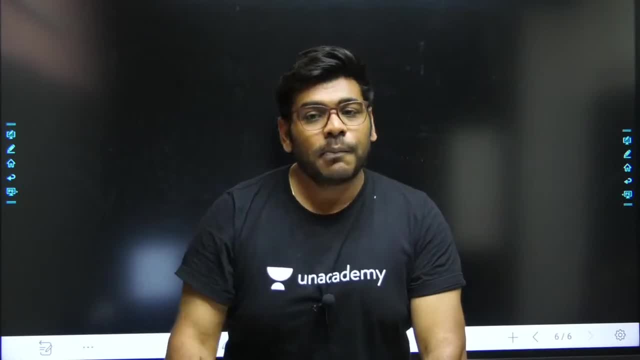 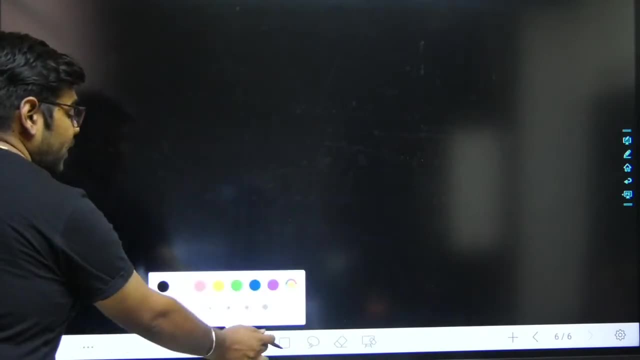 Why did they start from zero and why did they finish at zero? There is very little talk about this. so today we are going to talk about these graphs. Why did we finish them at zero and started from zero? So look carefully at these graphs. 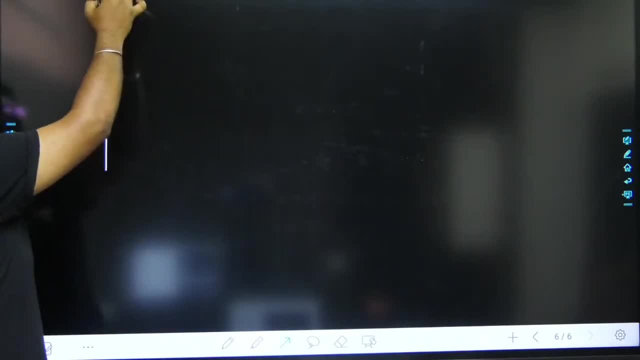 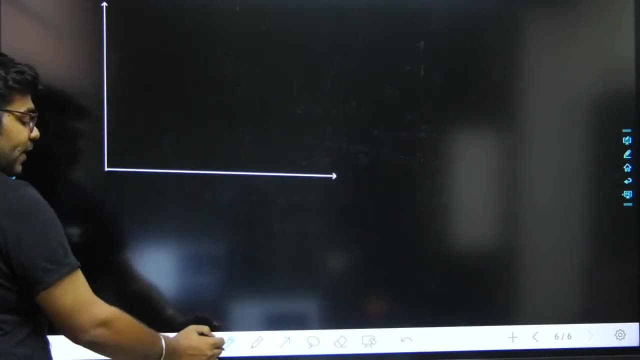 Can you make these graphs, And if there is any doubt anywhere, then tell me at the same time that sir did not come. Sir tell me again. So I said that, the first graph that you are getting to see. look carefully and forget the rest. 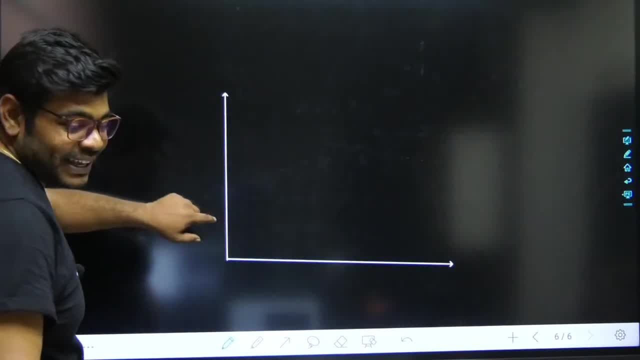 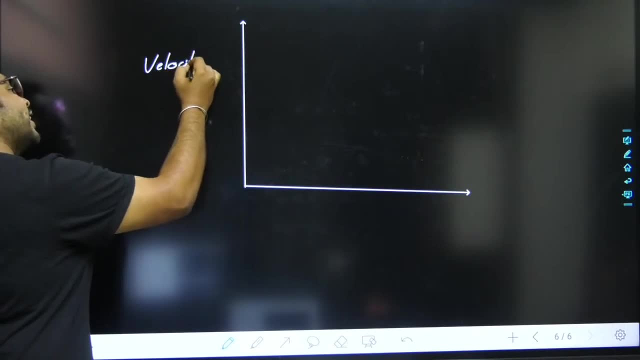 Forget the rest of the people. Yes, Abhay Pratap Singh is for you, son. Yesterday you had a spark, So I said that this first graph is between who? I said that this first graph is between your velocity and density. 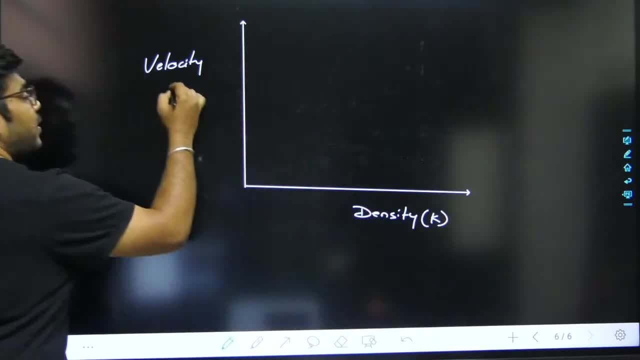 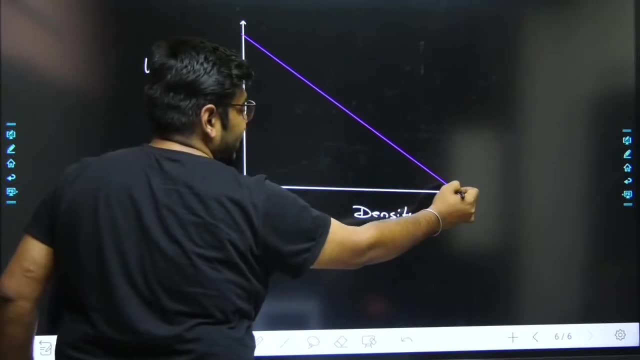 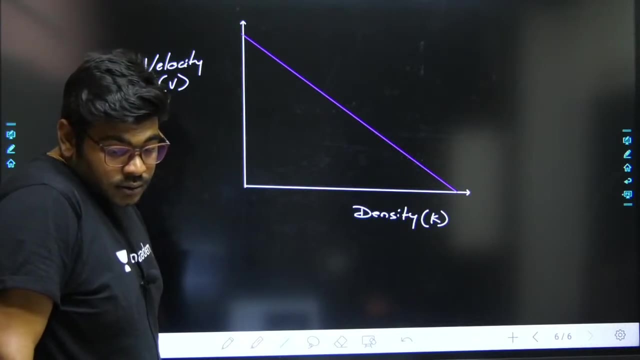 The first graph is between your velocity and traffic density: k and velocity. I mean you know that this graph is a linear, linear, negatively sloped linear graph. Here is the negatively sloped linear graph. So I said that I will talk to you about the negatively sloped linear graph. 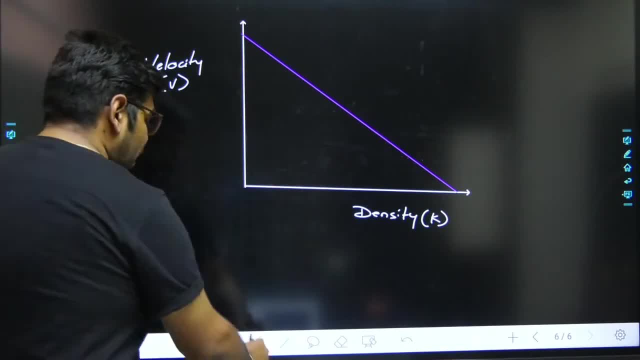 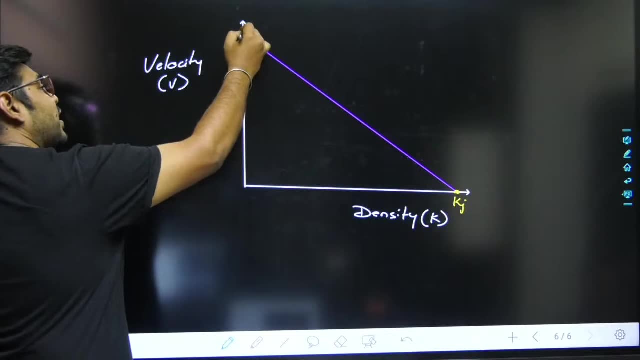 So this is your negatively sloped linear graph. You said that, sir, the maximum value that we get to see is the traffic density, Sir we call it kj, And the maximum value that we get to see here is the speed, Sir we call it vsf. 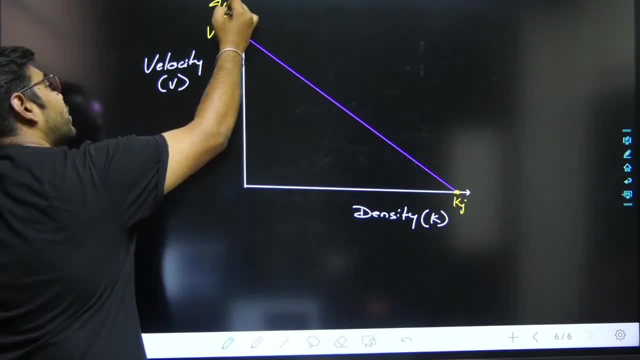 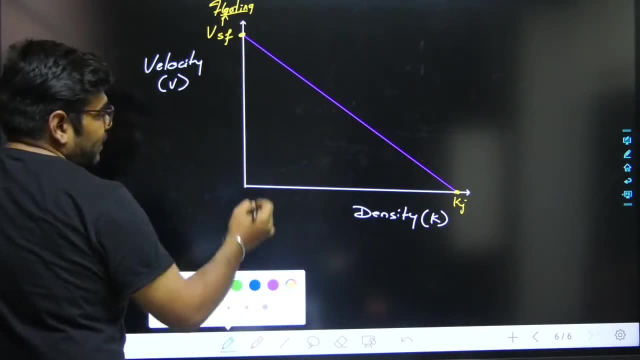 And, sir, we call it floating speed. Sir, we call it floating speed, We also call it floating speed. Okay, I said, sir, if you were talking about qmax, then, sir, can I say that you were getting. the value at v is equal to vsf by 2?. 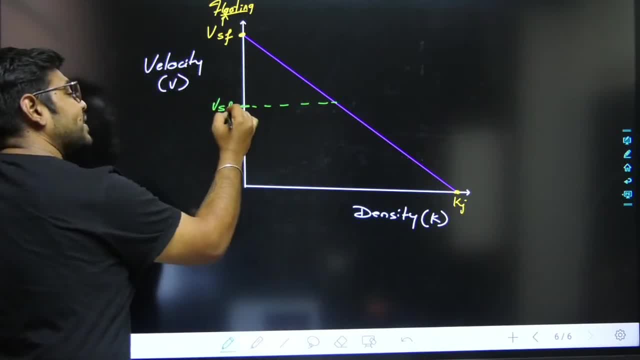 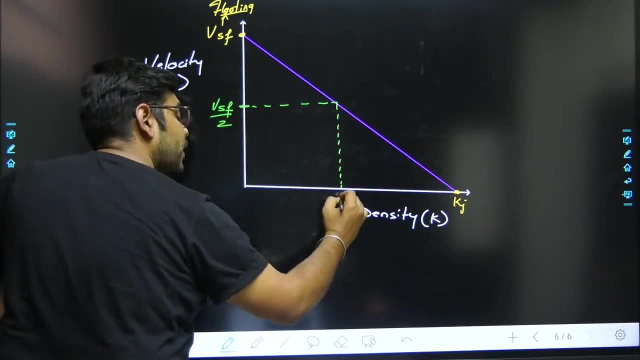 You were getting, the maximum value at v is equal to vsf by 2.. I said yes And you said, sir, k is equal to kj by 2.. If you were getting the maximum value at v is equal to kj by 2,, what was the value of the traffic volume? 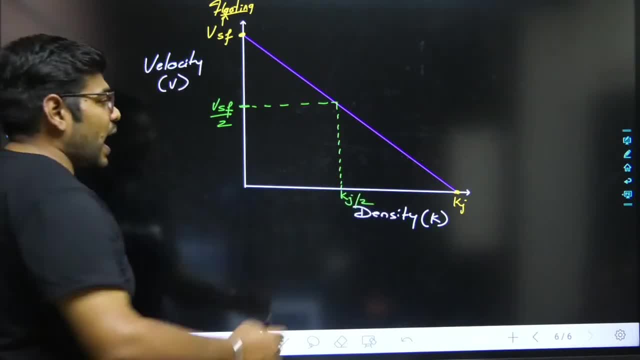 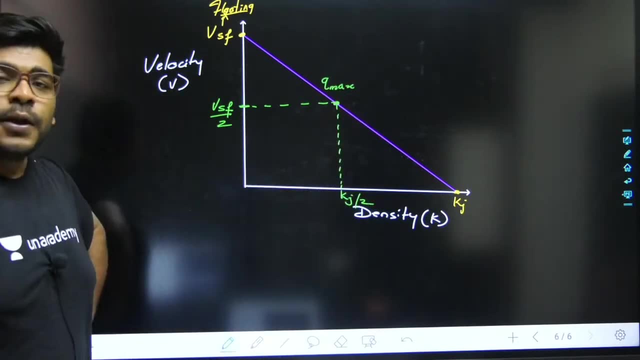 I said, sir, k is equal to kj by 2.. You said yes, So if you were getting it here, then this means that this is the point where you were getting q is equal to what You were getting, qmax. you said yes or no. 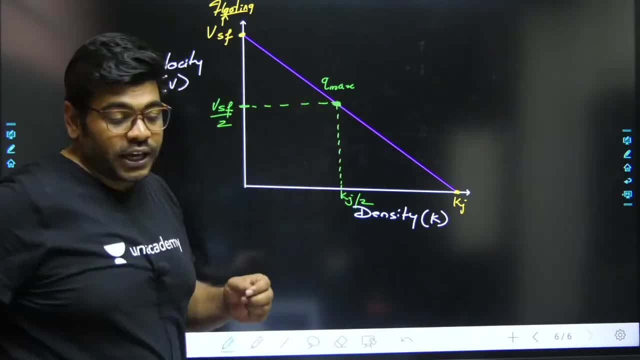 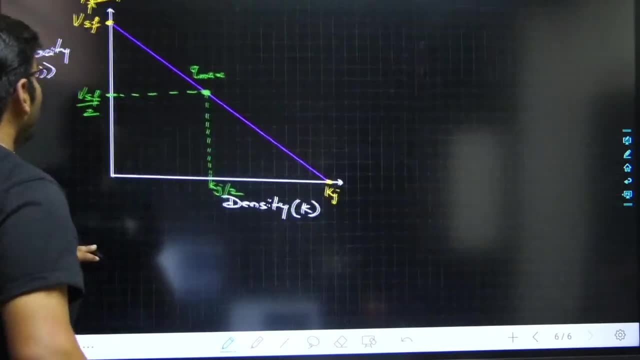 So I mean the point where you were getting qmax. this is the point where you were getting to see the maximum q. I mean, this is the point where you were getting to see the maximum q. So you saw this graph yesterday. 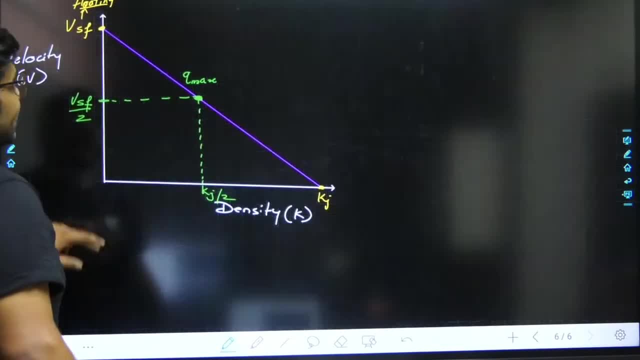 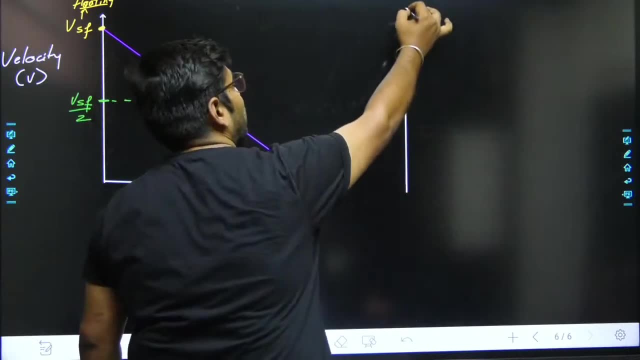 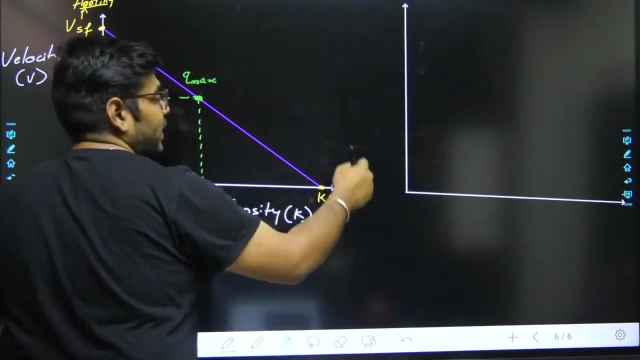 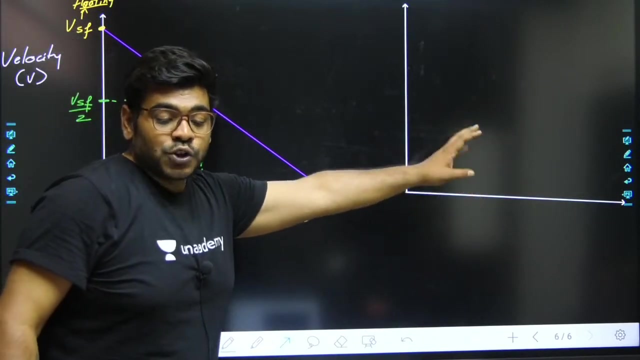 Now I am going to show a graph connected to this. look carefully, I am going to show you a graph connected to this graph, and this graph is between velocity and traffic volume. This graph is between velocity and traffic density. So the next graph you are going to see is between velocity and traffic volume. 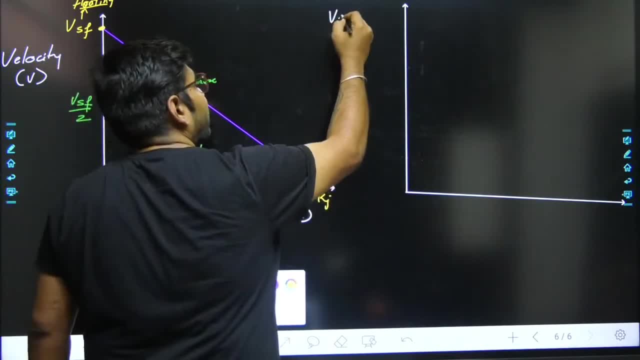 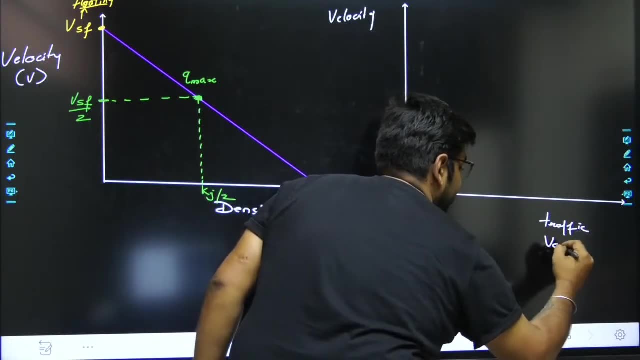 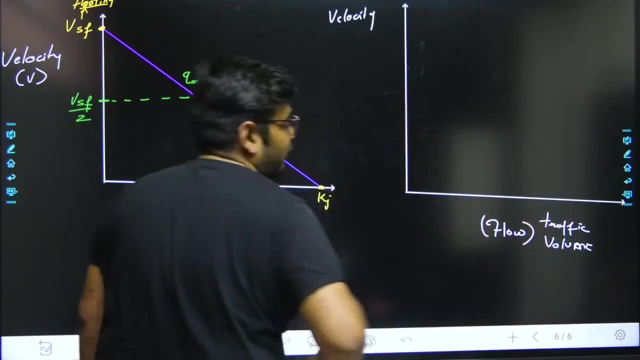 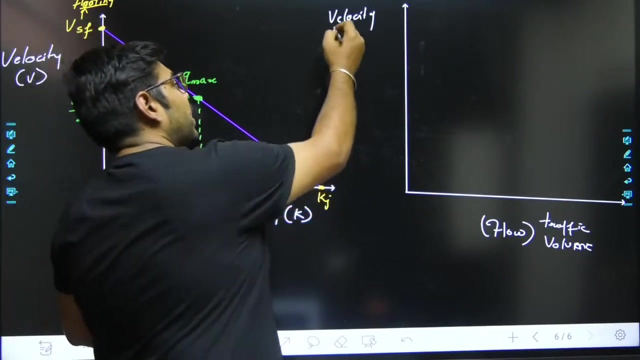 So I thought this graph is between velocity and traffic volume. You can also call it traffic flow, traffic volume or traffic flow. So this is between traffic flow and traffic volume. If we are talking about this graph, then look carefully. I thought: who is this talking about? V? 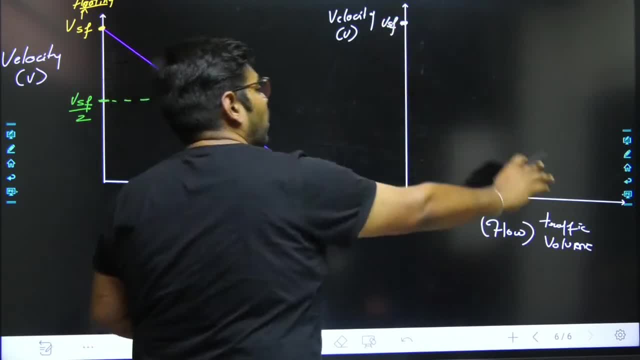 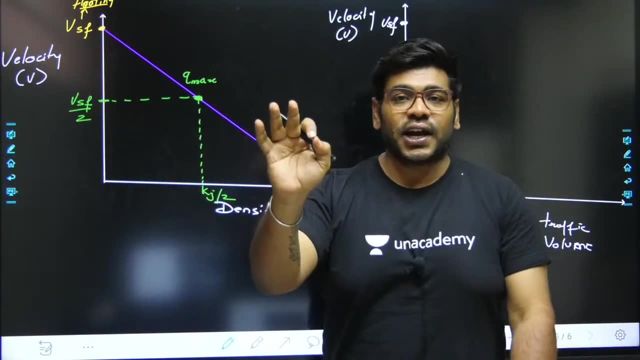 So I thought: who is this maximum point of yours? This maximum point is Vsf And I will show you the maximum point of traffic flow now. Come on, So everyone listen to me and keep an interactive session. You will have to answer the question I will ask. 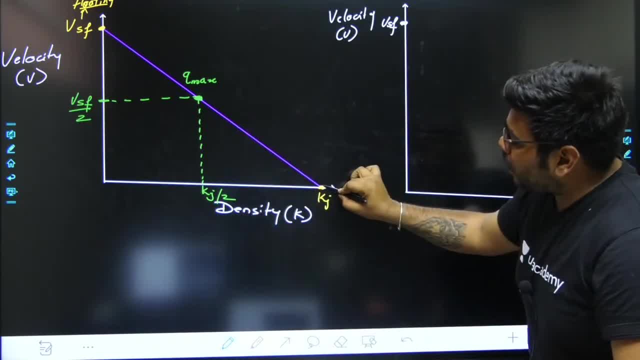 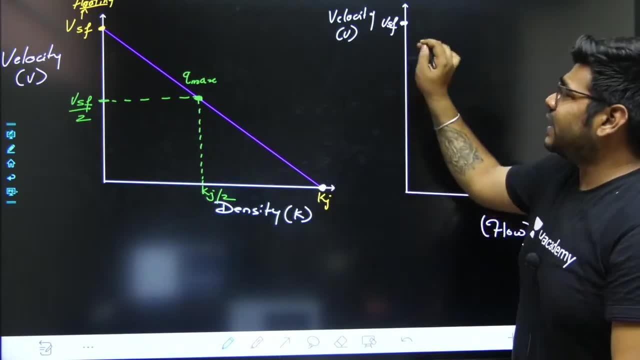 And I said the answer, When we are talking about K is equal to Kj. when I am talking about maximum density, then at that point of time, what will be the value of velocity? I said when I told you that your K is equal to Kj. 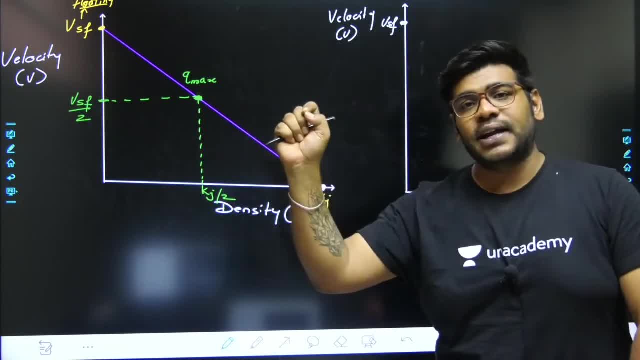 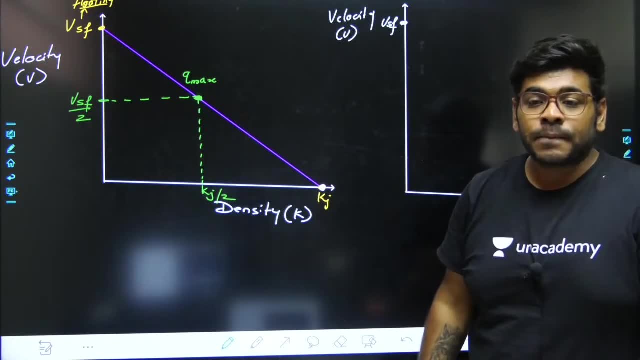 or your density is maximum, that is, jam density. then what will be the value of velocity at that time? what do you think? So, what will be the value of velocity at that time? what do you think? Zero, Very good. So those who are not understanding that there will be zero velocity. 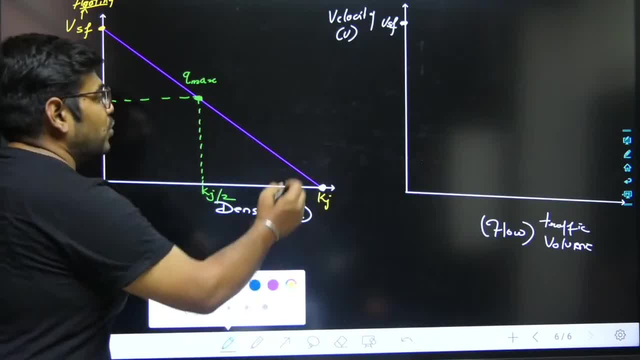 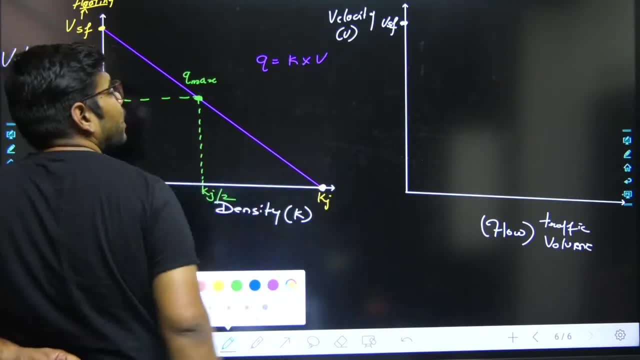 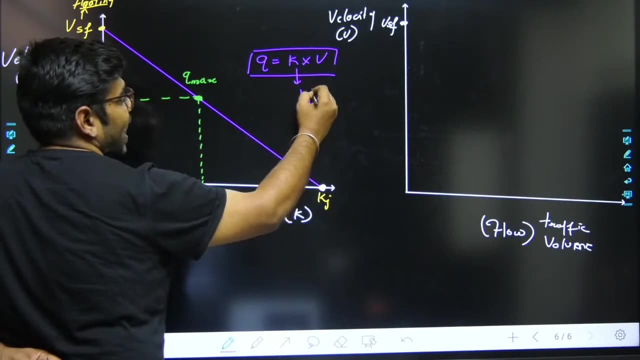 look at this expression and try to talk to me. I said: do you know that Q is equal to K into V? Q is equal to K into V. And I said: if this K is equal to Kj, if this K is equal to Kj. 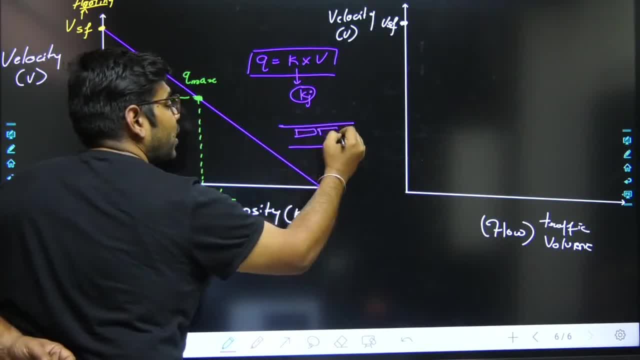 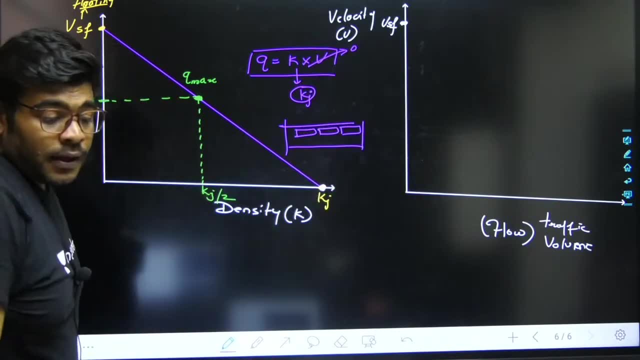 it means that no one is able to move on this particular lane. And when no one is able to move on this particular lane, then it means that this velocity tends to zero, Yes or no? So it means that you will understand that your velocity will tend towards zero. 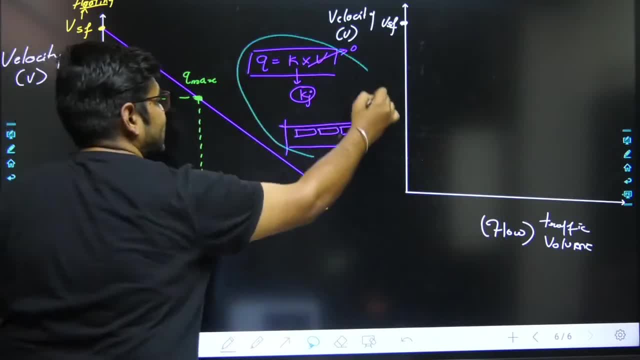 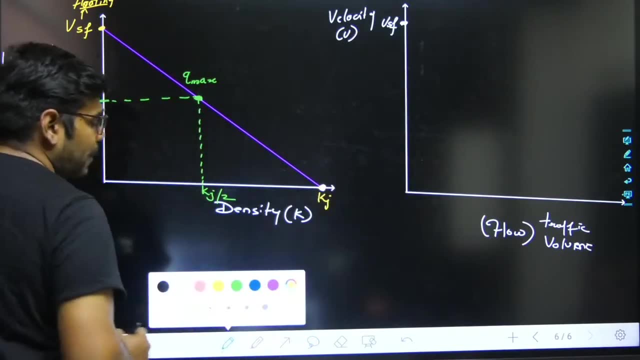 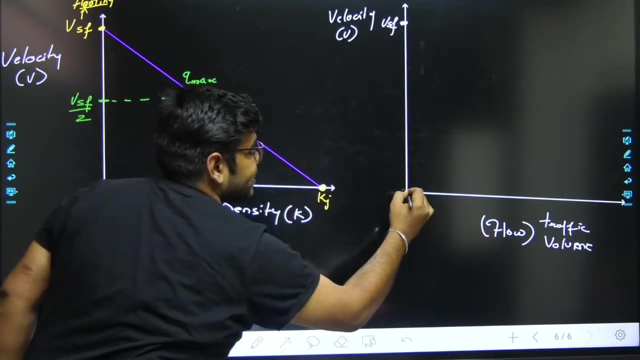 Okay, If you are so smart that you understand all this, if you are so smart that you understand all this, then you understood, and you understood that, at the point of time at which your k is equal to kj happened. at that point of time, the velocity became equal to zero. 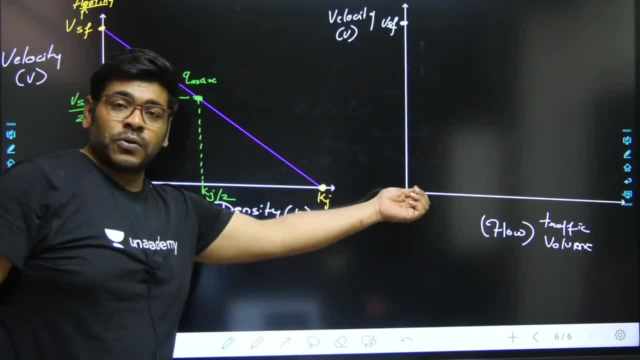 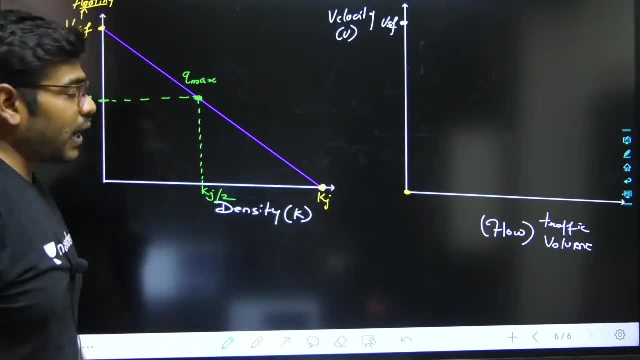 Say yes. at that point of time, velocity became equal to zero. Fine, At that point of time, the velocity became equal to zero. Okay, If you understood all this. so the next point that I am going to ask you about is: 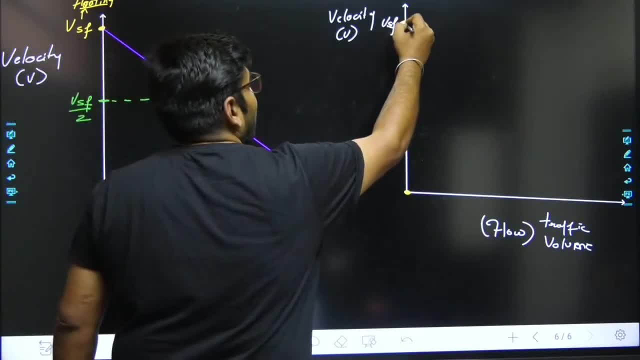 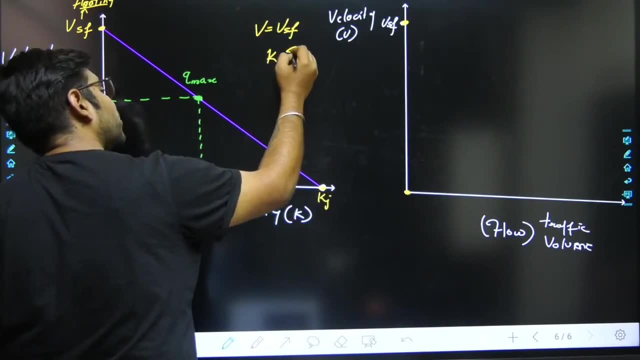 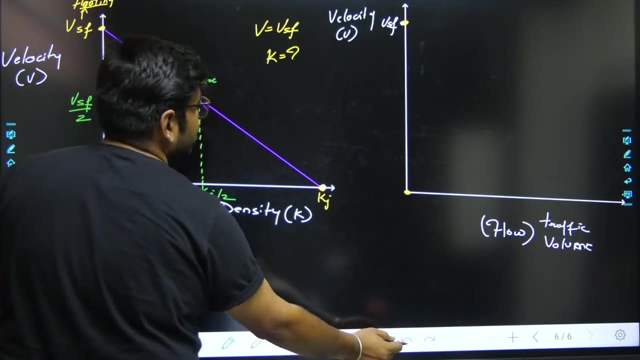 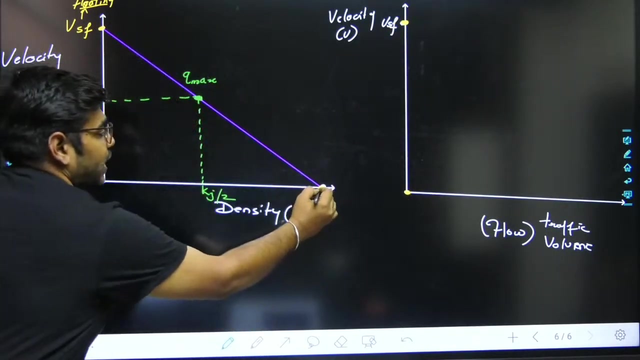 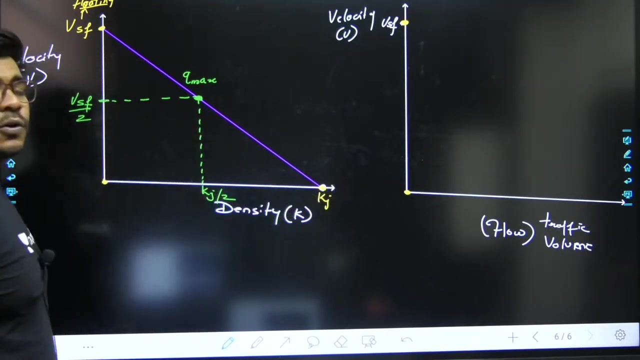 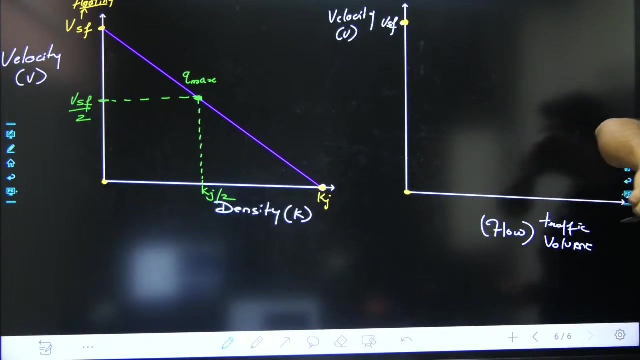 that at which point of time your velocity is equal to Vsf, at that time, what will be the value of K? Or I am saying that either we say this or leave this. I mean either. look like this: I said if V is equal to Vsf. sorry, I said if K is equal to 0, if K is equal to 0, then your velocity will be equal to Vsf. then your velocity will be equal to Vsf when your K is equal to 0. 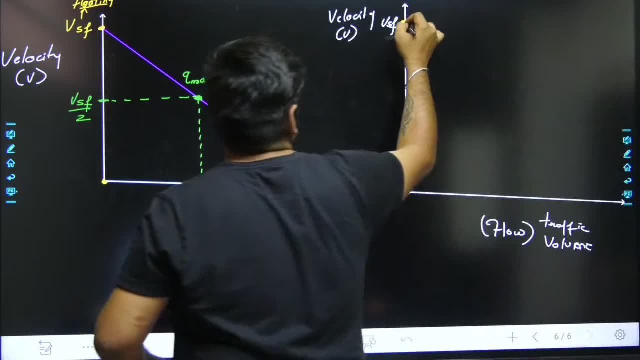 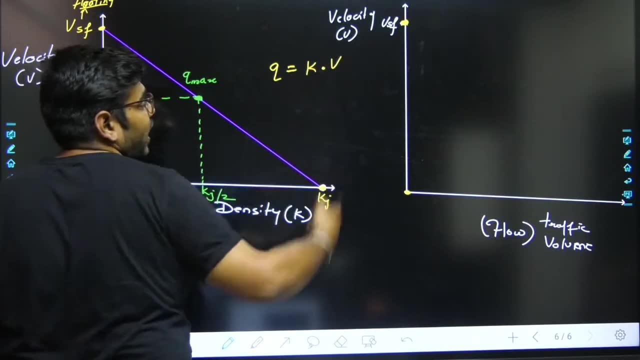 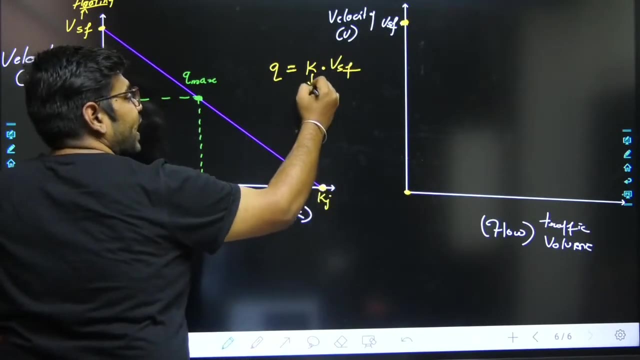 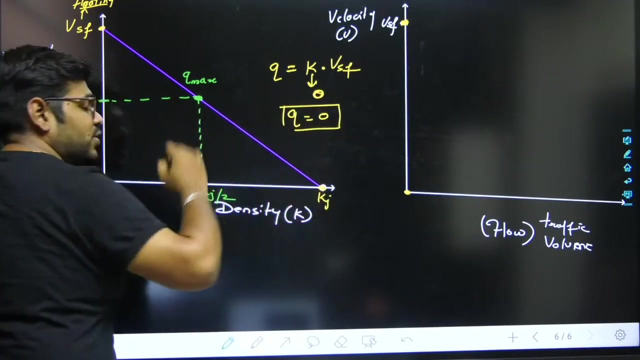 When your K is 0. And if your velocity is Vsf, When your K is equal to Vsf and your K is equal to 0, then you know what Q is equal to. Q is equal to K into V, Q is equal to K into V, and if V is equal to Vsf, then you know K will be equal to 0, and if K is equal to 0, it means Q is equal to 0, say yes or no. 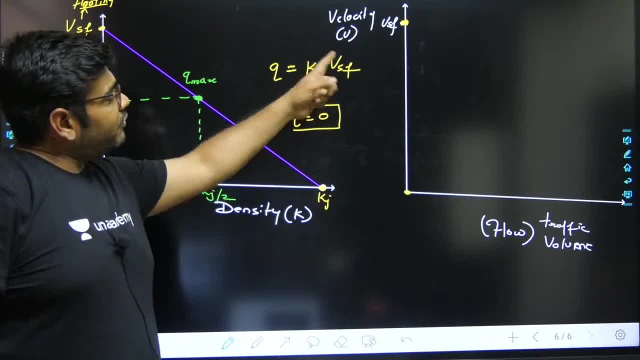 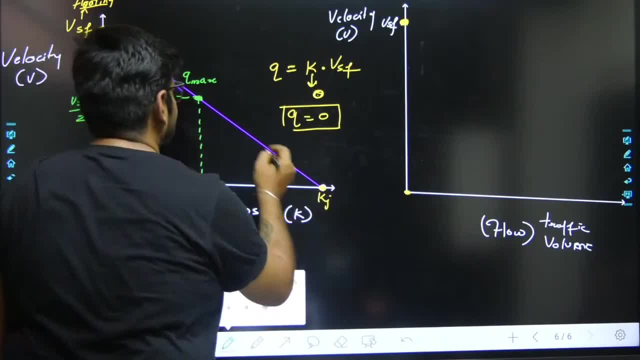 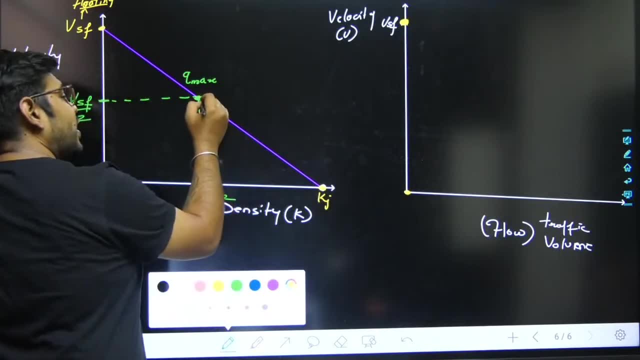 And if K is equal to Vsf, then K is equal to Vsf. And if you understood all these now I am connecting to this, See, see carefully. This line is representing QMax and this line is representing QD. 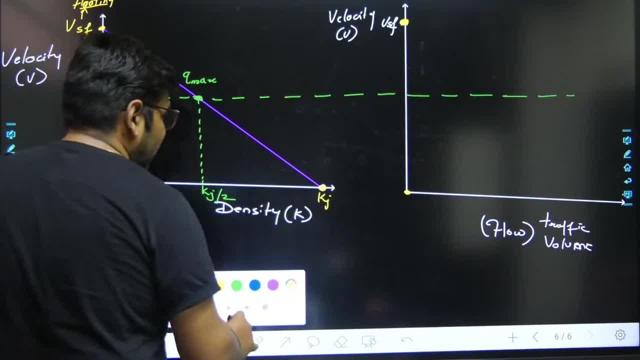 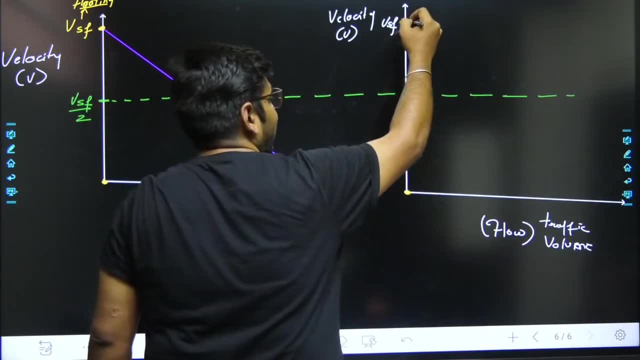 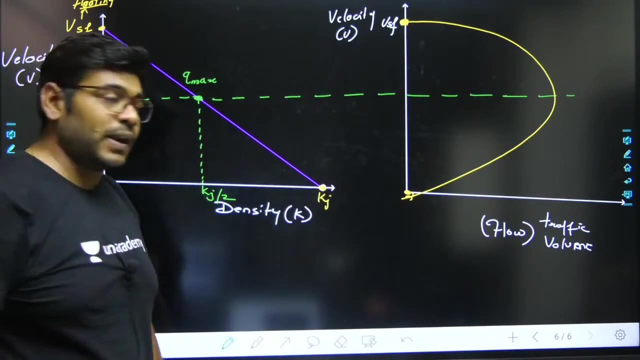 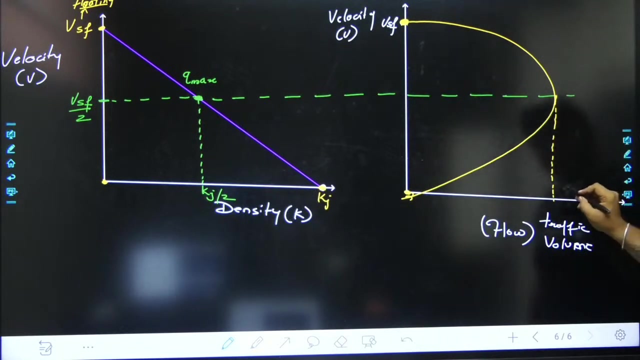 It is representing QMax. If you see here carefully, this means that starting and final points are zero after Q. So you will get to see this graph like this and at this point of time you will get the Q as Qmax. 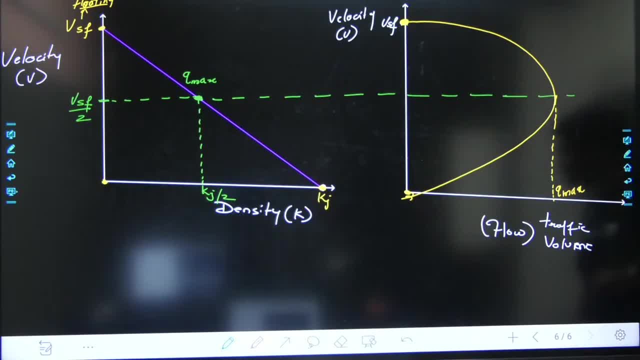 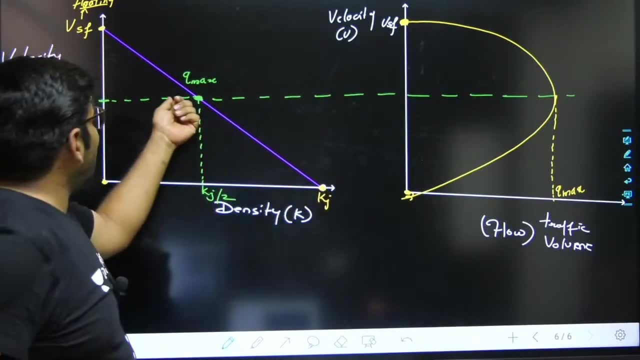 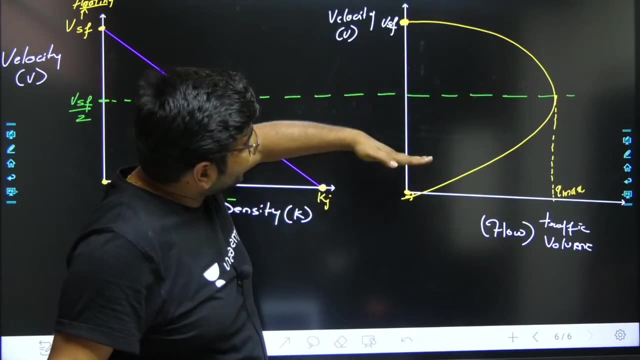 At this point of time, you will get the traffic volume as Qmax. Did everyone understand this At this point of time? I thought that this line represents Qmax, So your initial traffic volume is zero. Then, as you increase the velocity, your traffic volume will increase. 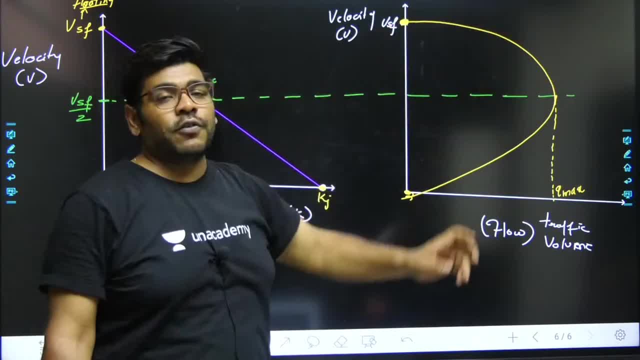 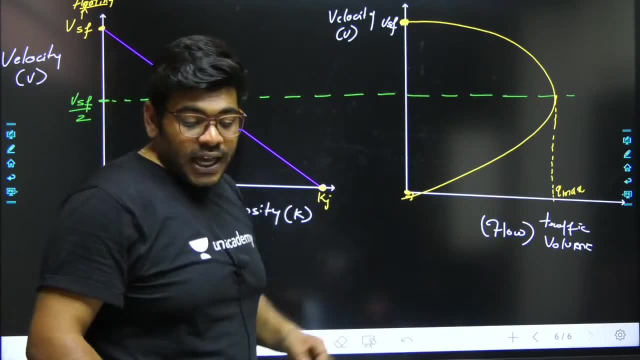 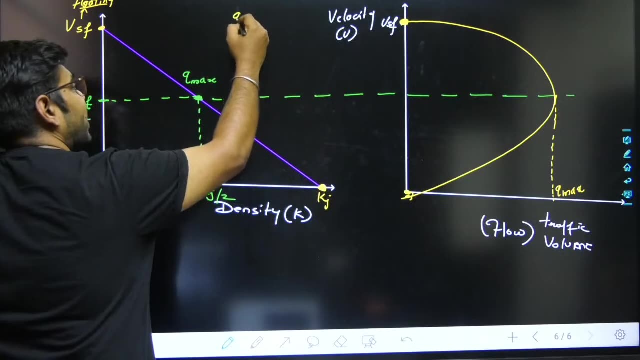 And if you increase the velocity more, then finally your traffic volume will be equal to zero in a particular section. I told you that at this point of time your K is equal to KJ. I told you that, if I am talking about this expression, Q is equal to K into V. 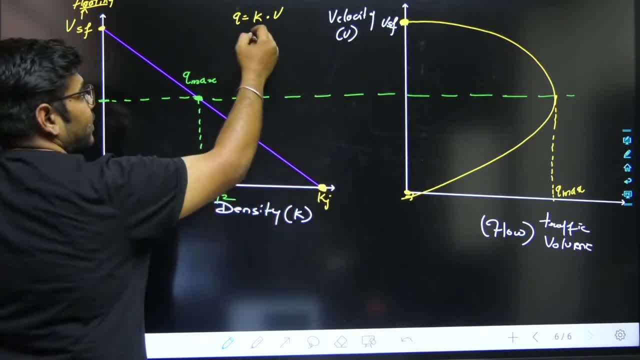 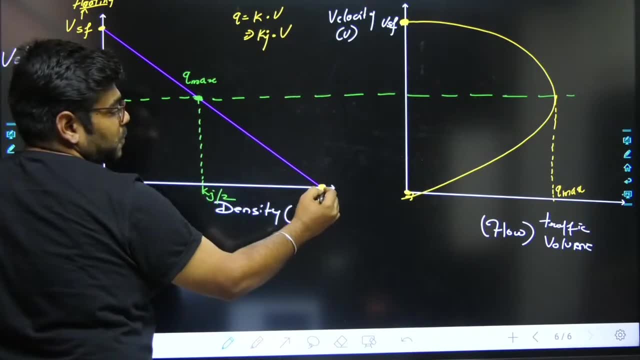 I mean, at this point of time K is equal to KJ. So if your K is equal to KJ, then your velocity will be equal to V. At this point of time we are talking about K and here we are talking about velocity. 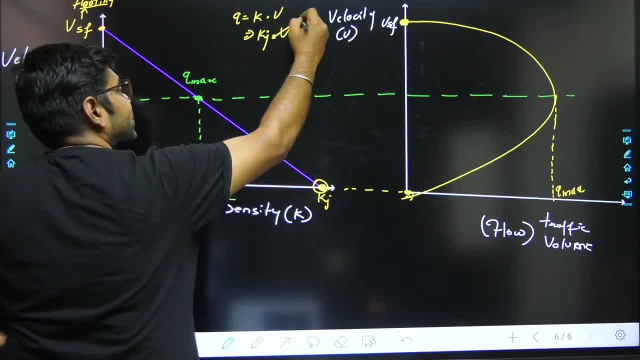 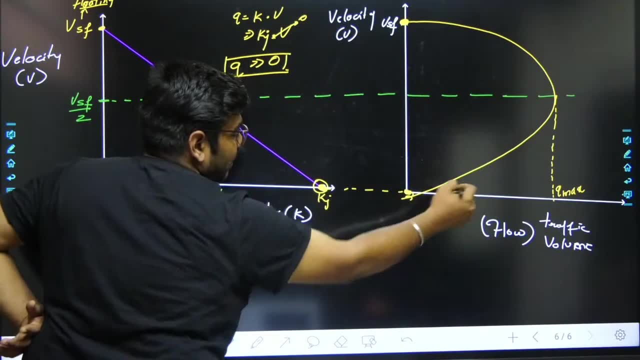 So if this maximum traffic density is there, then your velocity will be zero, And if the velocity is zero, then Q will be equal to zero. So if your velocity is zero, then your Q is equal to zero. Say yes or no. 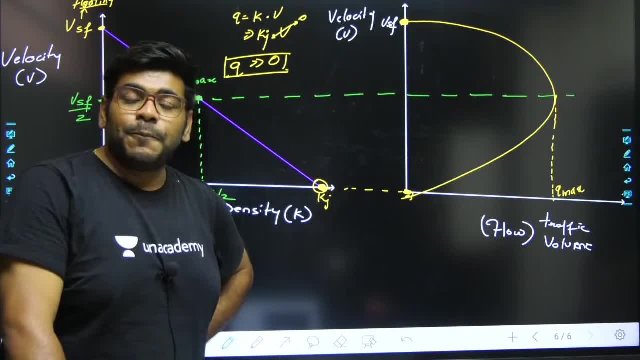 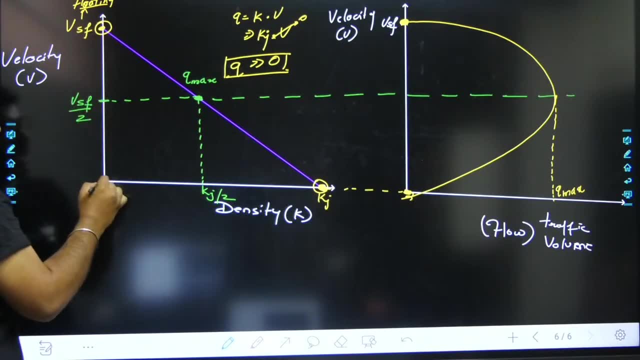 How is Q equal to zero on VSF? How is Q equal to zero on VSF? I have seen this graph. Do you understand this? That at VSF, the value of K is zero? And if you don't understand this, 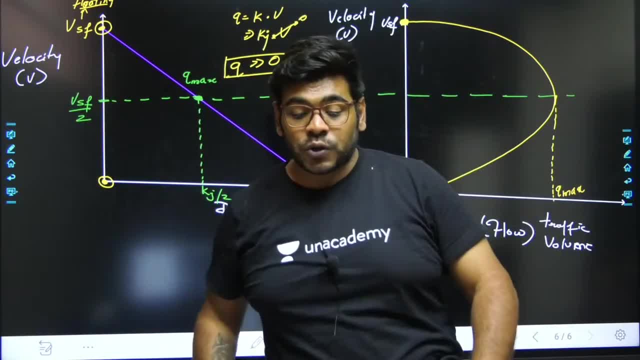 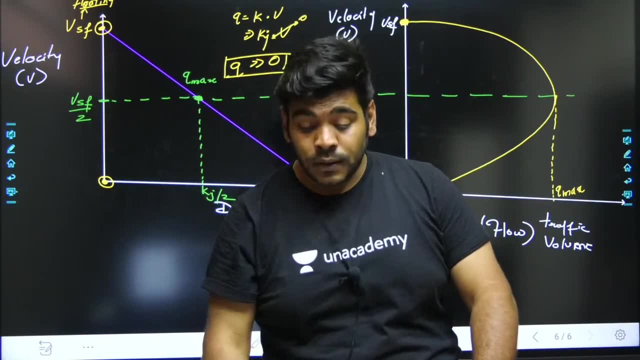 and if you don't understand this, then please understand this. please understand this what I am saying. please understand this. that what I am saying is. please listen to me carefully. why will a lot of people run away? because 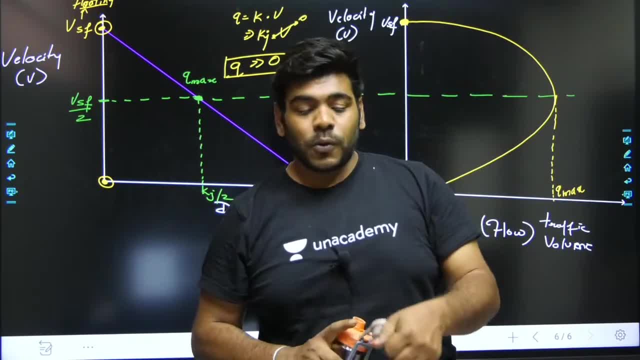 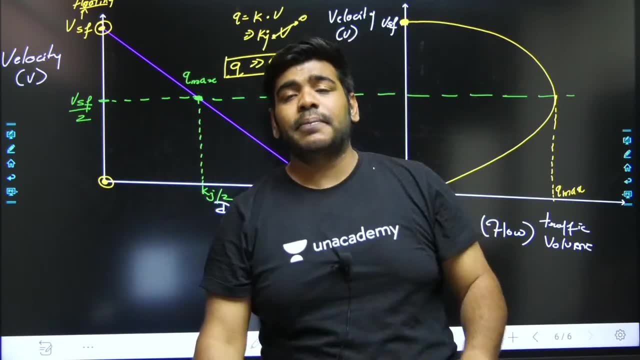 what I am saying is that we don't want to study anything tough. we don't want to study anything tough, so we won't even talk about easy today. we will not even talk about easy Today. we will talk about all tough. 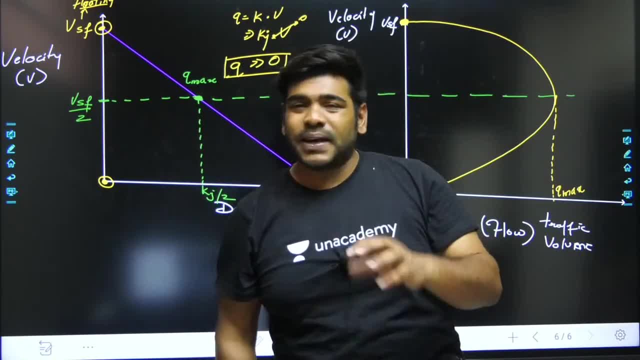 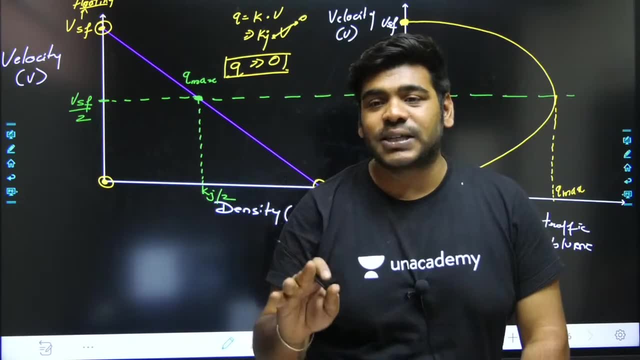 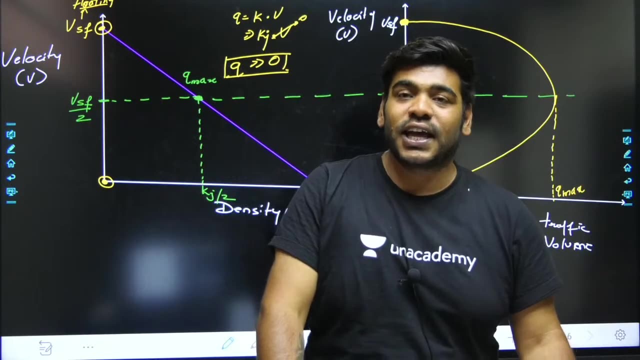 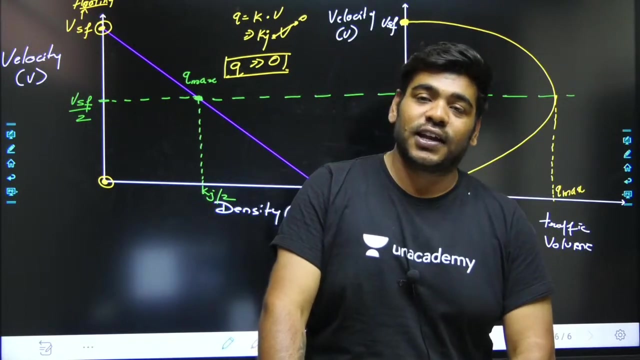 And I will take you to some another level. Okay, so people who study with me- always The rest of the people- will come. the time will come when they will ask you from where to read. where will you get the notes? do you understand? they will talk to you about all this, that where will you get the notes? where is the number of this video wrong? but they don't know that you have read everything first and we will not tell anyone at that time which number is wrong and which is wrong. come on, let's start the talk. 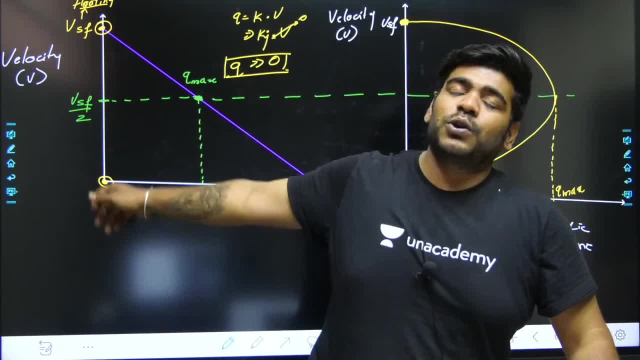 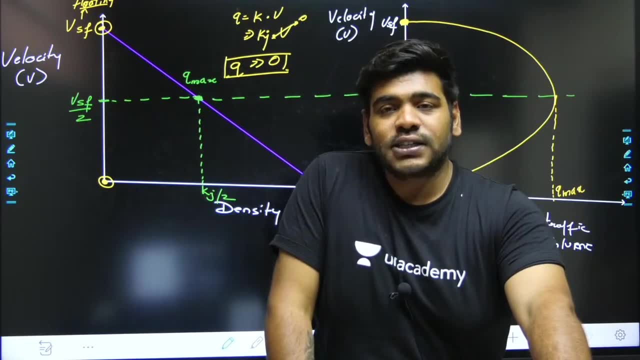 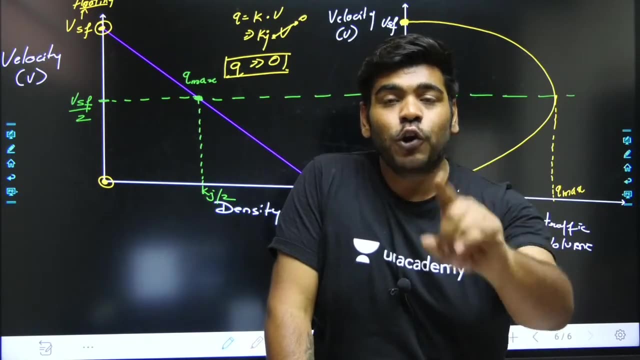 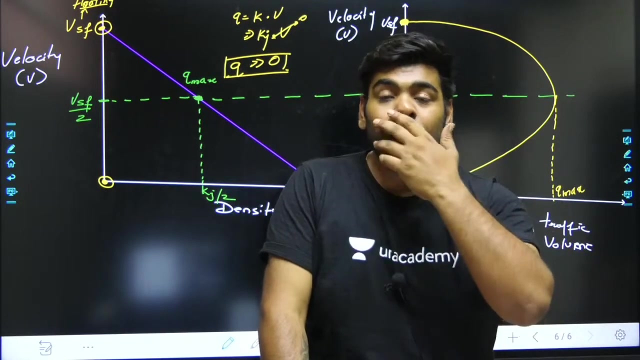 So I said: look, if you don't understand that K is equal to 0 and V is equal to VSF, then remember that day. that means it is yesterday. so remember that day when I was telling you this, when I was telling you this, when I was telling you this, remember that day when I was telling you this: that VSF means floating velocity, and floating velocity means when your vehicle is moving in a particular section with zero hindrance. 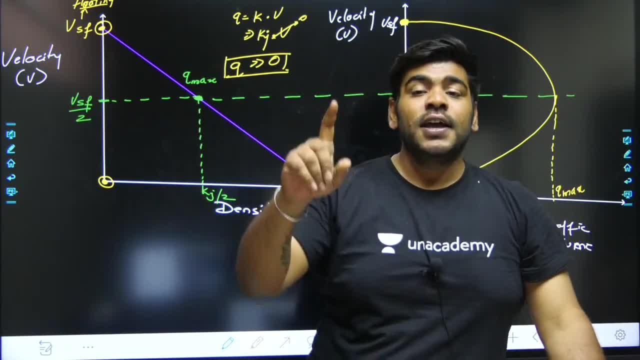 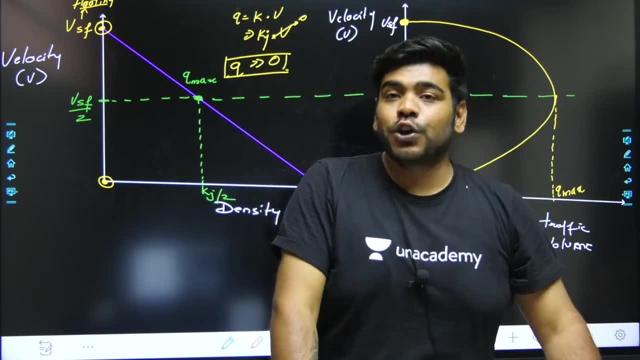 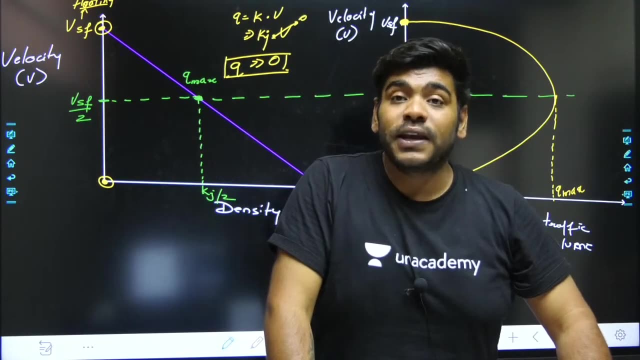 Say yes, I said this definition yesterday. So I said: look, I said this definition yesterday, what I said about floating velocity, that when your vehicle is moving with zero hindrance it is called as floating velocity. Say yes, and zero hindrance means traffic density is equal to 0, meaning in that particular section there is no one to stop your car. there is no one. 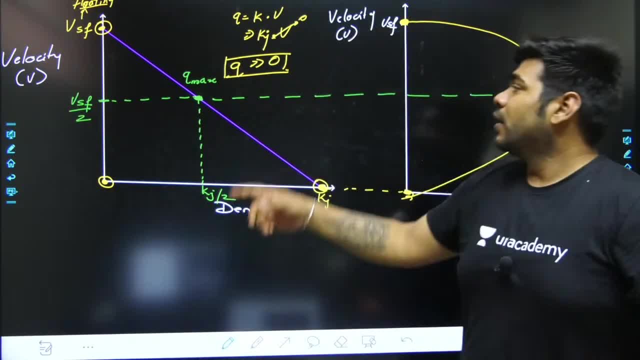 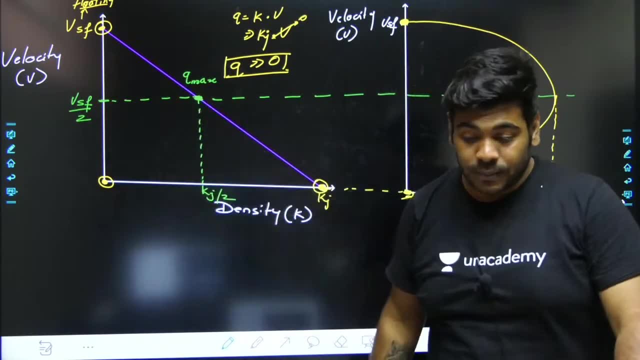 So I said zero hindrance means traffic density is equal to 0,. so when your V is converting into sorry, when your VSF sorry, when your K is equal to 0, your V is equal to VSF and K0 means Q0. 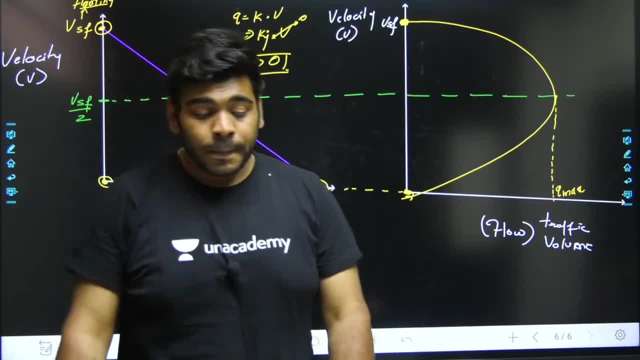 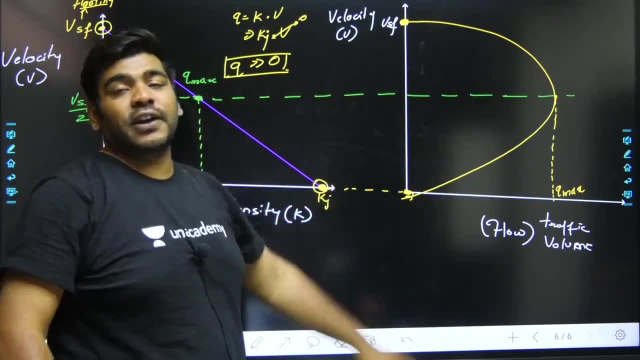 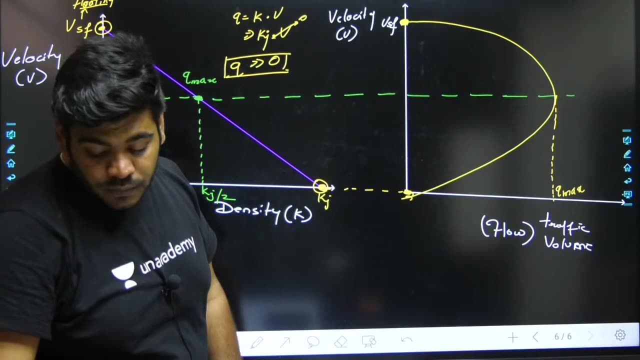 K0 means K0.. If this is understood, then I think you understand this graph. okay, if you understand this, then everyone will understand this graph. and if this graph is understood and if this graph is understood, everyone understands. everyone understands very good if it shines. 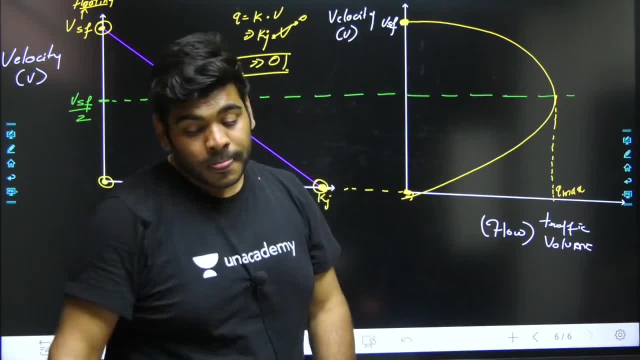 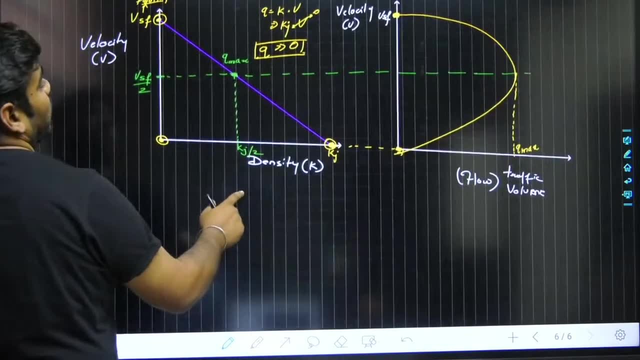 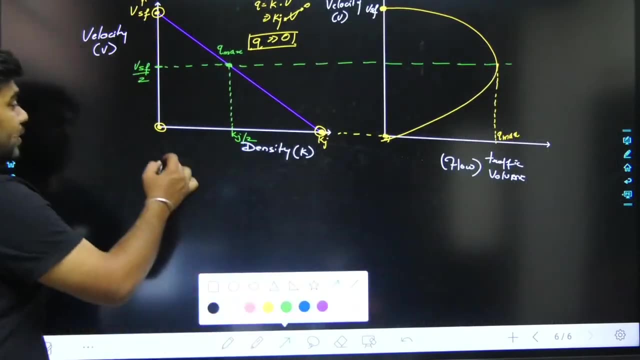 And if this graph is understood- everyone has understood, everyone has understood very good- If it shines, then the next thing will shine here. I mean come, I mean, come, look here. now we want to make one more graph from this graph. 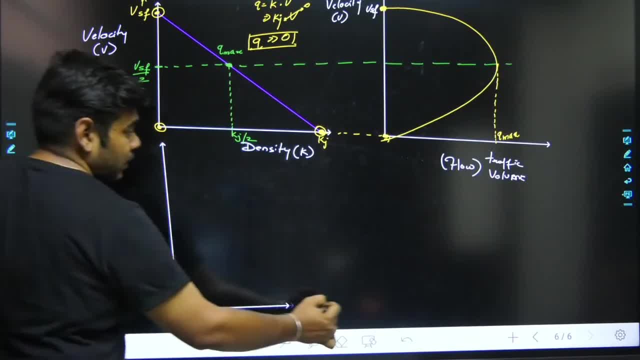 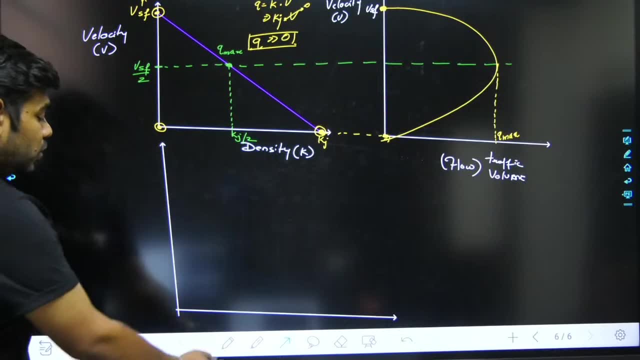 I mean now we want to make one more graph from this graph. here is the next graph. I mean we want to make the next graph from this graph And we said to this graph: who will it be between? I mean, who will it be between? 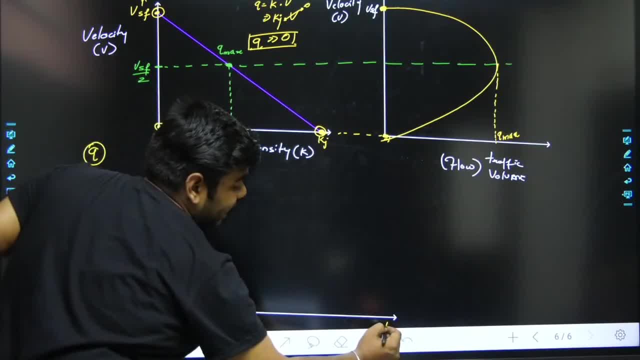 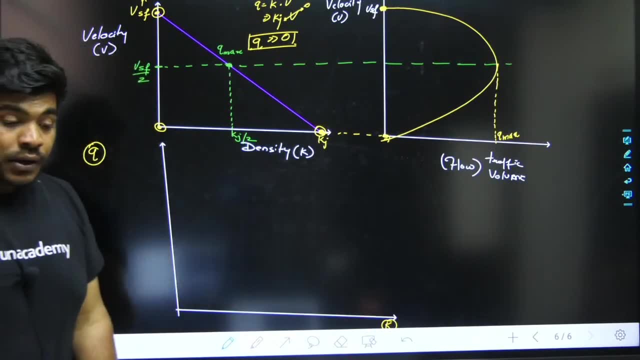 So I said this will be between traffic volume Q and traffic density K. What did I tell you? We are making this graph between traffic volume Q and traffic density K. We are making this graph between traffic volume Q and traffic density K. So I said: look here, look here, I said, when K is equal to 0,. 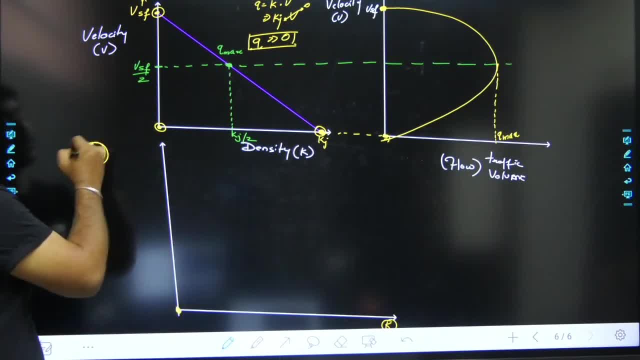 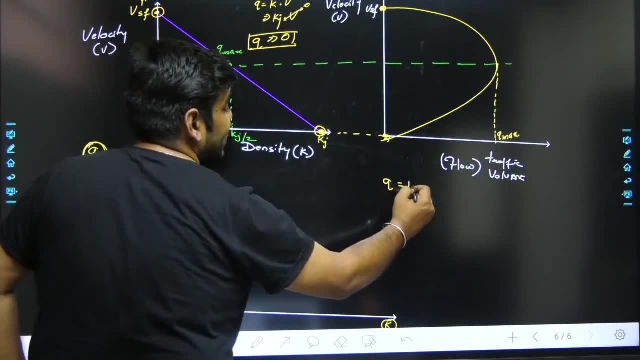 when K is equal to 0,, then what will be the value of Q? When K is equal to 0,, then what will be the value of Q? So you said, look here, Q is equal to Sir, equal to K into V. 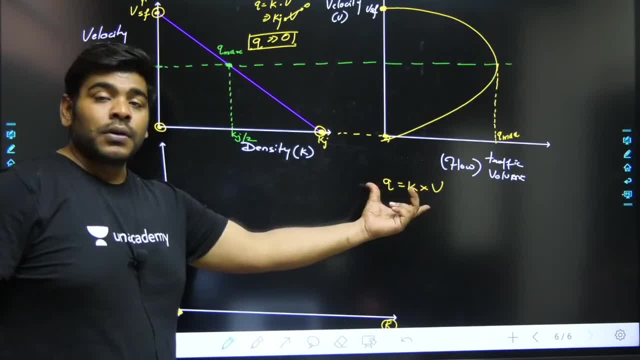 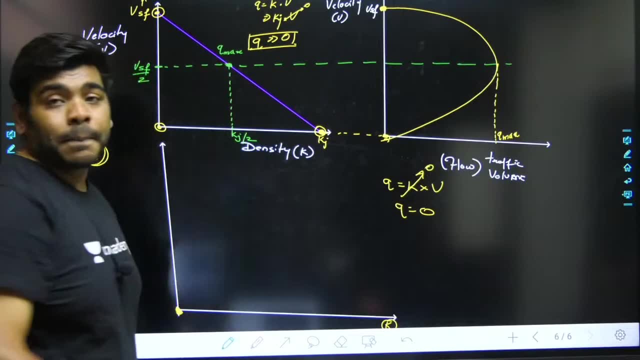 Q is equal to Sir, equal to K into V. So, Sir, when K is equal to 0,, when Sir K is equal to 0, then, Sir, the value of Q will also be 0.. Say yes or no. 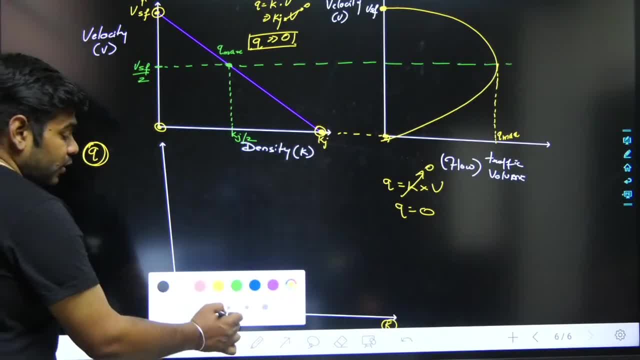 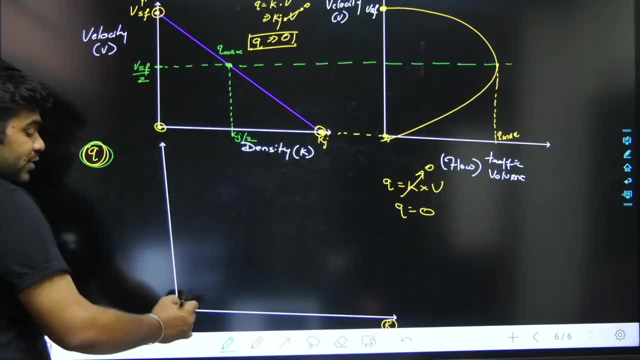 Say yes or no. So I understood that the value of Q will be 0.. The value of Q will be 0.. Very good, This is Q. Its value is 0.. K is equal to 0, then the value of Q is 0. 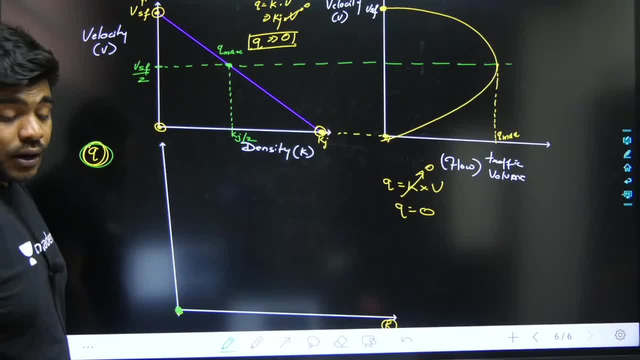 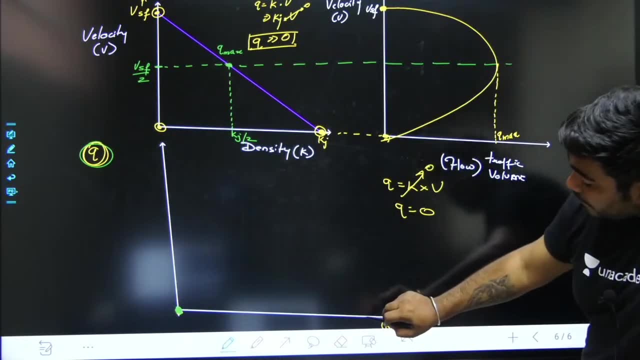 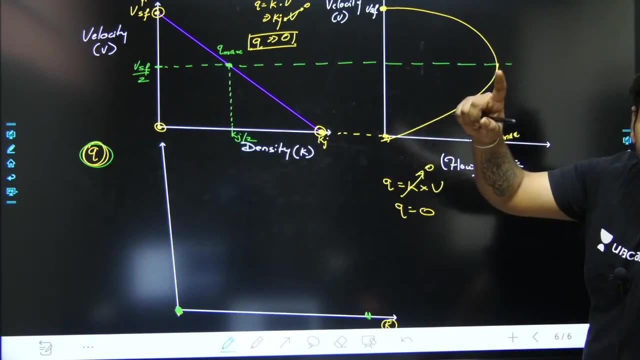 Very good, I talked next to you. Next, I talked to you When K is equal to KJ. when K is equal to KJ, then what will be the value of Q? Next, I talked to you When K is equal to KJ. 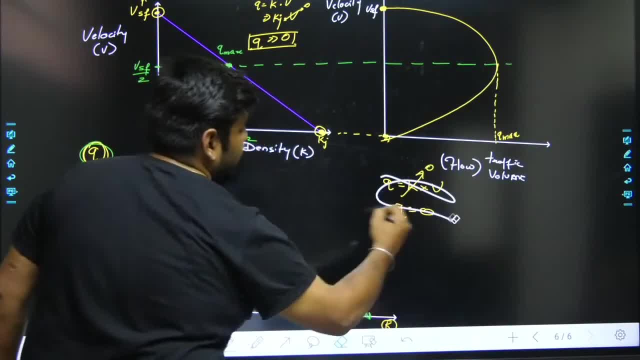 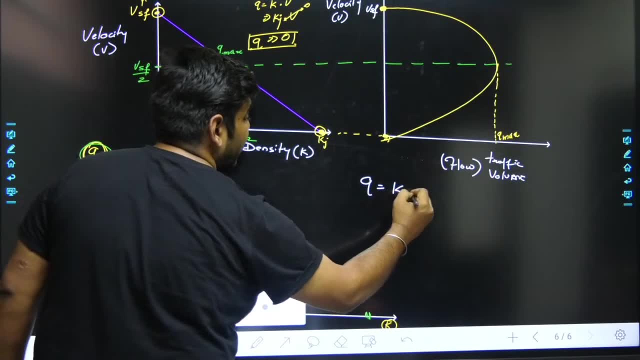 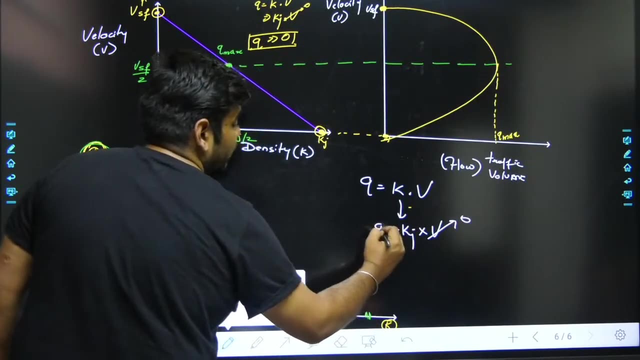 you said: all right, Sir. I said next I talked to you- when K is equal to KJ. When k is equal to kj, then you know, velocity tends to 0, it means q is equal to 0, say yes or no. 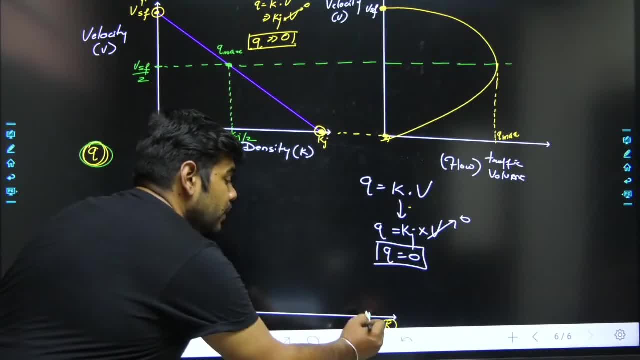 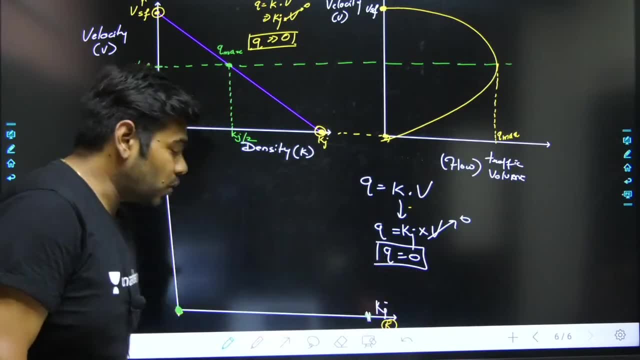 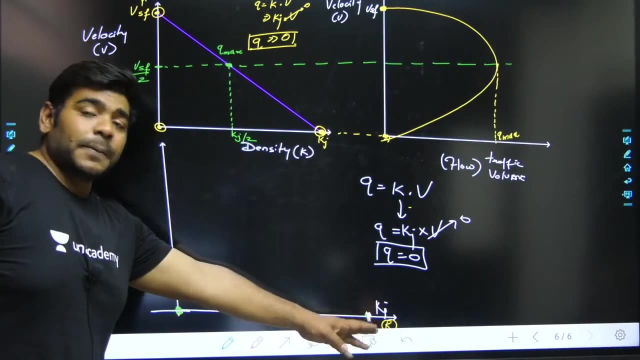 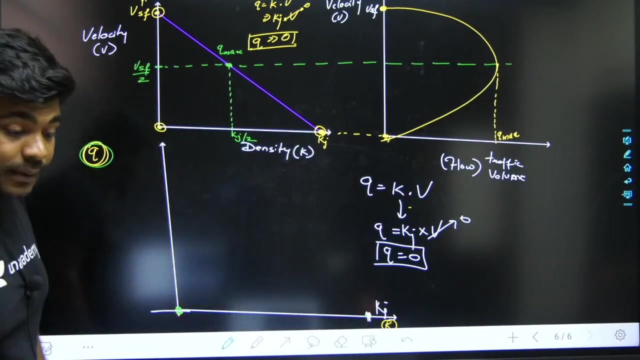 When k is equal to kj, then also the value of q is 0, say yes or no. Then the value of q is 0, so we understood that according to this line, the value of q is 0.. Whenever the value of q is 0, when k is 0, then also q is 0. and when k is equal to kj, then also q is equal to 0. 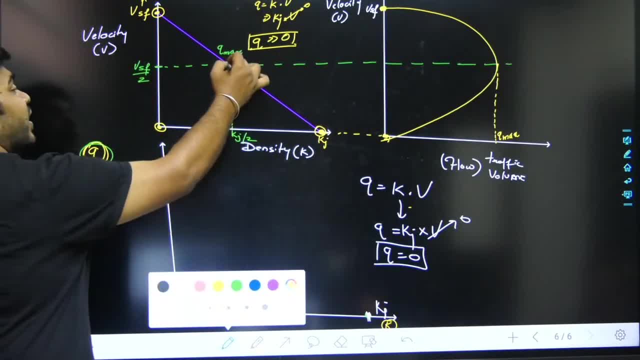 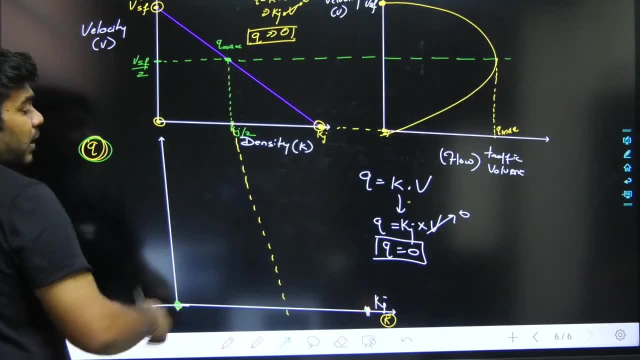 And even then, if q is equal to 0, then we bring this line of qmax down. Means, if we bring this line of qmax down. So I said, look here carefully. what I want to say Means, look at this line carefully. this is the line of qmax. 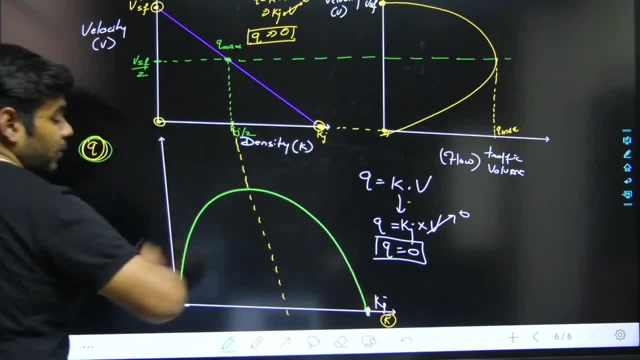 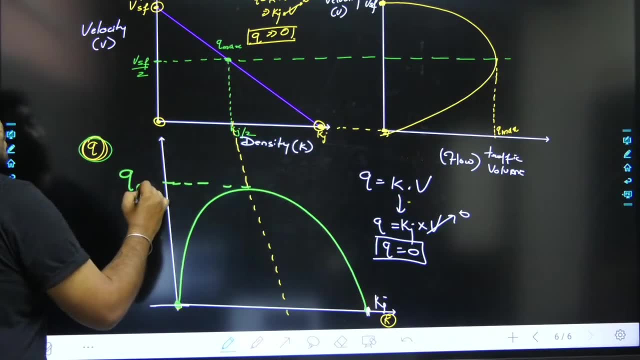 Means the graph you are getting to see now. you are getting to see this graph, Now the graph you have got to see. you have got to see this graph And this value, we call it qmax. We call it qmax, Did you understand? 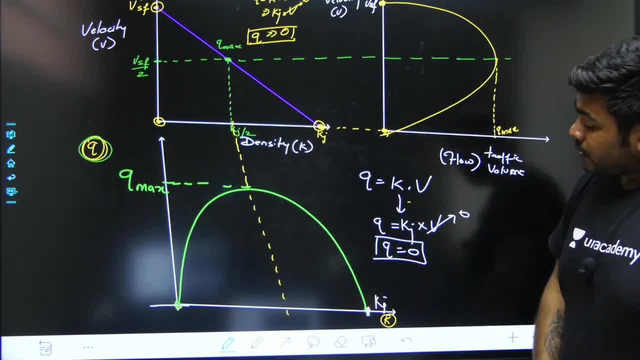 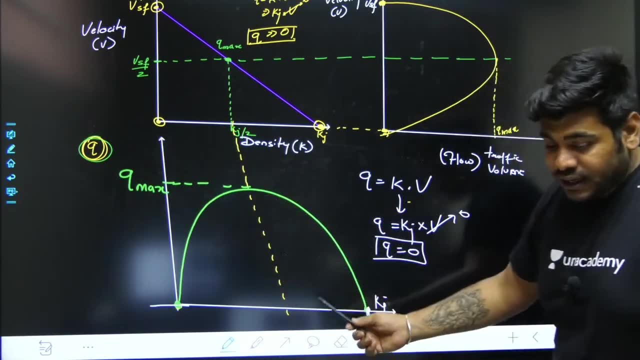 Look carefully and tell me: did you understand this graph also? So when k is equal to 0, then also the value of q is 0.. And when k is equal to 0,, then also the value of q is 0. So when k is equal to kj, then also q is equal to 0.. 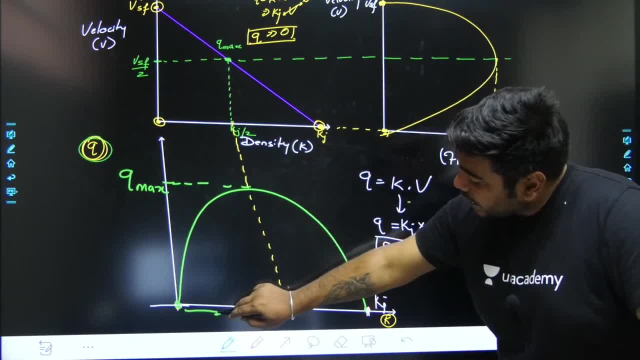 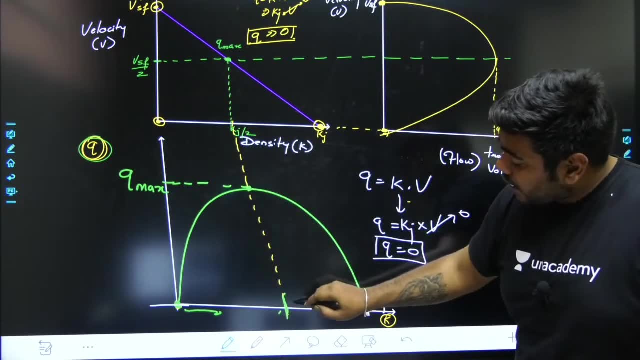 So slowly, slowly, as your traffic density increases, your traffic volume will increase And when your traffic volume will be maximum, then at that time this k is equal to kj by 2 point will be there. This point will be how much You will get to see maximum traffic volume at this point on kj by 2.. 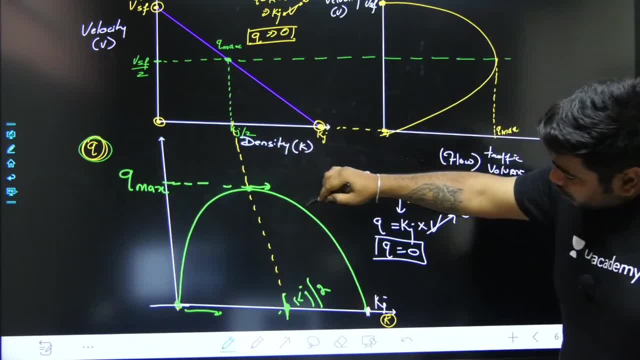 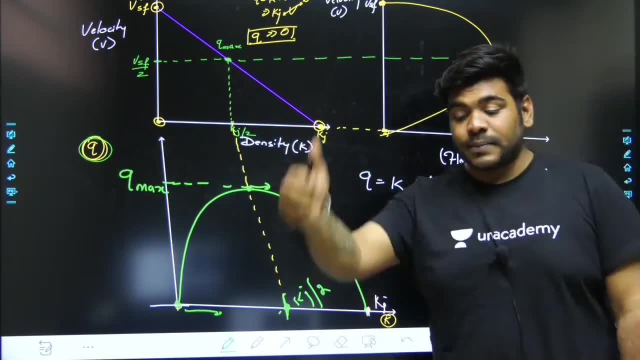 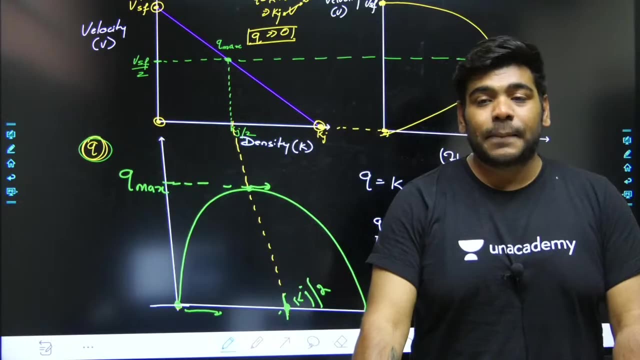 And then even after that, if you will increase the traffic volume, then also your traffic volume will decrease slowly, slowly. Do you understand this thing? Tell everyone quickly. Do you understand this thing? Is there anything that we will not be able to tell? 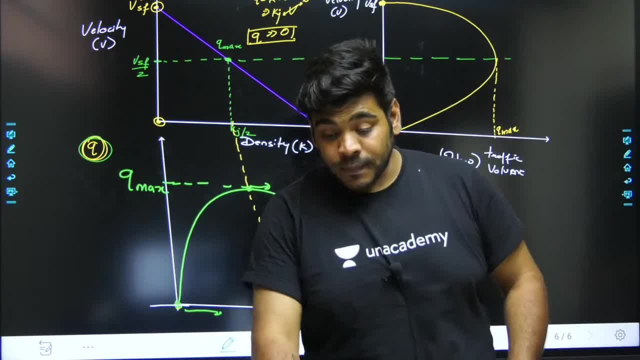 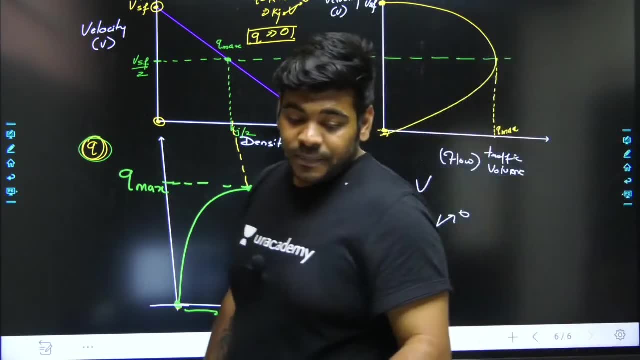 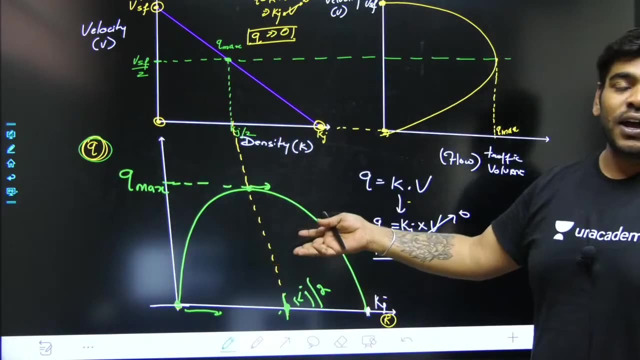 I mean, there is nothing that we will not be able to tell. k is equal to kj by 2.. What should I tell my son? Splendid, Very good. Is there something amazing? I had said that it will be difficult, But we will understand it. 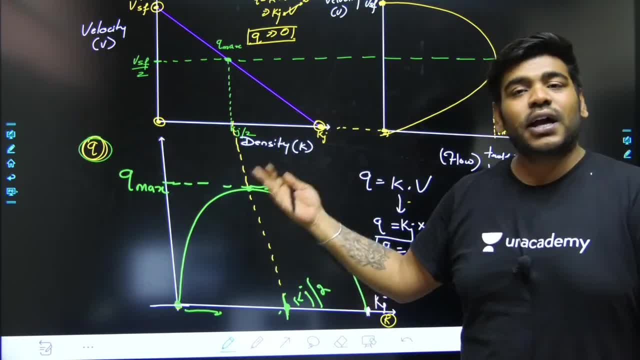 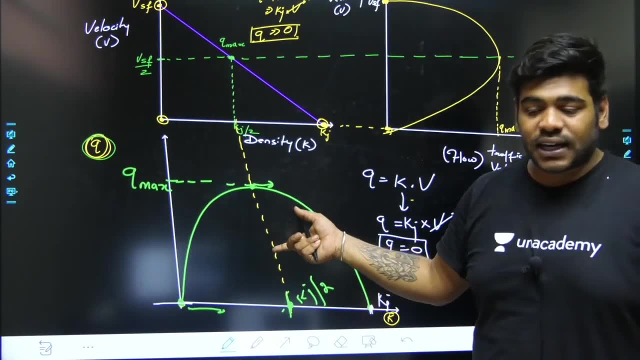 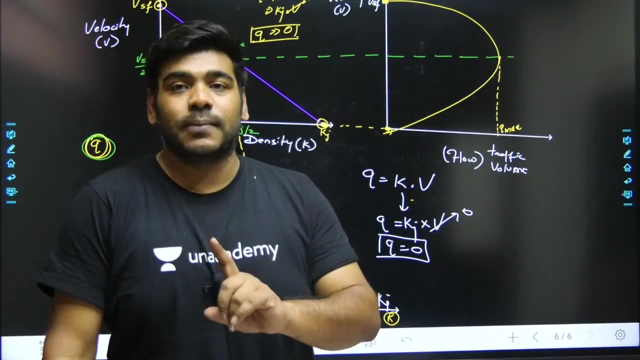 We are studying it. When no one will understand, then we will not understand. Then there is a discussion: How will this be saved from us? And when we will be sitting and talking in an interview, then only we will be talking, When we will be talking technically. 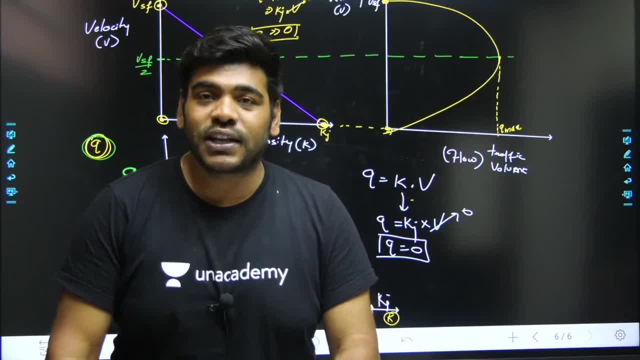 Everyone will be sitting and listening. What is he talking about? He is making q equal to zero. Sometimes he is making k equal to zero. Sometimes he is making kj equal to zero. From where is he putting zero And what is he talking about? 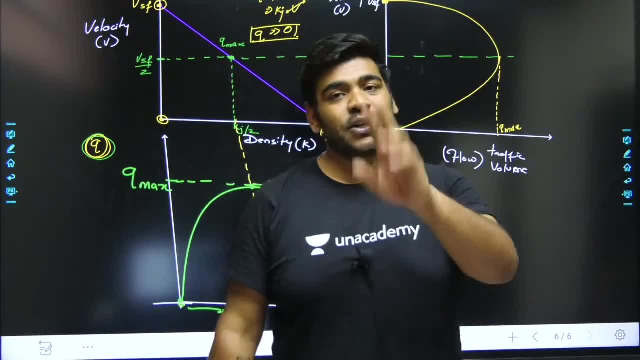 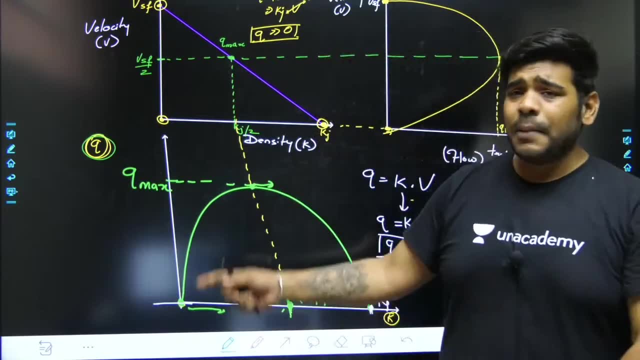 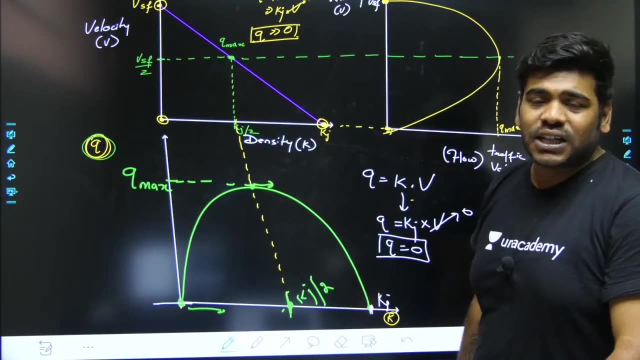 I don't understand And don't let him understand The one who should understand. he has understood. Ok, Son, for this linear and parabolic. we will draw an equation of a graph later. It is not important for us. That is why I have not played anything with the equations of the graph. 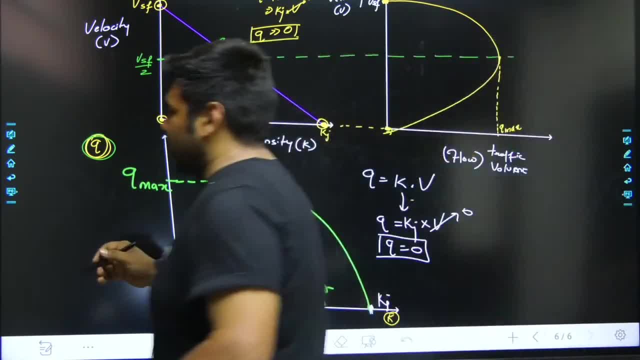 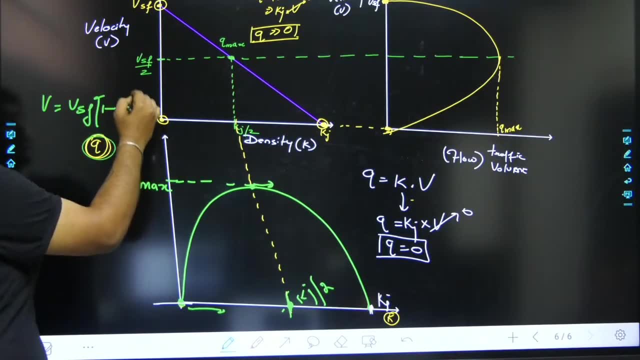 Ok, I said that when you saw this, when you see this equation, you convert it. v is equal to vsf1 minus k by kj. You convert it by doing this. So this equation, In addition to this, the equations of q and k are made. 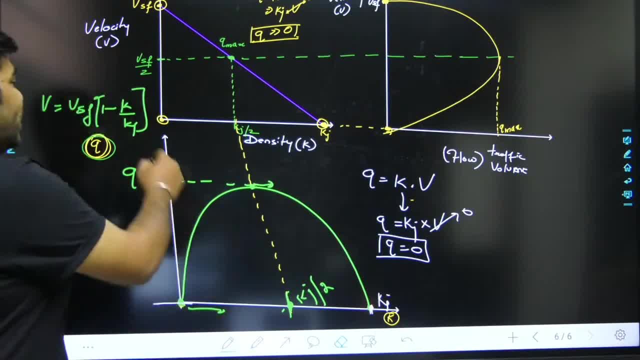 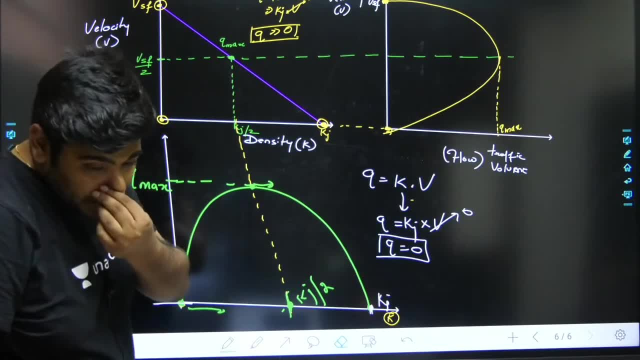 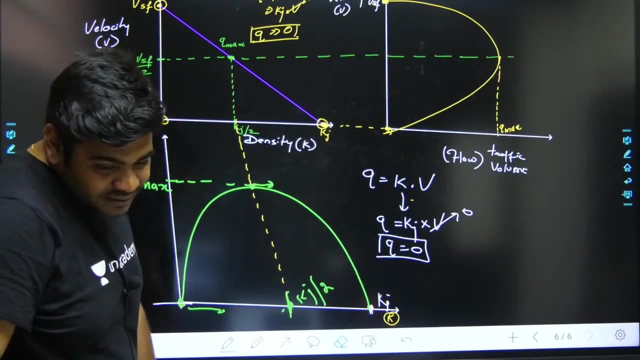 The equation that is made in the graph is a parabolic equation, Which I have not told you by deriving it completely. Ok, We have talked about as much as it was important for us according to the gate. Ok, Love from Maharashtra, Ok. 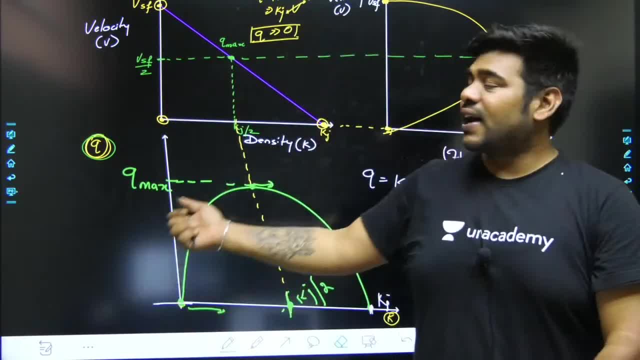 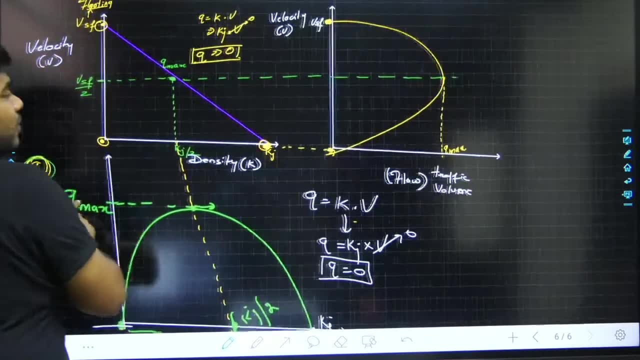 This graph is valid in the green shield model. Yes, I have made this graph only for the green shield model. For whom is this graph? I have made this graph only according to the green shield model. Beyond that, son, everything is about the PhD. 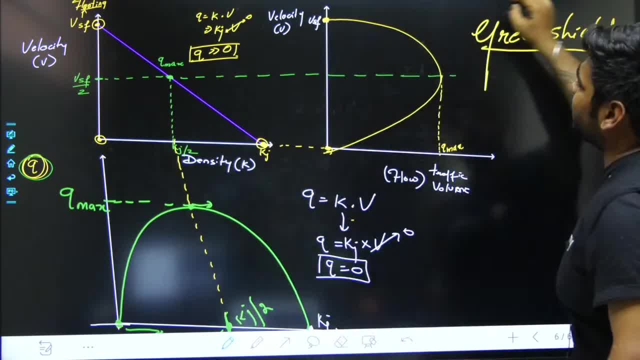 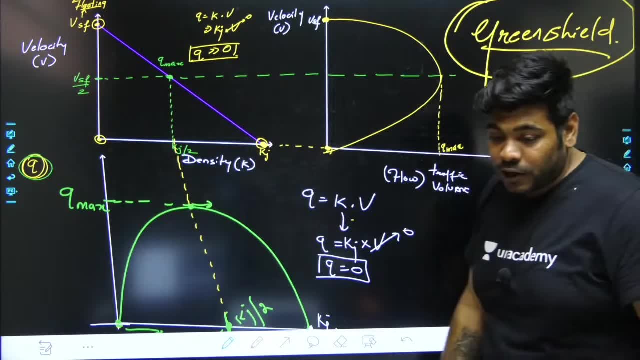 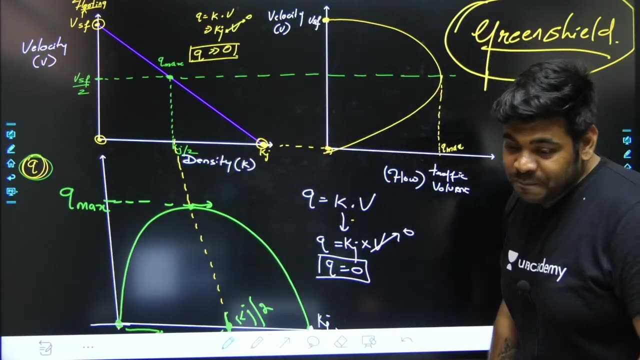 Beyond that, everything is about the PhD, So this graph is valid. I have told the relation of all three. This is only for the green shield model. Ok, This is only for the green shield model. Ok, Come on, let's talk. 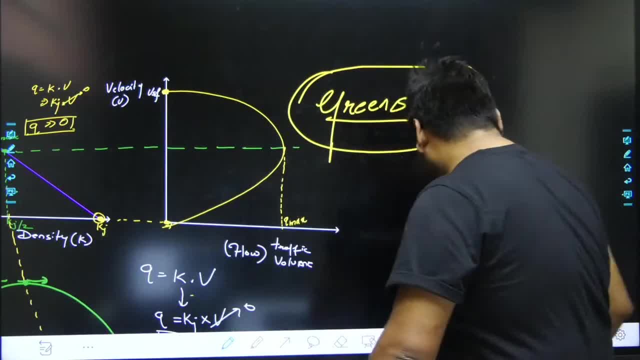 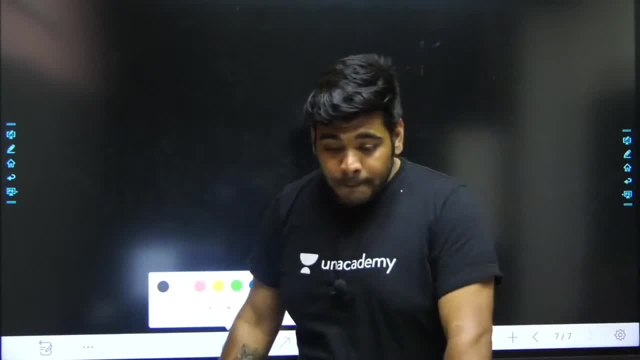 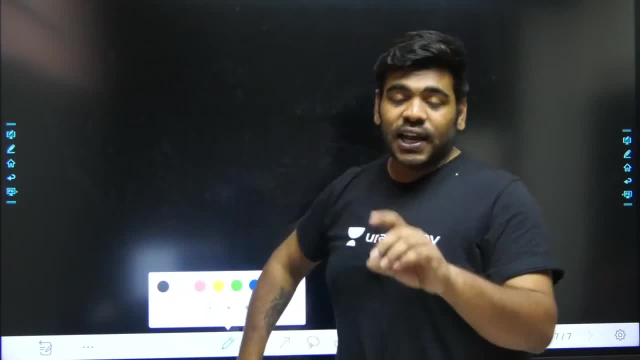 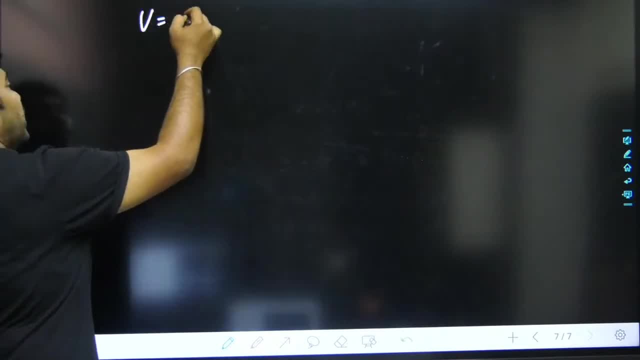 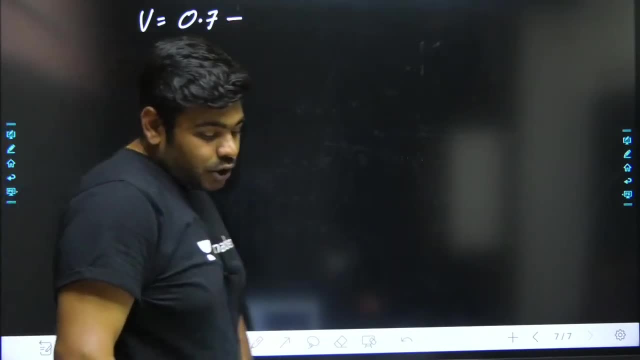 Come on, let's talk. Come on, let's talk. The questionfi has been given you several times. OK, Avg gives you a relation. v is equal to. This question has been asked many times: 0.7k. 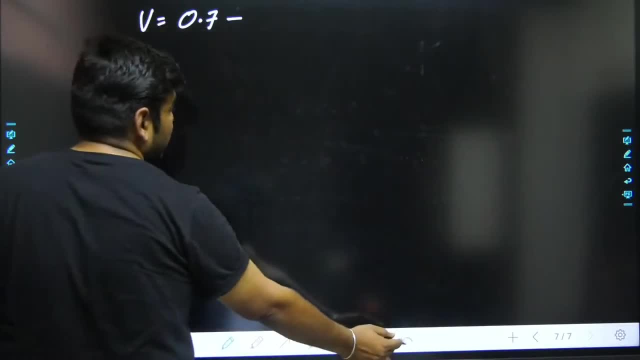 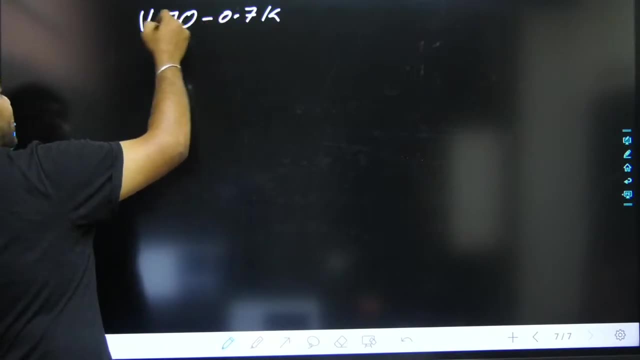 v is equal to 0.7 minus sorry. v is equal to 70 minus 0.7k. v is equal to 70 minus 0.7k. It has been given you. I have given a relation to you. 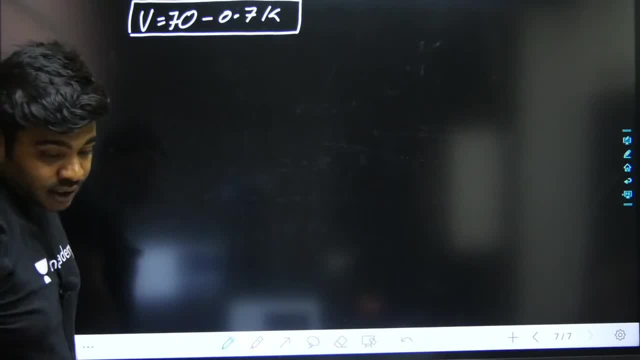 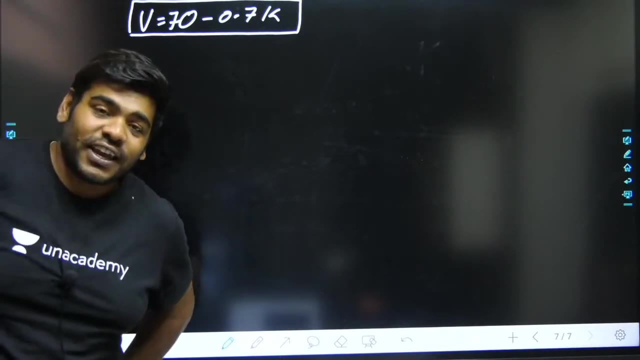 one is given to you. I have given the relation of velocity to you. OK, Today we keep the practice session, no, so I have given a relation. come, let's talk. I have given a relation. v is equal to 70 minus 0.7k. Ranjit, you stay here and understand. 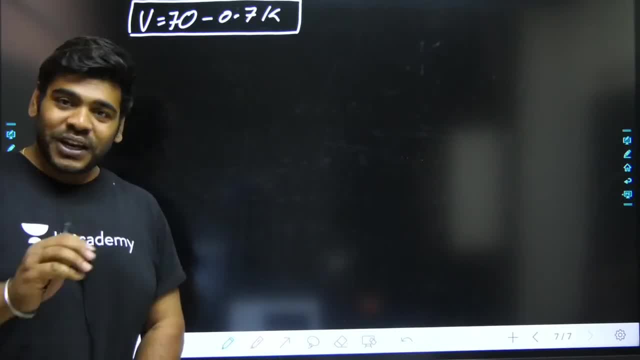 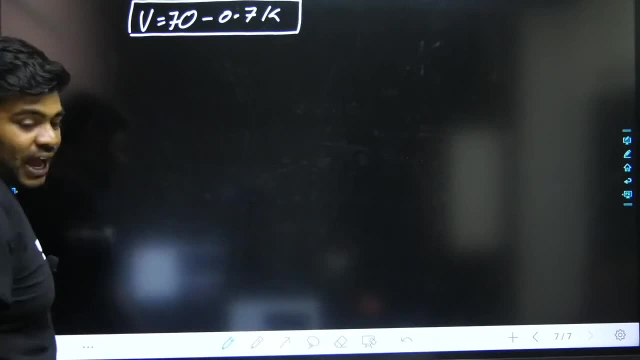 what you have missed. you have given money and you have become so you stop and understand this. so I have told that. look here you were asking this Amman co yesterday. for that reason I am saying that, I am saying that this expression has come in the same gate. 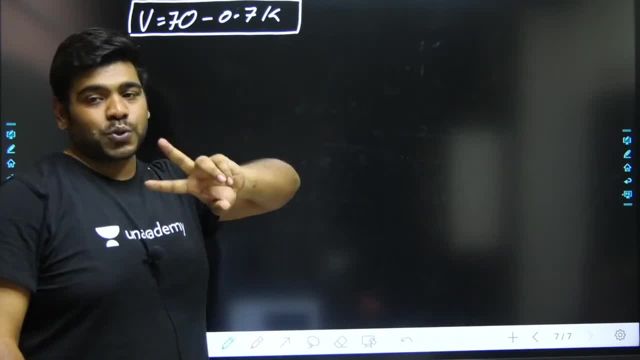 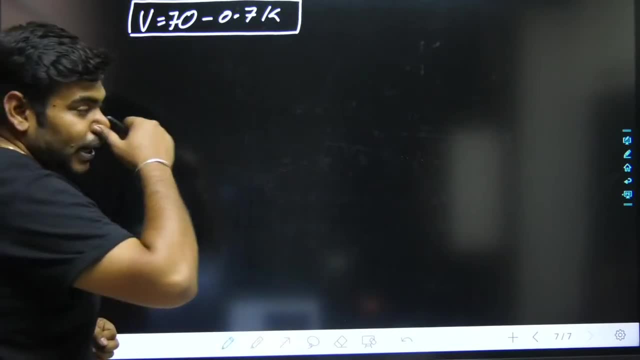 earlier too. this expression has come in the same gate earlier too, and comes twice, not once, but twice. Ok, that is why we have started talking through this expression. so we have started speaking from this expression. so I have told you that, if you are, if you have ever targeting engineering, 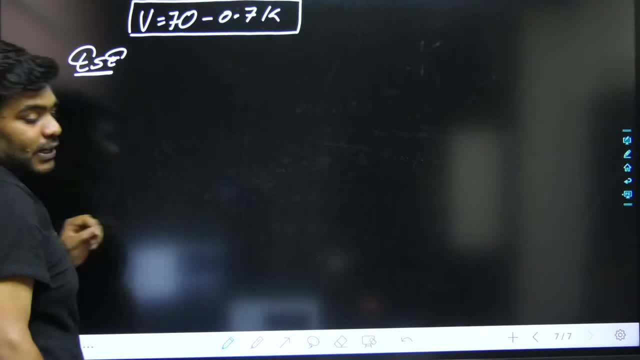 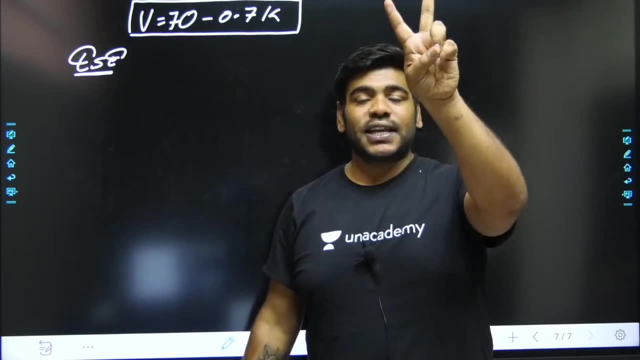 services. if your target is engineering services. if your target is engineering services, then it is important to return at the time when everything is done. that said you gingerly. So I will suggest you how to approach this question. I will tell you two different ways. 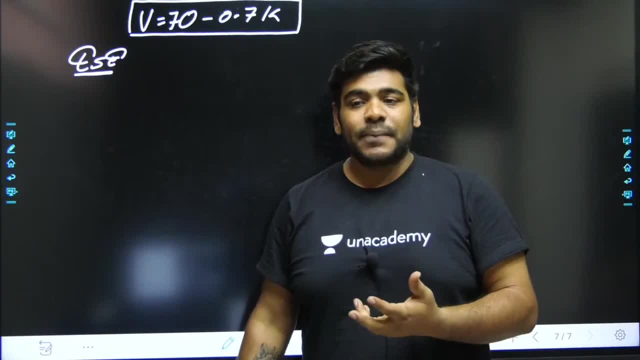 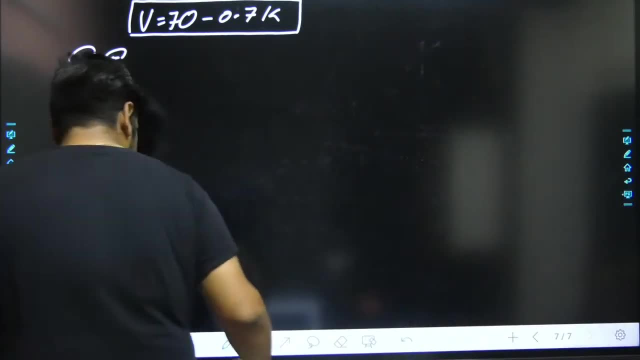 Whenever you are writing the mains of any SSC, JEE or engineering services, then how do you have to approach, And when you are approaching for GATE, then how do you have to approach? I am telling you that. So I said first of all, let's talk about engineering services. 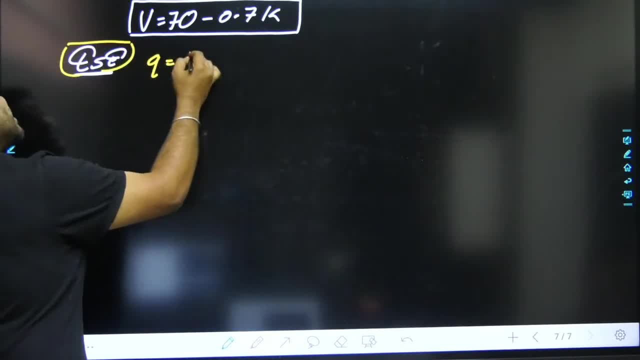 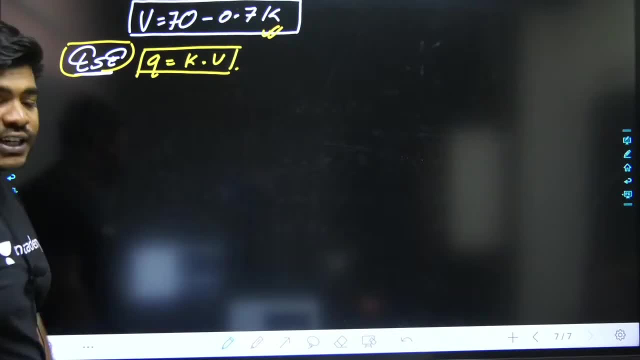 How do you have to do engineering services? So you know, Q is equal to what, It is equal to K into V and I have given you the expression here. As soon as I saw this expression, I understood that I have been given the expression of linear velocity variation. 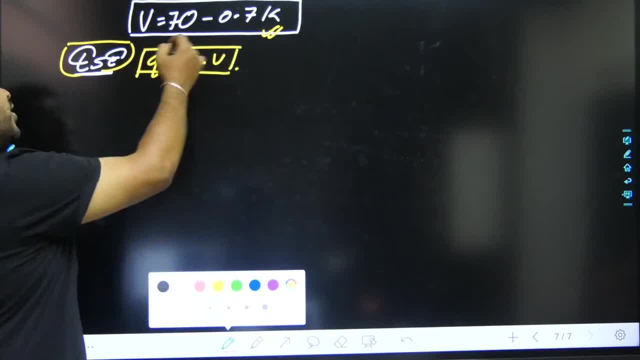 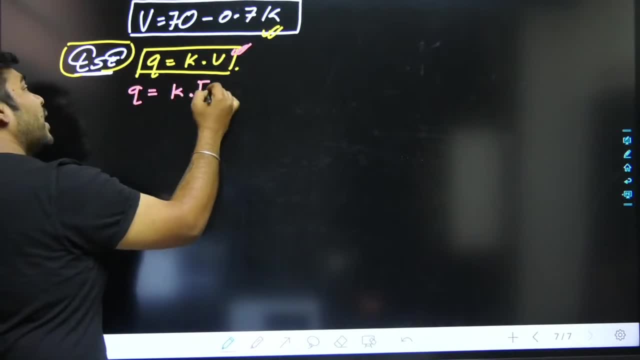 Okay, if I understood this, then I know that Q is equal to what. It is equal to K into V. So I said that Q is equal to K multiplied by 70 minus 0.7K. It is equal to 70 minus 0.7K. 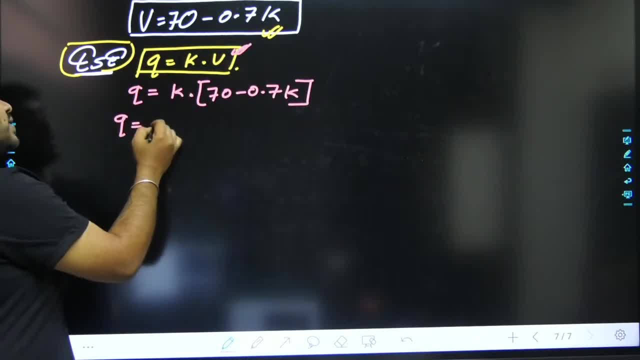 Very good. And if I understood this, then I said that Q is equal to 70K minus 0.7K. It is equal to 70 minus 0.7K squared. Yes, it will be like this. Now you know that this expression, this Q expression, has come in front of you. 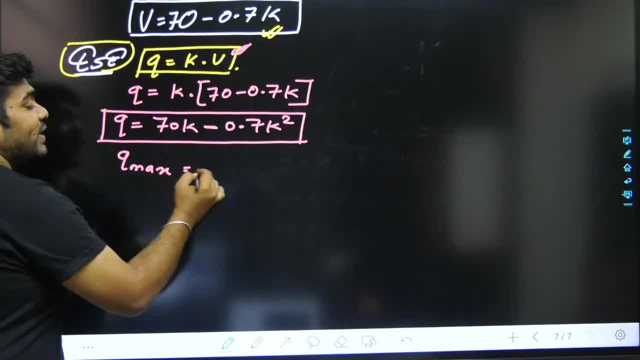 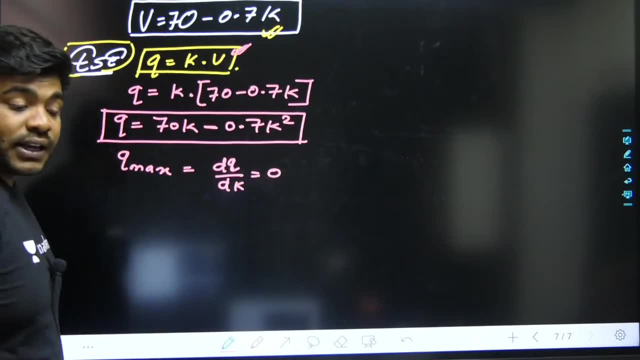 What do you have to find out? You have to find out the value of Qmax. And to find out Qmax, what will we do? DQ by DK is equal to what. It is equal to 0.. I mean, DQ by DK is equal to what? 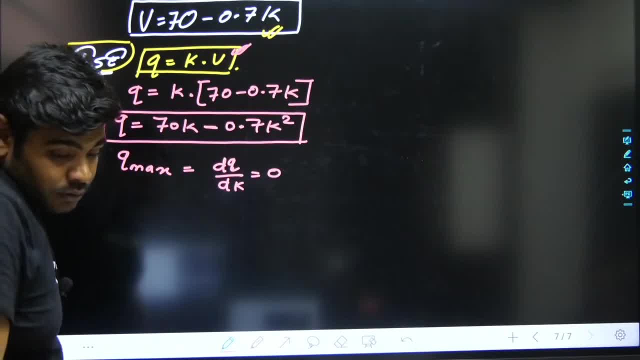 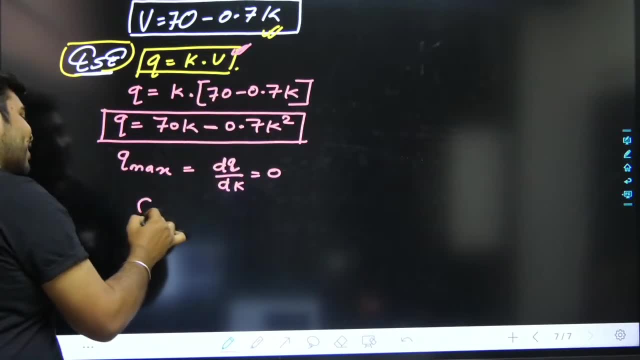 It is equal to 0. So if you, okay, let's talk about DQ by DK. So I mean DQ by DK is equal to 0. So 0 is equal to 70K. If you do 70,, then what is the value? 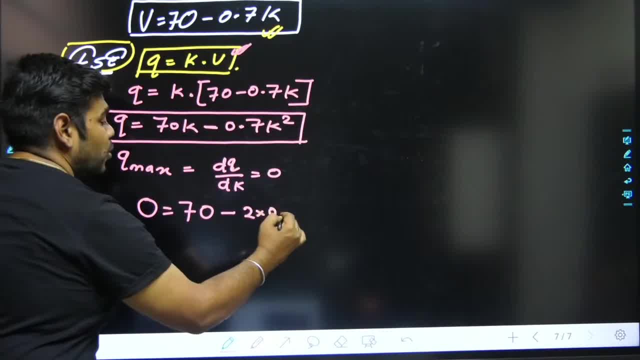 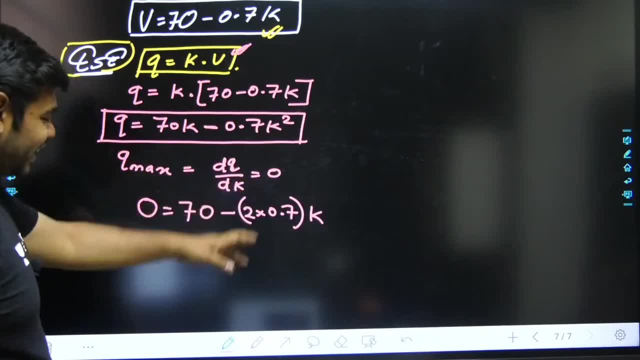 70 minus 2 multiplied by 0.7K, 70 multiplied by 0.2 minus 2 into 0.7K. So I mean, if you see from here then it will be, 2 into 0.7K is equal to 70.. 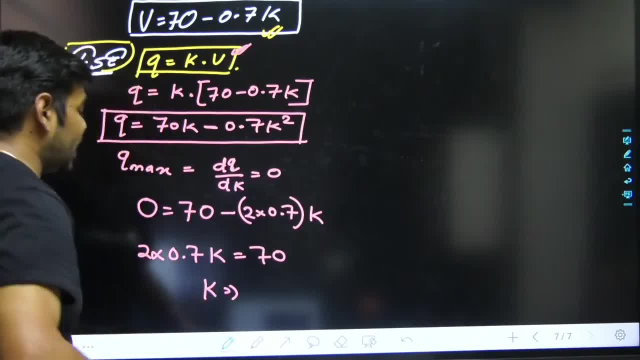 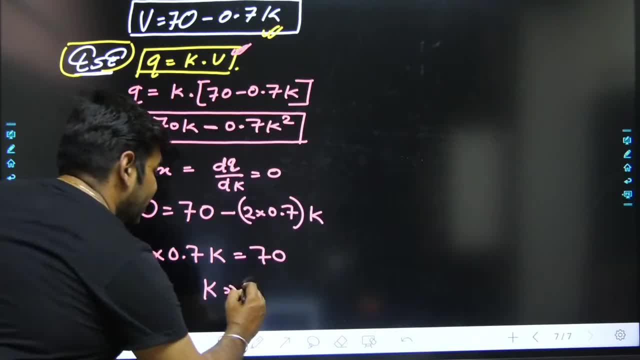 So I mean, take it from here and find out the value of K. So when you are finding out the value of K, then you will have. So from here the value of K will come. it is coming out as 50.. 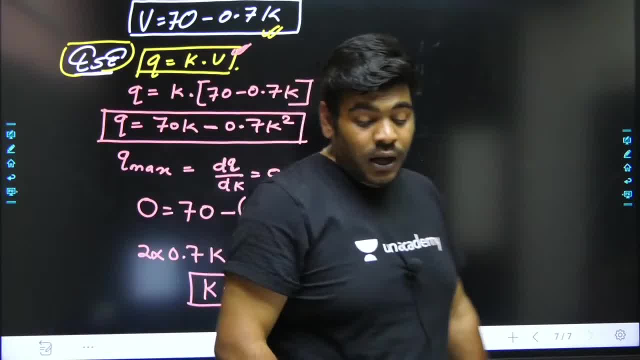 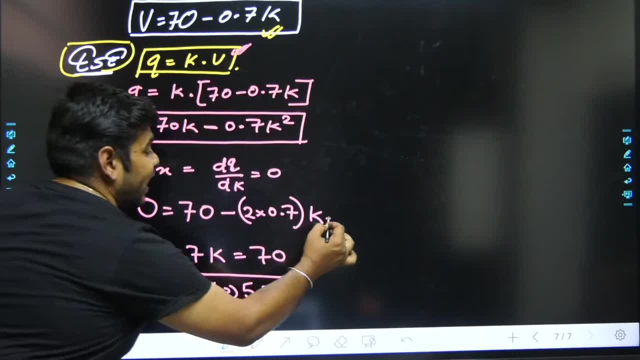 I mean the value that is coming to you, the value of K will come. it will be 50. Okay, it will be 50. And I mean, instead of K, what will become? It will become KJ. Why. 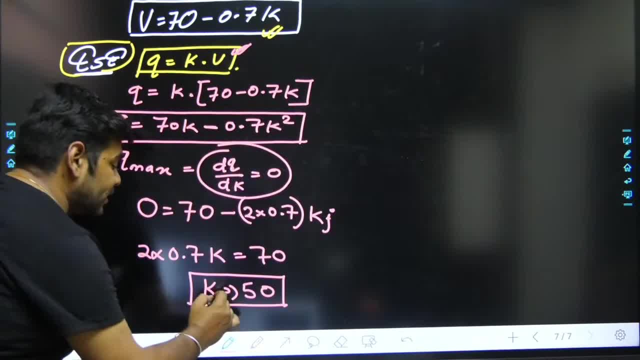 Because you are talking about DQ by DK, the maximum. You are talking about the maximum, So the value that will come to you, the value of KJ, will come. I mean the value that will come to you from here. 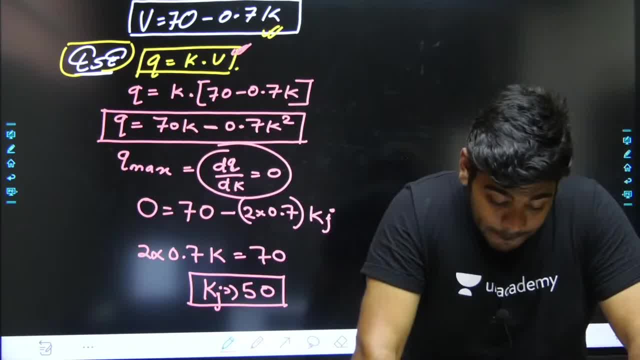 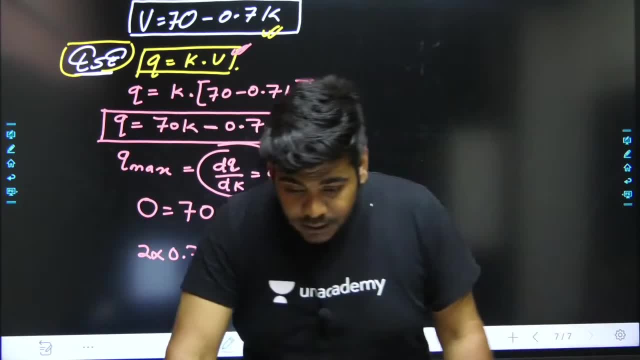 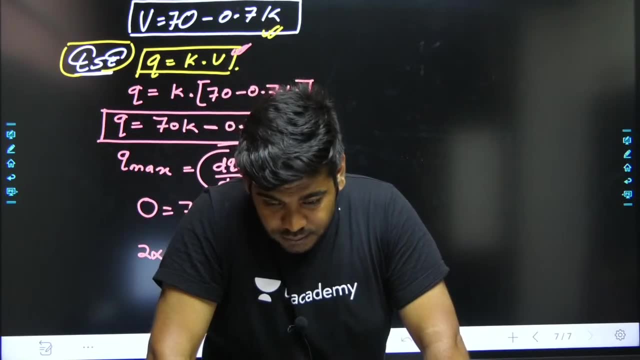 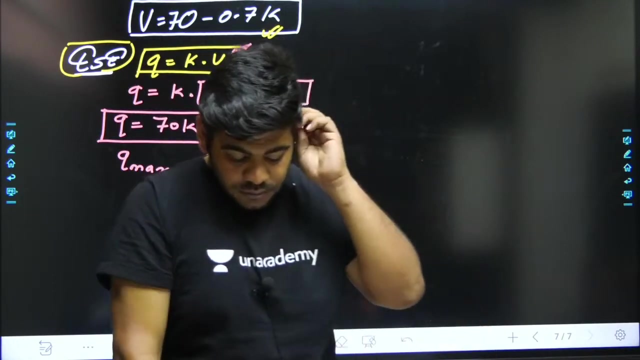 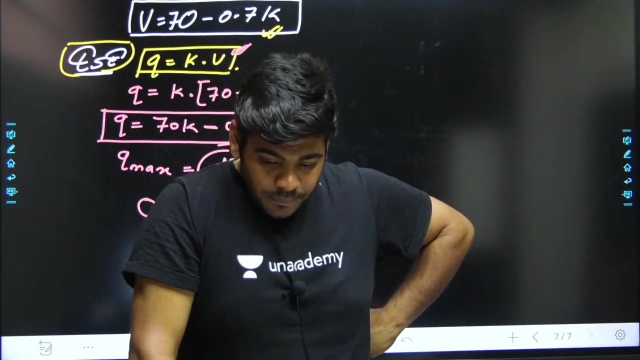 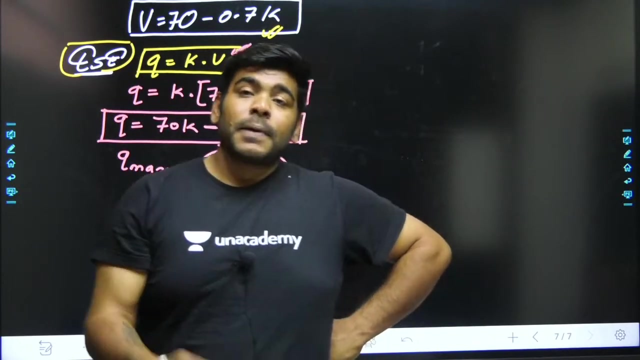 Whose will it come? The value of K maximum will come. What are you saying? It will be the value of KJ by 2.. I am reading: What will it mean? You will get blocked. You will not be able to see anything. 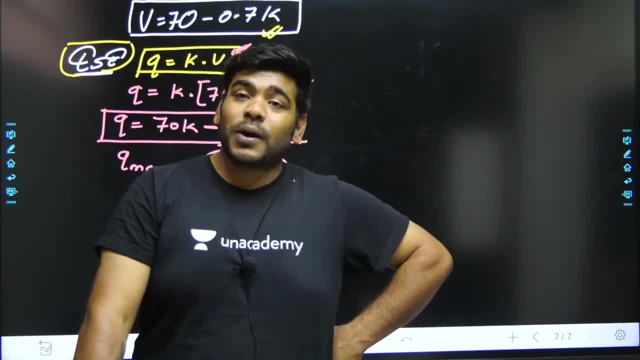 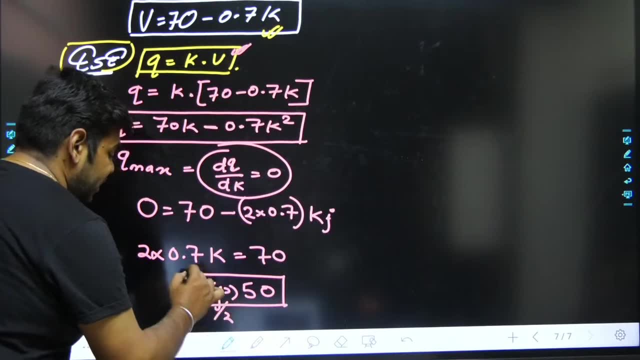 You will not be able to see anywhere And sir will not even read everything completely. Q max K is equal to KJ by 2 will come. This value will come. this KJ by 2 will come. This value will come. this KJ by 2 will come. 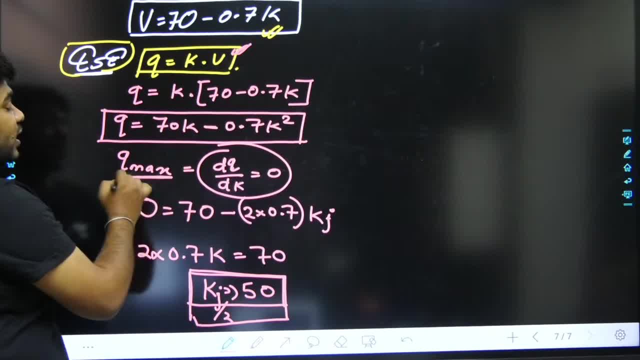 Okay, So I mean what we are talking about, which we are talking about this Q max. So the value that comes on who this KJ Looking at 2, it comes on. so it means that the value that will come from here. 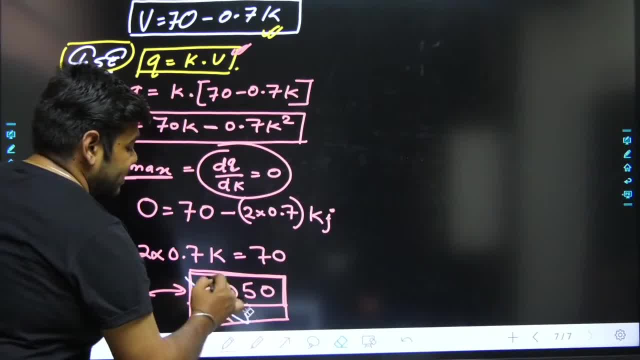 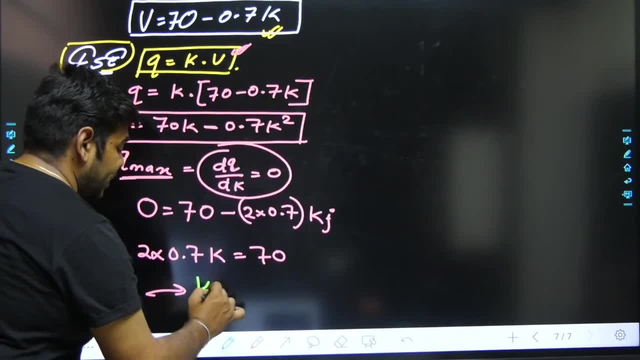 this KJ by 2 value will come. Okay, So I mean, this value appeared in front of you. whose name came? This KJ by 2 value came. This value appeared. this KJ by 2 value came, and how much does this KJ value came in front of you. 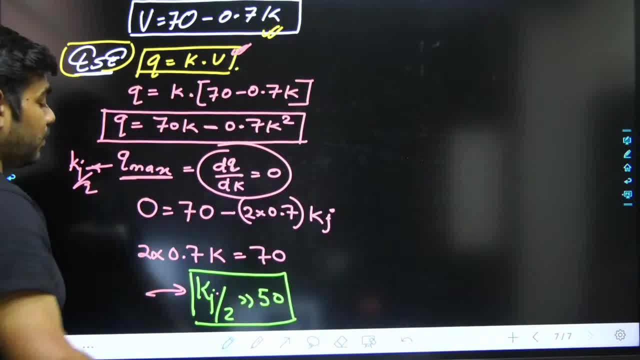 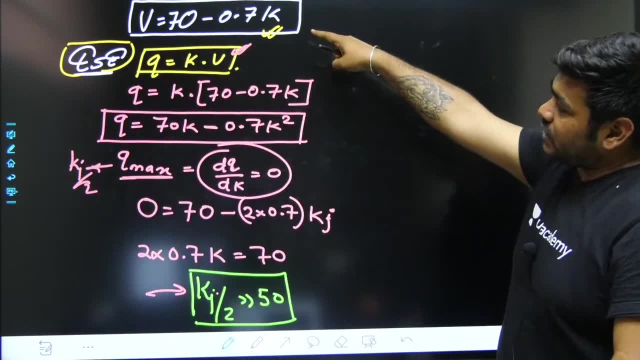 50 came. OK, You have a KJ value of two has come. I mean, what are you going to do here? you have the value of K is equal to KJ by 2? You mean, keep it aside. When we put the value of K here, then the value of V will come. and how much is the value of V coming from here? take it out and tell me. 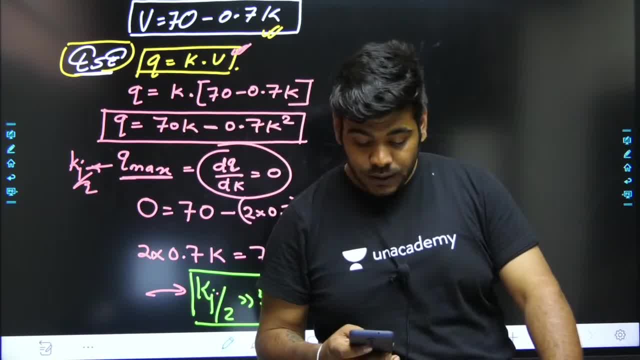 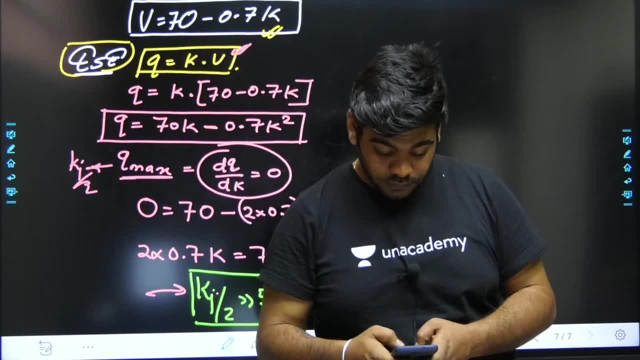 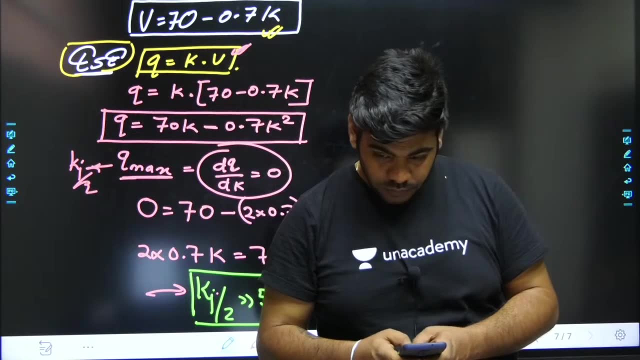 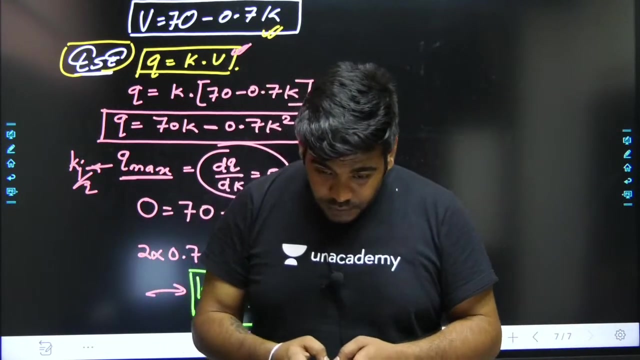 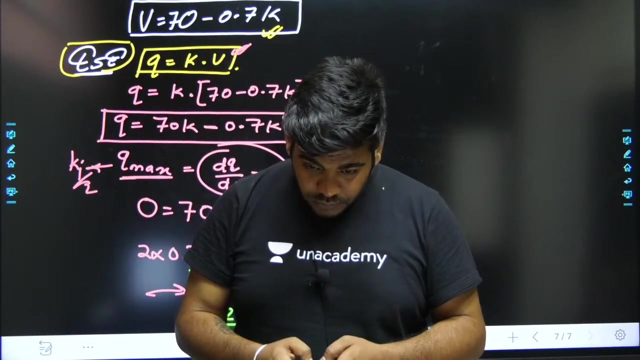 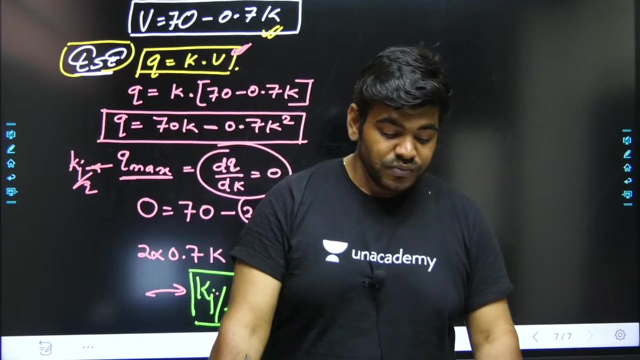 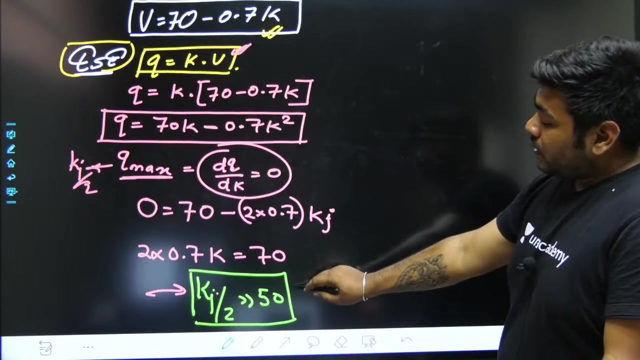 Wait a minute. wait a minute, I will remove your pain. What is your name? Okay, So that's it from here. You took it out from here. What is the value of K? Kj by 2 has come. 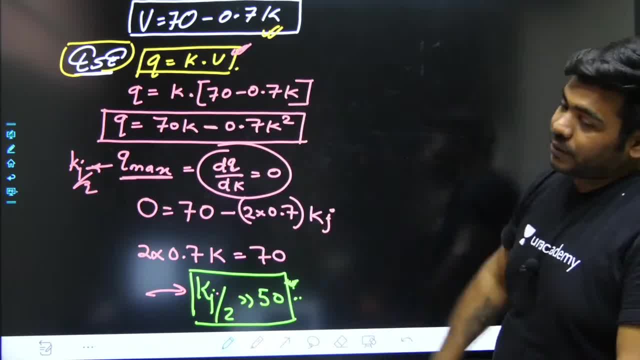 You have taken out the value of Kj by 2.. The value of 50 has come. You will put it in V. How much is the value of V coming? Tell me How much is the value of V coming. Take it out. 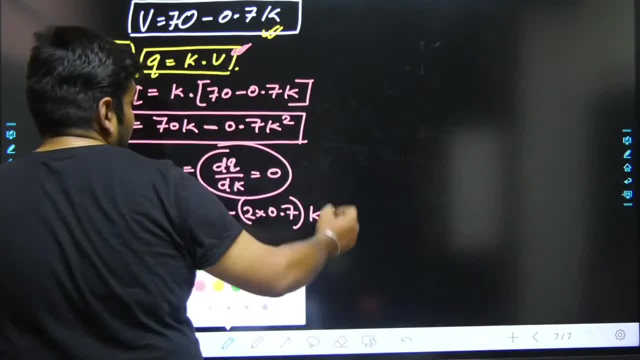 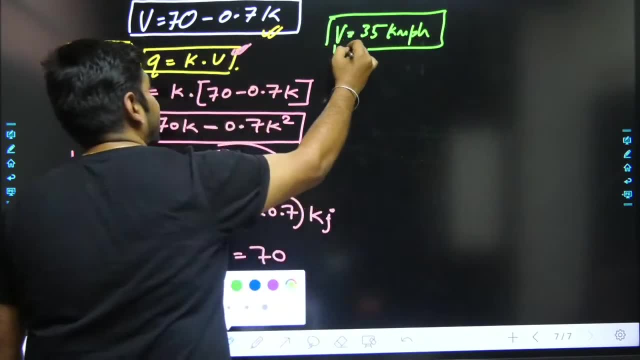 So the value of V that you will take out from here, your V value will be coming, Whatever value of V is coming. someone said that 35 is coming, 35 is coming, 35 Kmph. I told you that the value of V that is coming, whose value is it? 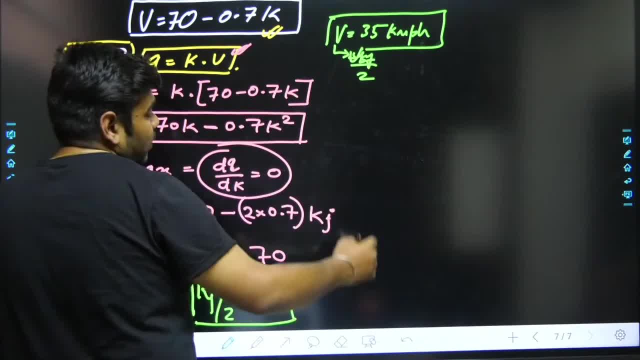 It will be the value of Vsf by 2.. It will be the value of Vsf by 2.. So I told you. So we will talk about Qmax. So what will you say? Qmax is equal to 50 multiplied by 35.. 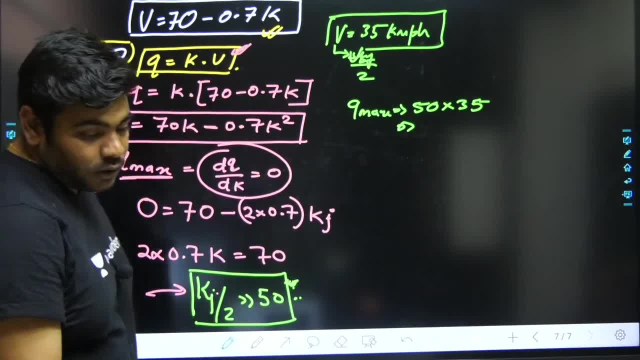 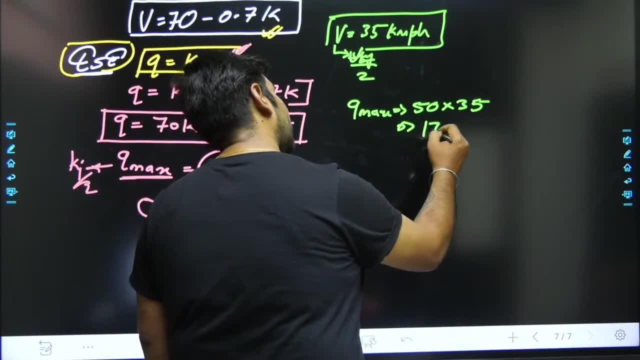 How much value is coming. If you do 50 multiplied by 35, then how much value will come. So I mean, how much will this value come? 50 multiplied by 35, this will give you 1750.. So I mean the value that will come. it is coming out as 1750. 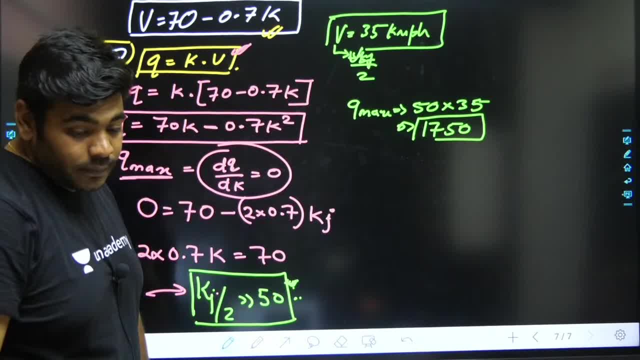 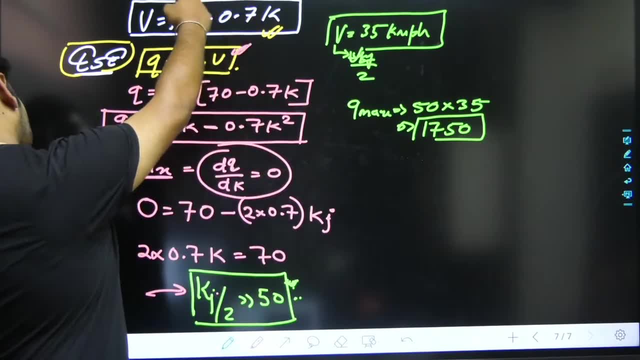 Okay, The value that will come from here. how much will come? 1750 will come. Okay, The value that will come from here, how much will come 1750.. When you will put the value of K from here, then it will come. 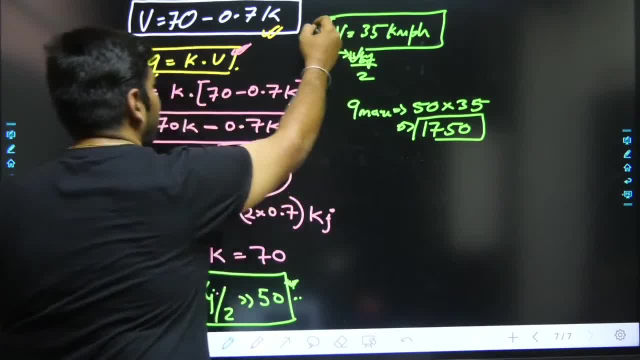 When did the value of V come? Okay, Don't worry about this. Where did it come from? I mean, you put the value of K here. If you put your K here, then the answer will come. Your velocity will come 35.. 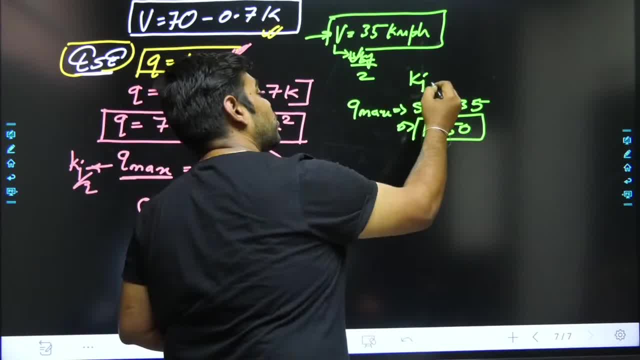 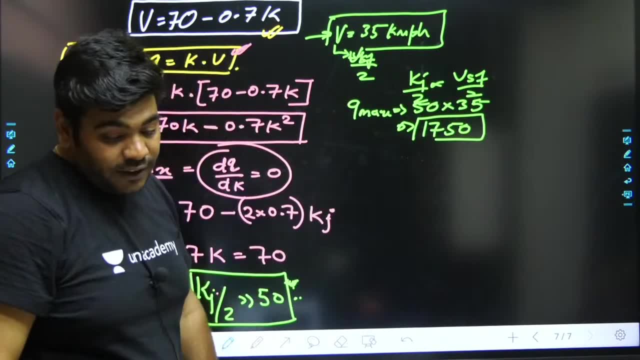 And Qmax. you know what it is. Qmax is Kj by 2 multiplied by Vsf by 2.. Kj by 2 multiplied by Vsf by 2.. So you saw the value that came: 35 multiplied by. 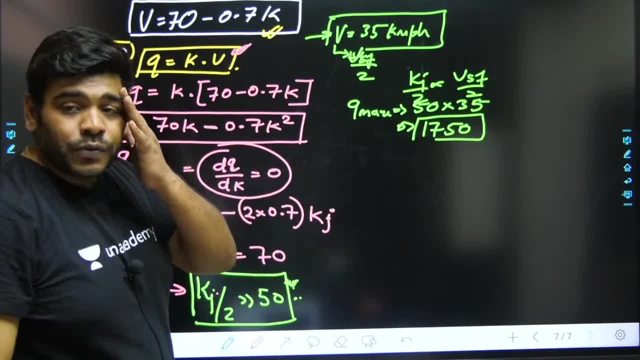 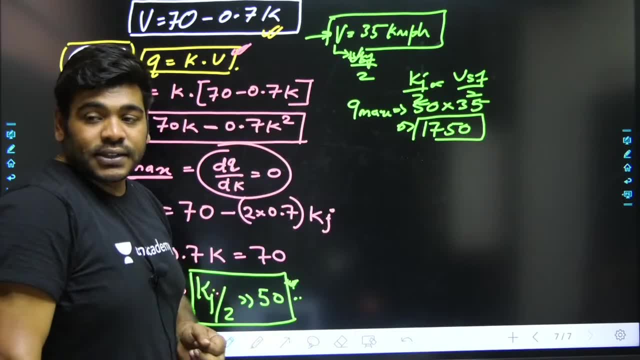 Okay, Okay. So the value came till here. So this is done. For whom were we talking? We were talking about engineering services. I mean, for whom were we talking? We were talking about engineering services. Okay, I mean, if you were asked the same thing in the gate, then I mean look here, look carefully. 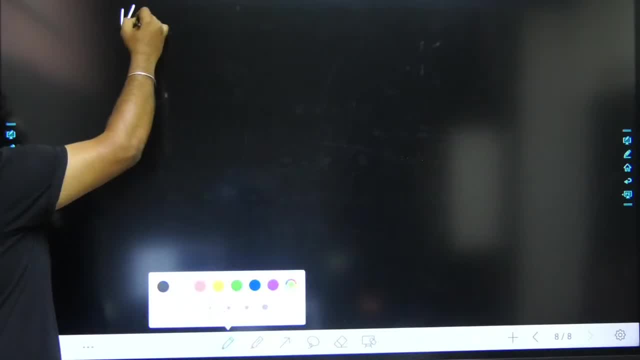 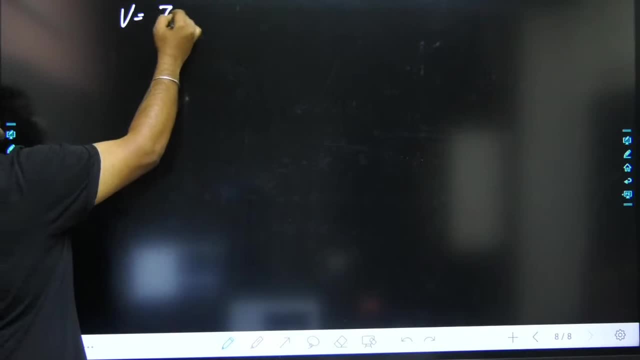 what I am saying. a lot of drama has happened. I mean, if I had talked to you in the gate then this velocity would have given you. it is 70 minus. Look here the velocity was given. it would have given 70 minus 0.7 K. 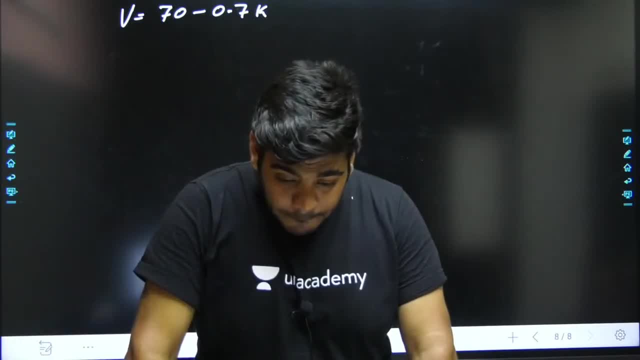 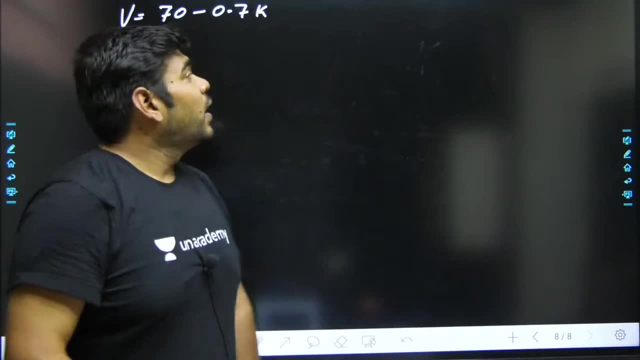 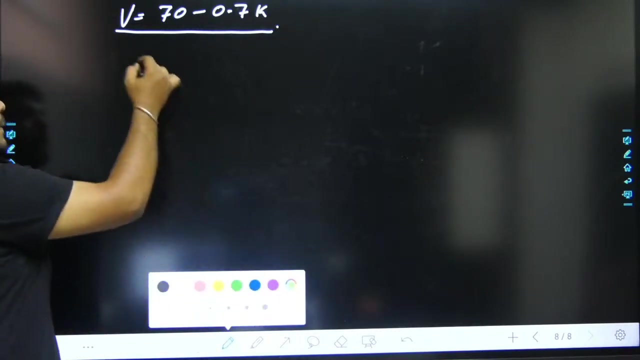 Okay, Okay, Okay, Okay, Okay, Okay. so I said: look here, if I had talked here, velocity v is equal to 70-0.7k, and if you are sitting in the gate exam, then how do you approach this question? look carefully. 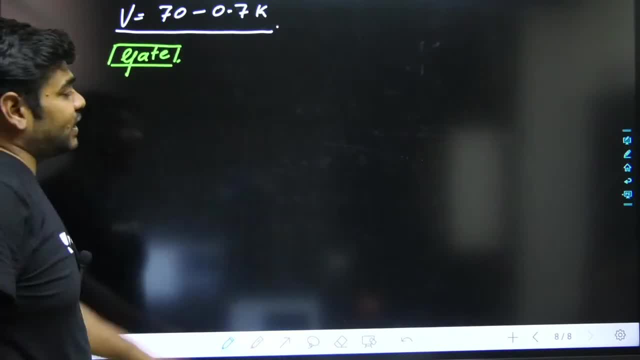 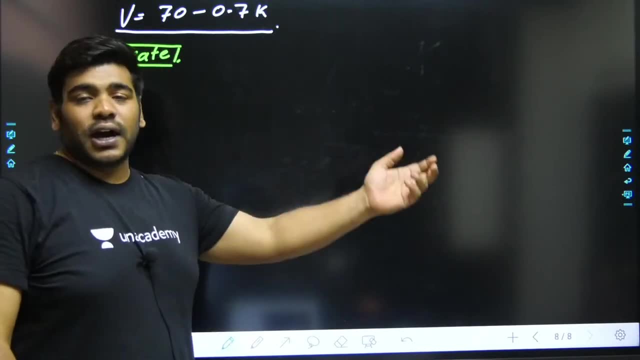 I mean, if you are sitting in the gate exam, then I have told you the conventional approach, that how you are doing conventionally, because if you learn that question according to the gate, then you will never go on that approach, on the conventional approach, and this is always. 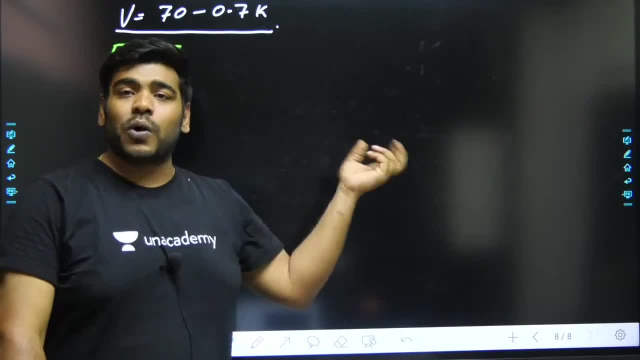 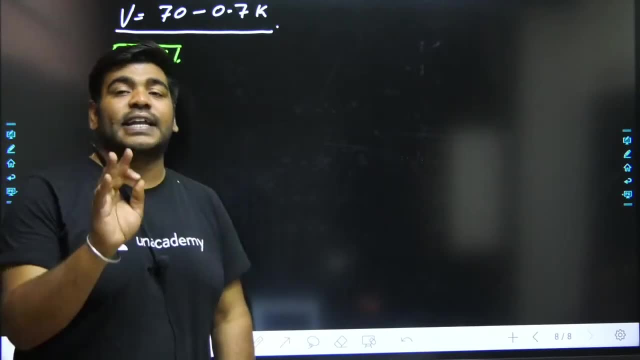 the problem that you will come to the question of number 4 or 5 in one line, which we do not have to do, which we do not have to do. so what is our motive? now we will see according to the gate, and you know that gate exam tells us that we have to steal time and when we 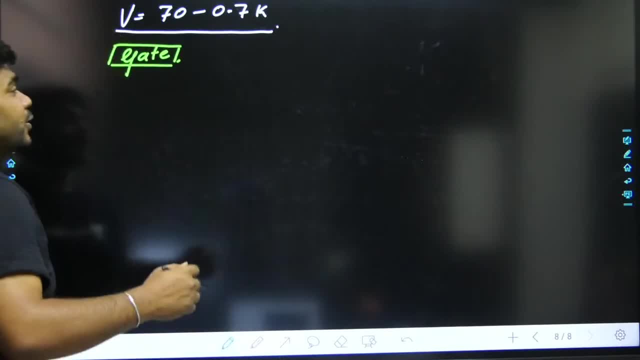 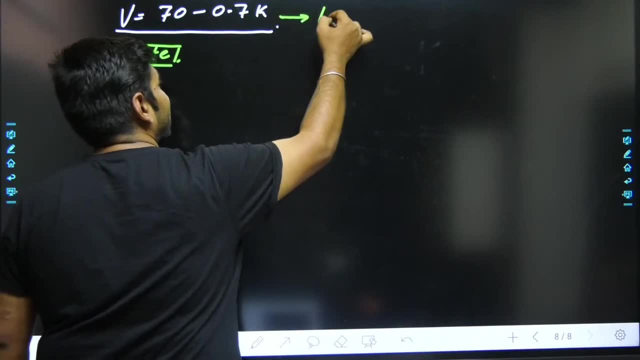 have to steal time, then see how you are stealing time from the rest of the people. so what will you do to make it better than the rest of the people? see here. I said: when you know this graph, who is he talking about? he is talking about linear relation. I said: 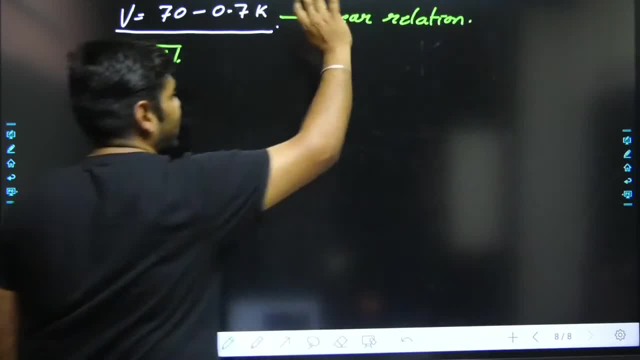 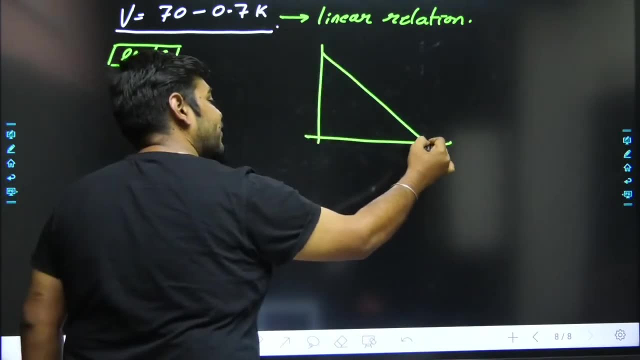 yes, who is he talking about? he is talking about linear relation. yes, yes, sir, this is talking about linear relation, and if he is talking about linear relation, it means that you know this graph very well, that this is a negatively sloped graph. this value is: 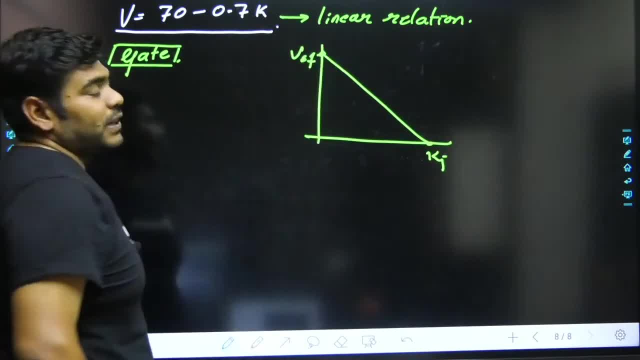 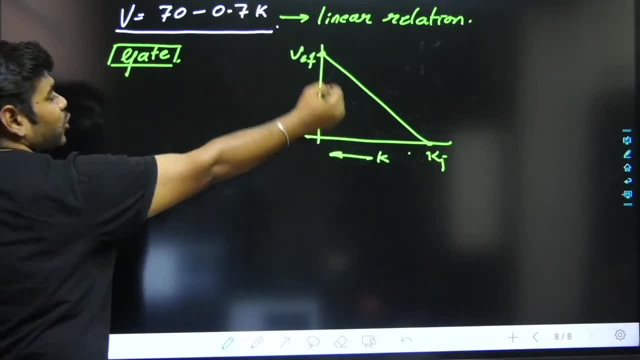 KJ and this value is Vsf, say yes, you know. so when I will talk about K is equal to when this is the value of K. when I will put it to 0, then when I will put the value of K. 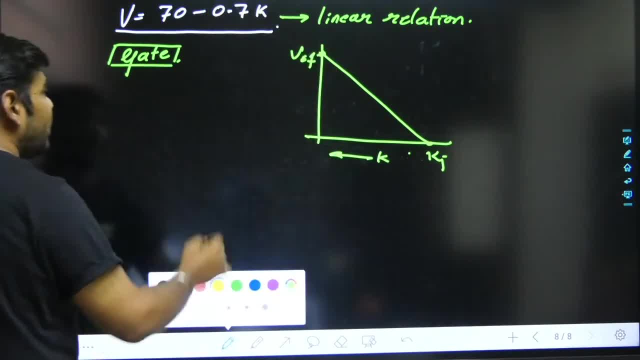 to 0,, then will I get the value of Vsf? yes, sir, I will get it. so I will put the value of K to 0, so as soon as you put the value of K to 0,, put the value of K to 0, then. 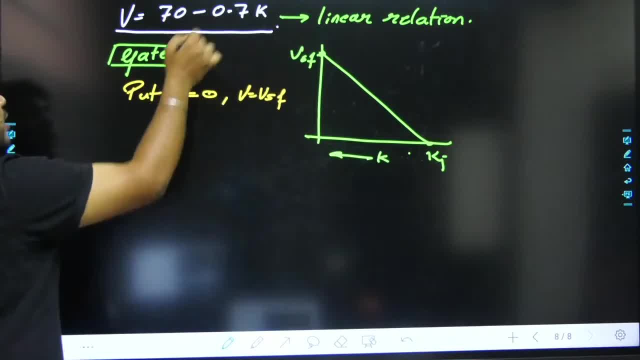 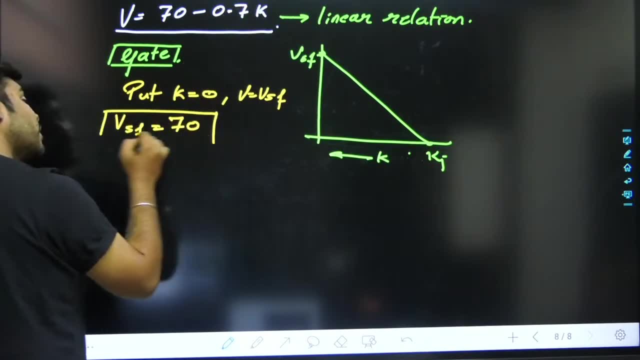 what will you get? you will get: V is equal to Vsf. so I mean, see, here, this will happen. Vsf is equal to. as soon as you put the value of K, then you get the value of Vsf. you get. 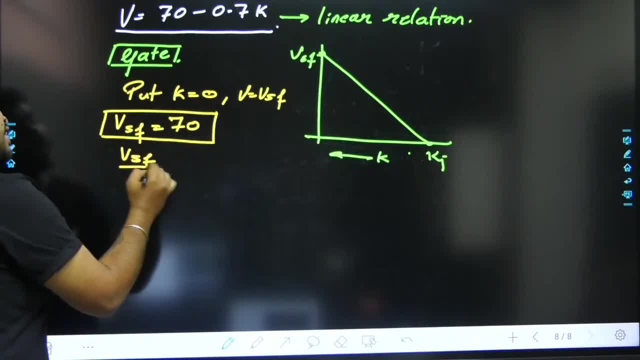 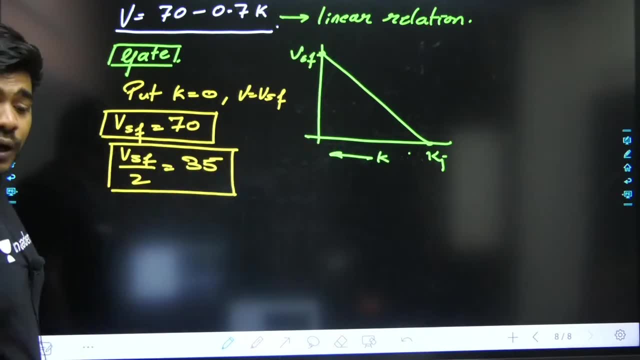 70,. I mean the value of Vsf is 70, then if you take out Vsf by 2 from here, then what will be the value? it will be 35, I mean how much this value will come in front of you. 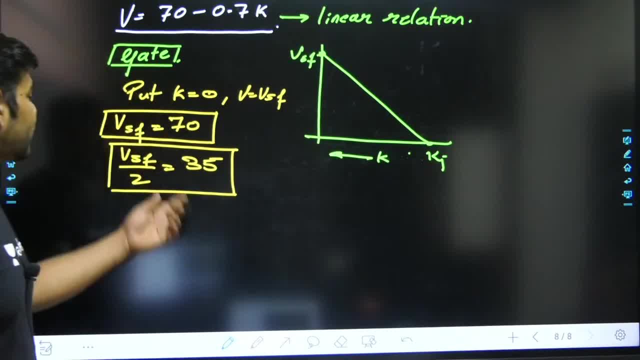 35 will come right. so you came to the value of Vsf. I mean, the value of Vsf came in front of you, and if you have the value of Vsf, then what did you do? you put zero to K then. 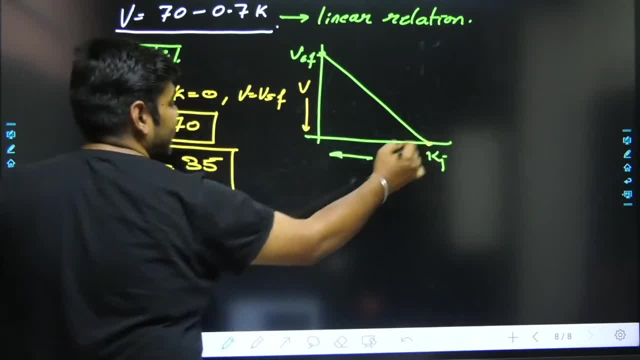 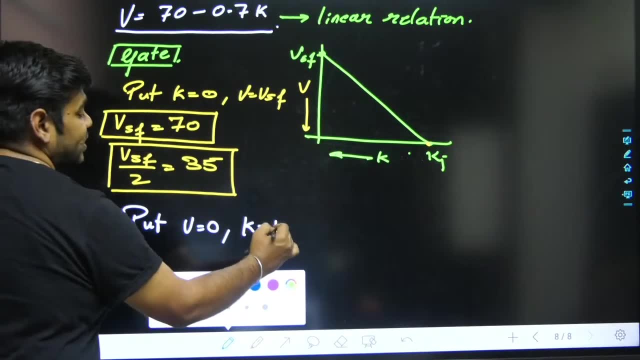 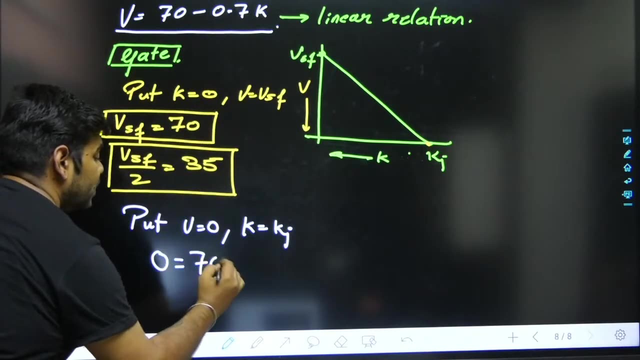 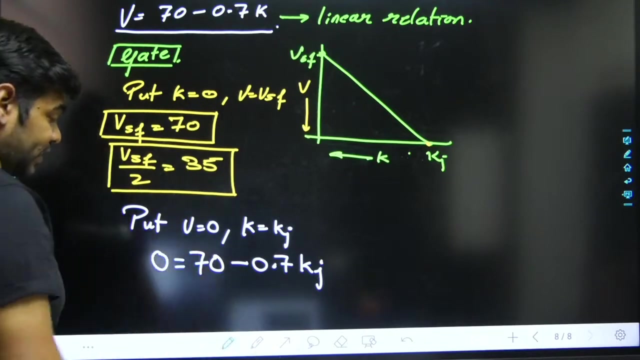 Now this time, if you put V is equal to 0, then K is equal to KJ. so what did I do next? I said: put V is equal to 0, so when you put V is equal to 0,, then K is equal to KJ. so if you put V is equal to 0,, then K is equal to 0, so this will be: 0 is equal to 70 minus 0.7 KJ. 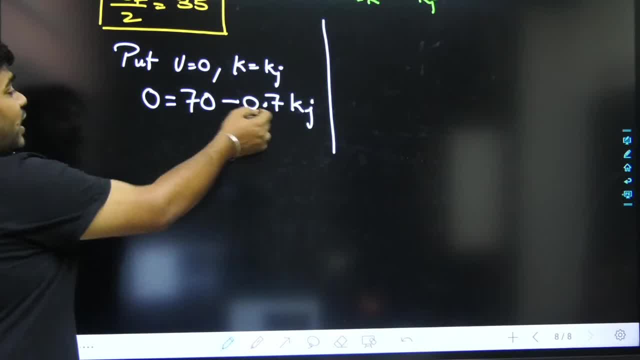 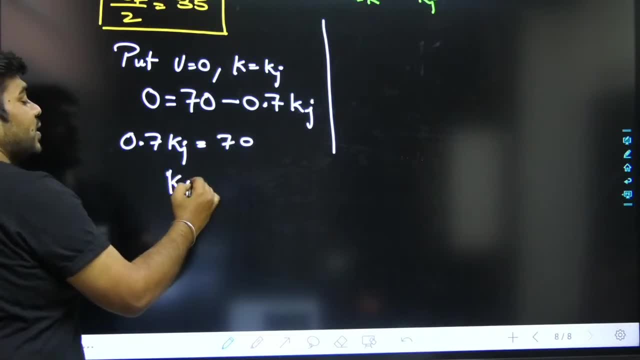 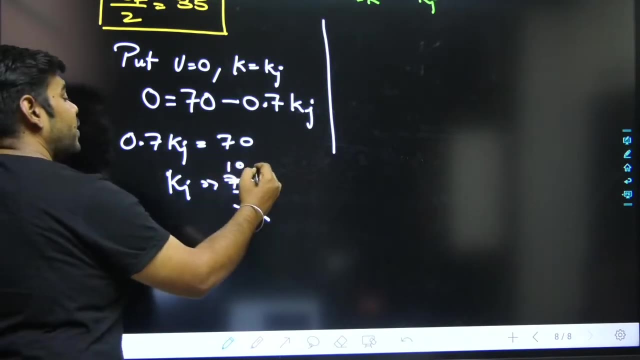 So let's solve it further. so the value that will be 0.7 KJ is equal to 70, so I said KJ is equal to 700 divided by 7, so it will be 100, so KJ by 2 will be 50,. 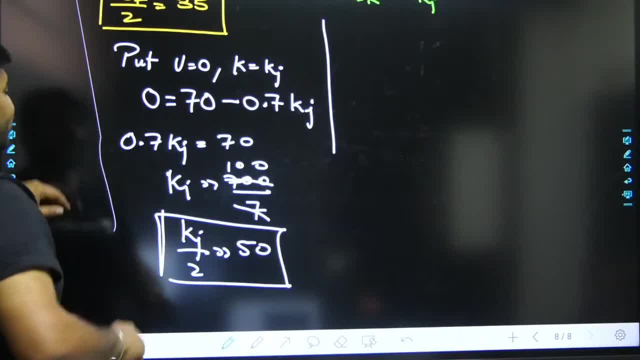 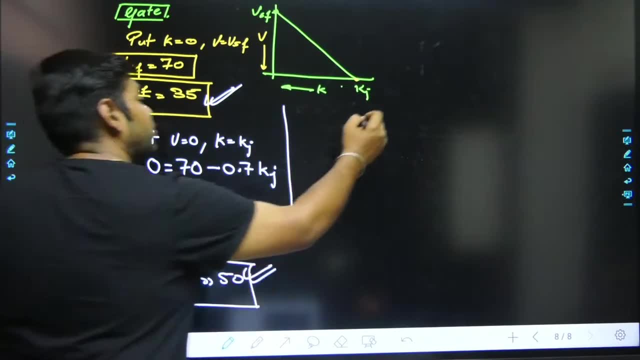 so your KJ by 2 is 50 and your VSF is: see, this is your VSF passion. your VSF by 2 is 35 and your KJ by 2 is 50.. So I thought, if someone will ask you, Qmax. 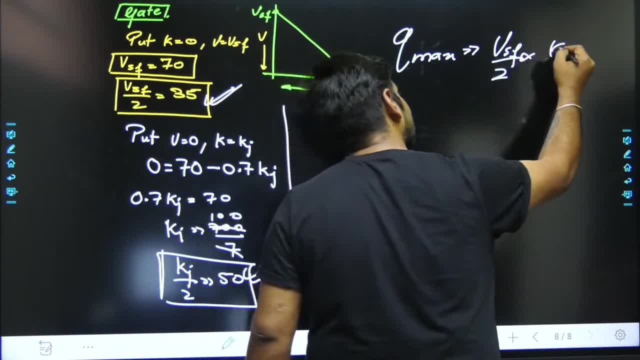 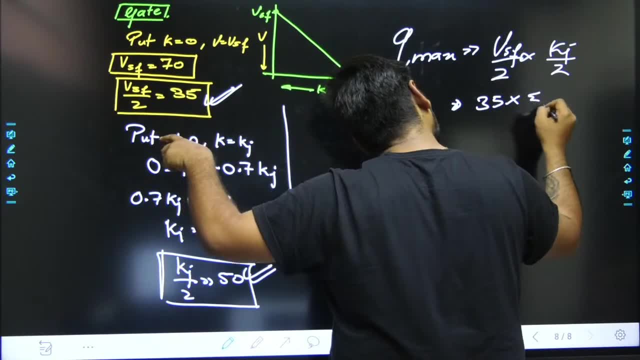 then you will be able to tell Qmax: it is VSF by 2, multiplied by KJ by 2.. So VSF by 2 is given as 35 and KJ by 2 is given as 50. So I thought the answer will be 1750 vehicle. 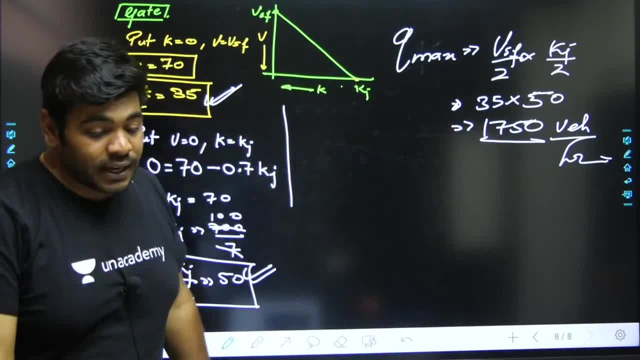 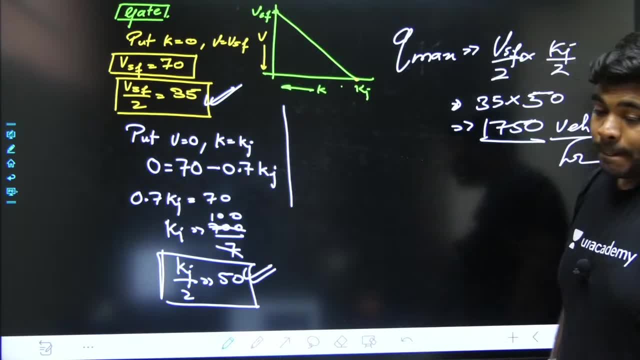 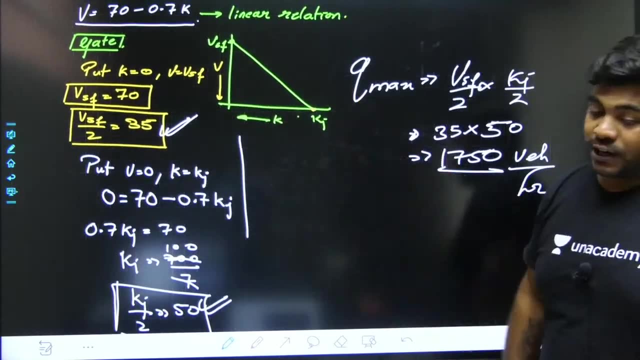 per hour, Say yes or no. Did everyone understand what I said? What do you say? What do you say? What do you say? I said that if you have to solve this question in GATE, then you are going to follow this method. I mean, let other people do it, Whatever they do. I have taught. 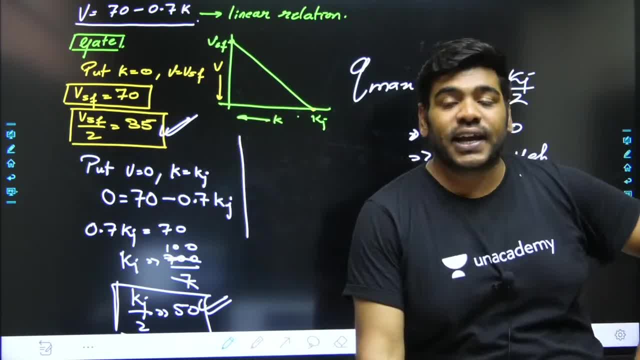 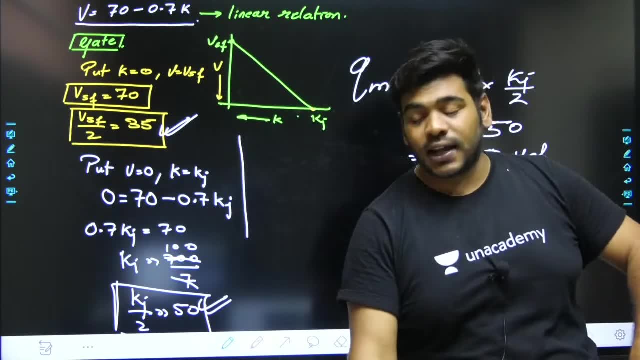 you the conventional approach and I told you the normal way that- how to solve the question in the GATE exam. Did you enjoy it? Did everyone enjoy it? Did everyone enjoy it? Did everyone enjoy it? I said this had to be done So. 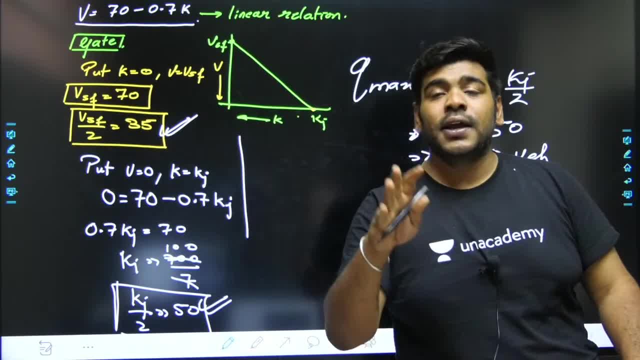 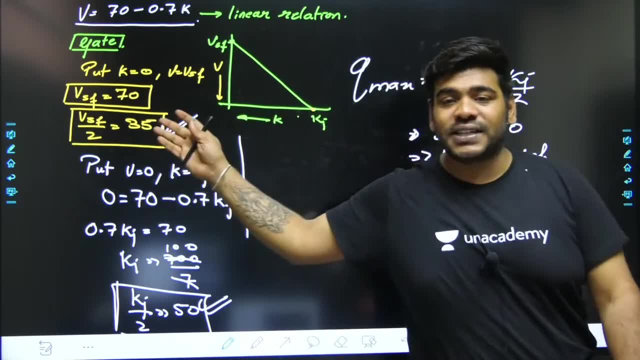 I told you to just steal the time like this from others. you have to keep hiding the time from others who are doing pretence. We have to do this only. It will be done in one line. Yes, it will be done in one line. I said this is to teach. You will solve the. 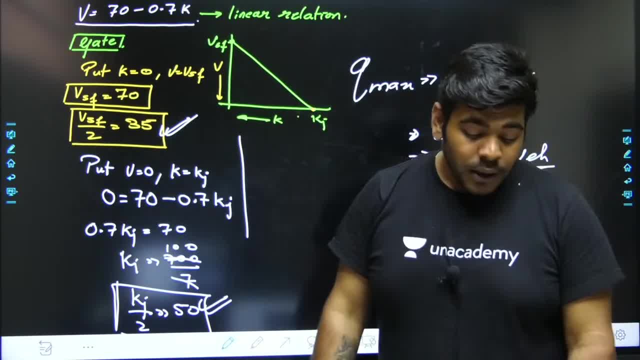 one more question. let's see how many times you get the answer. Let me see how long the answer will be given. Then here comes the second question. I look at the second question: how long do you answer As soon as I write that, If I take a little time to see the answer? 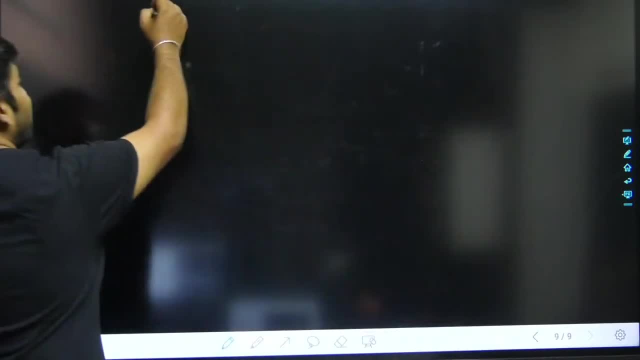 after a while. there is only one question to see. it will come in front of me And then, if I looks at my question, it will come back. Okay, continuing according to the te, Let's see how long you will answer Here. the expression of velocity V is equal to 53 minus 0.43k. 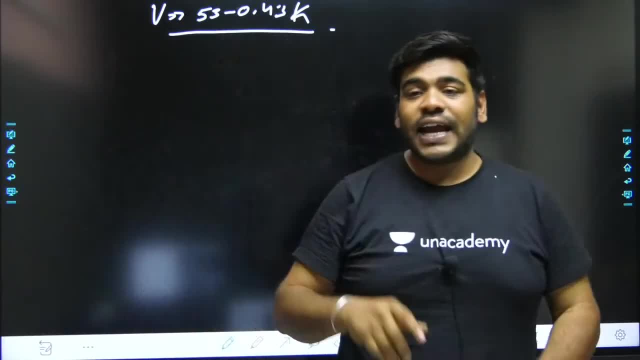 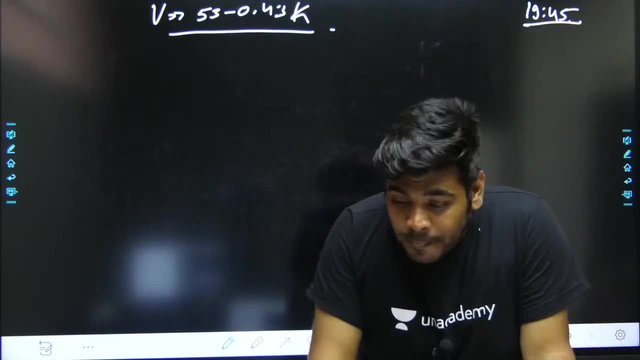 Your time starts now. My laptop has time of 1945.. Let's see how much is the first answer. does it come within a minute or not? Let's see whether the first answer comes within a minute or not. Let's see whether the first answer comes within a minute or not. 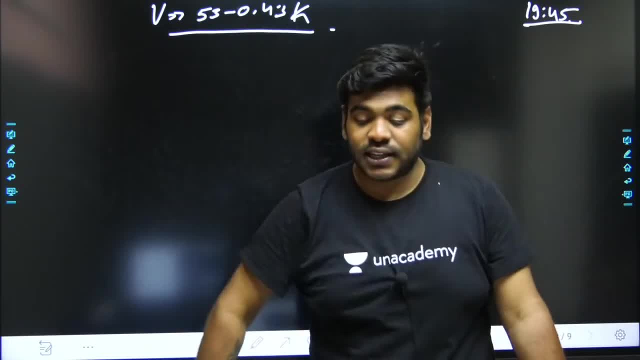 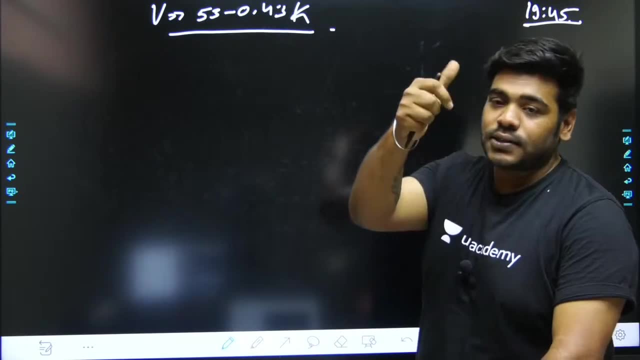 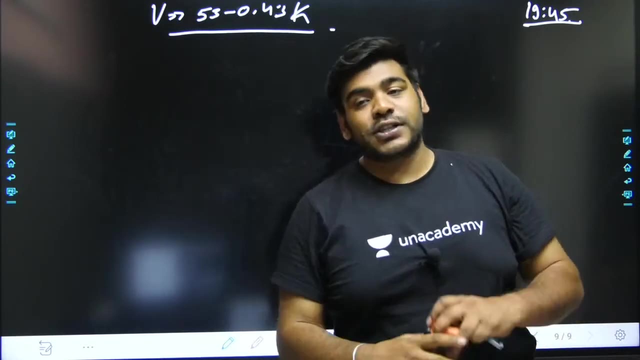 Come on, guys, fast, as fast as possible. fast Come on, let's see how fast your answer comes. So if you guys are enjoying it, like the session quickly, I don't have to say it every day to like it. I think they don't teach such approaches. 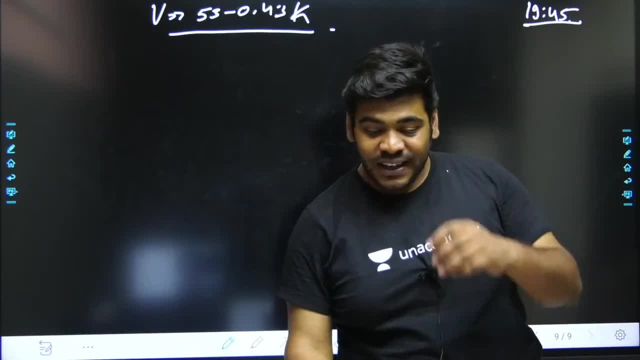 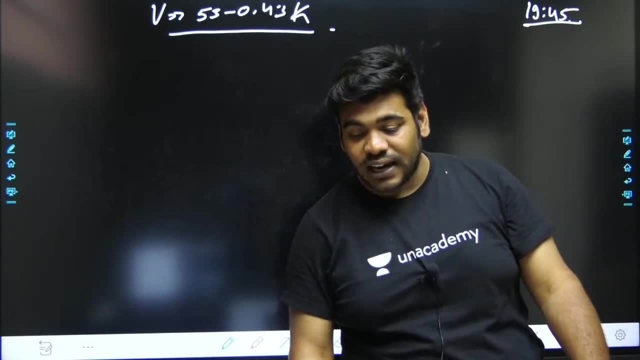 1633,. very good, the answer has come in the first minute. The answer has come in one minute. 1633.1213.. Okay, why are you taking out 61.63?? Who asked the value of k? The value of Qmax was asked. 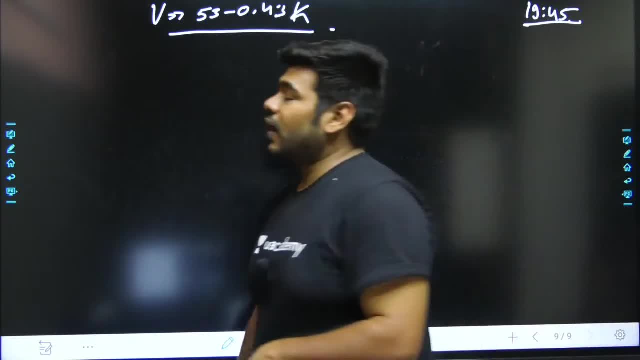 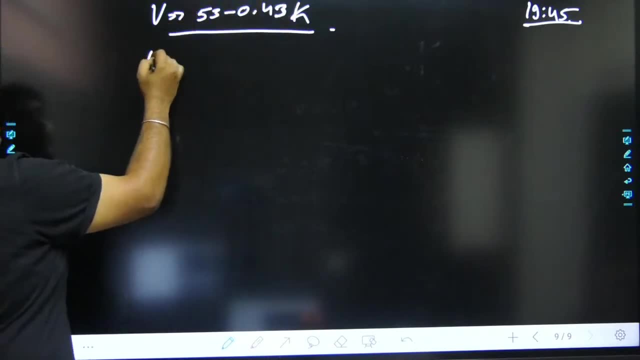 Qmax was asked 1633,. the answer has come from a lot of people. Very good, So let's see how everyone has approached it. I said if I want I can solve it in a minute. Let's see here. let's put the value of k as 0.. 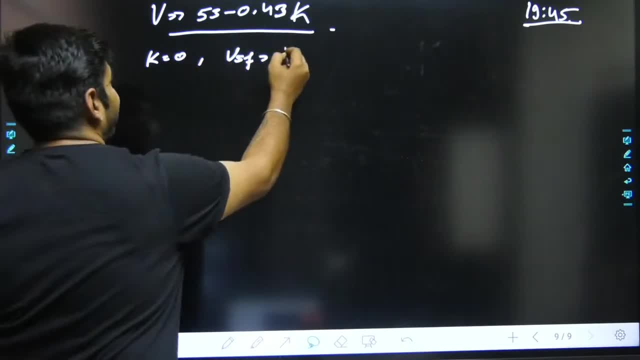 If I put the value of k as 0, then the value of Vsf will come and the value of Vsf will be 53.. The value of Vsf is 53.. I said, put the value of Vsf as 0.. 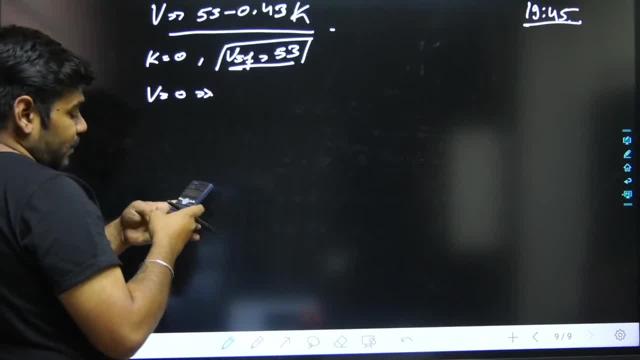 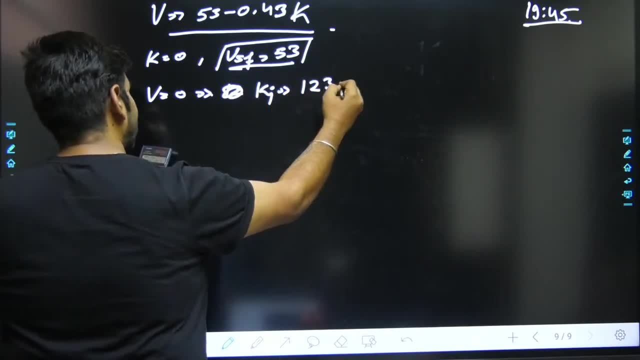 As soon as I put the value of Vsf as 0,, the value of Vsf will be 53 divided by 0.43.. The value of Kj will come. The value of Kj is 123.255.. I know Qmax. what is Qmax? 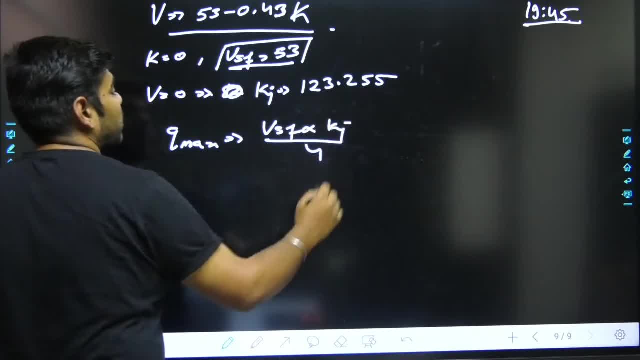 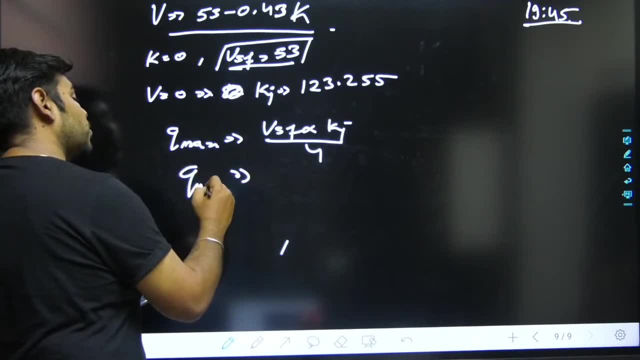 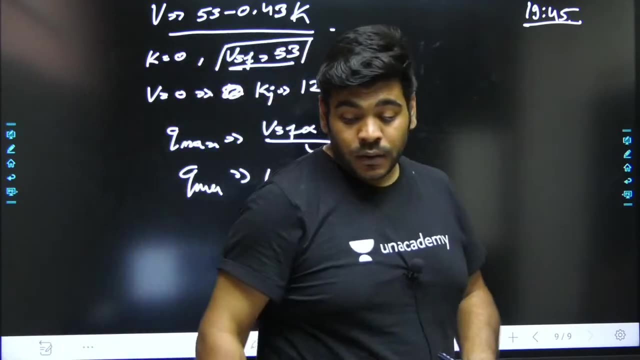 It is Vsf multiplied by Kj, divided by 4.. The game is over. I said here: multiplied by 53, divided by 4.. Here is the answer: Qmax is equal to 1633.139.. Here is the answer. tell me. 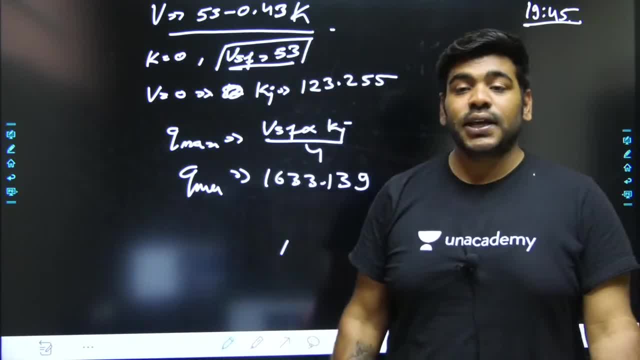 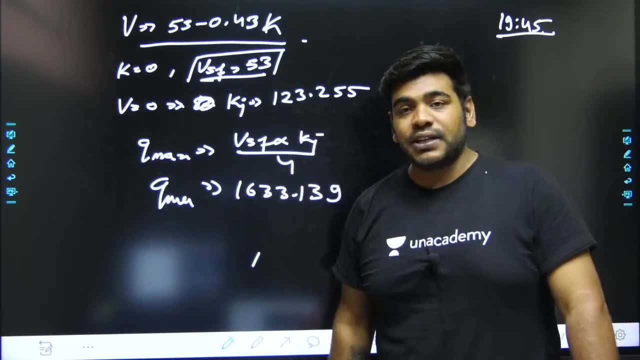 Very good, So I learned something new. I learned something new So I said: look, the question should be solved in one line from you. The question should be solved in one line from you. It is about gate examination, so it should be solved in one line from you. 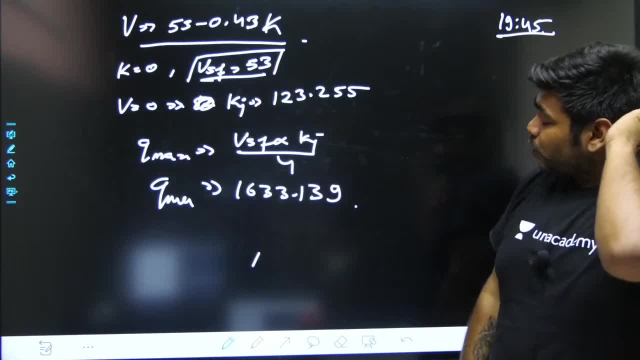 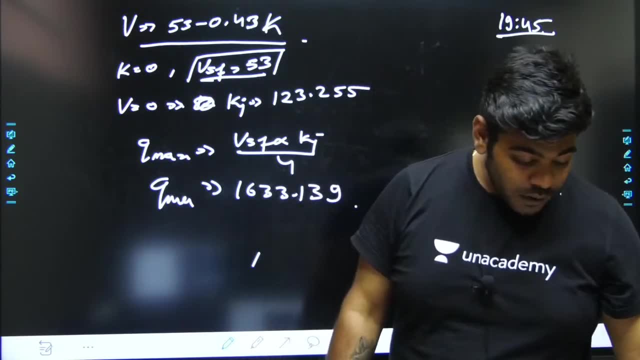 Okay, Okay. This is the Qmax thing. This is the Qmax thing. You have learned this. Come on, let's talk about the next thing. Let's talk about the next thing. Did I teach you any space headway? 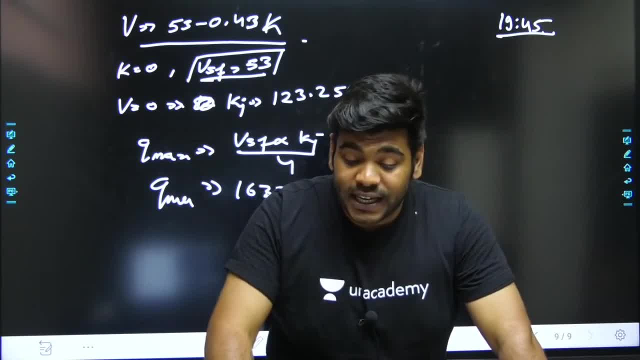 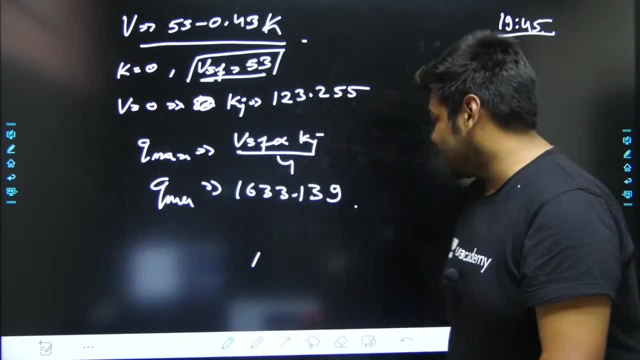 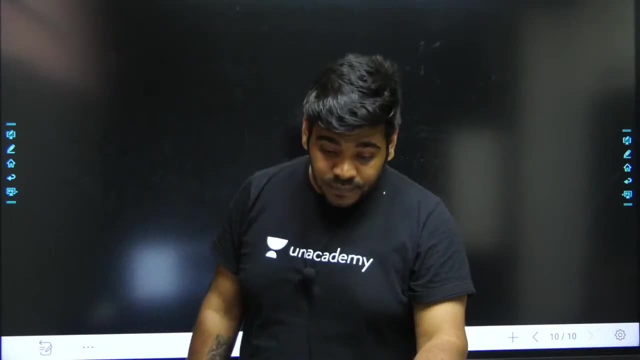 Did I teach you any time headway? Did I teach you any space headway and time headway? Tell me quickly. Really, sir, it is beyond our imagination. Okay, Okay, This will come again in the gate. There is potential for the gate. 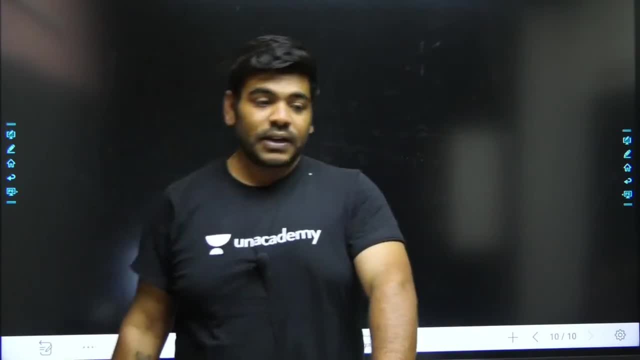 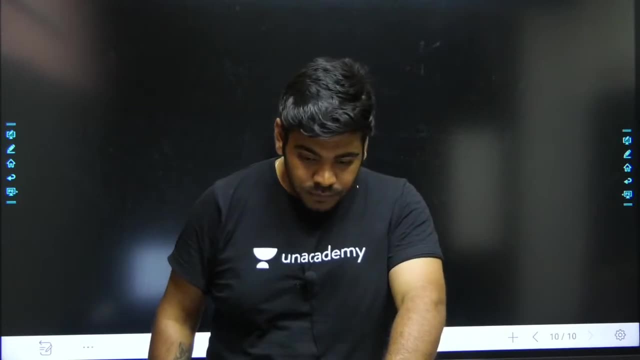 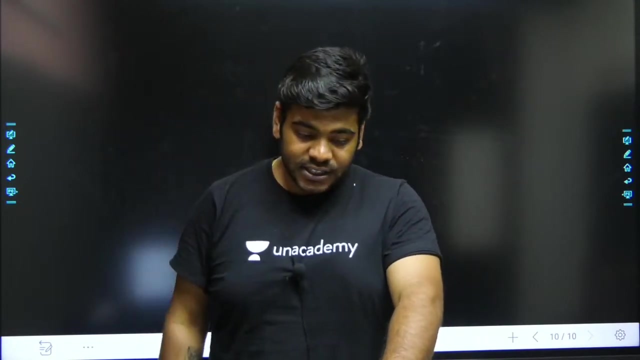 That means it is asked in the gate every time. That's why we talked about it. Okay, 1634 answer, Son. we were just looking at it like this, so 1634 will be the answer. Come on, let's talk more. 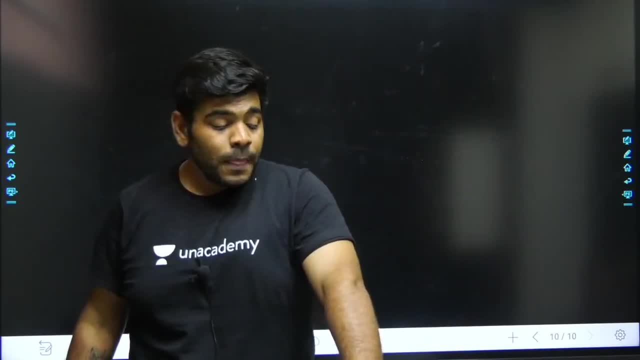 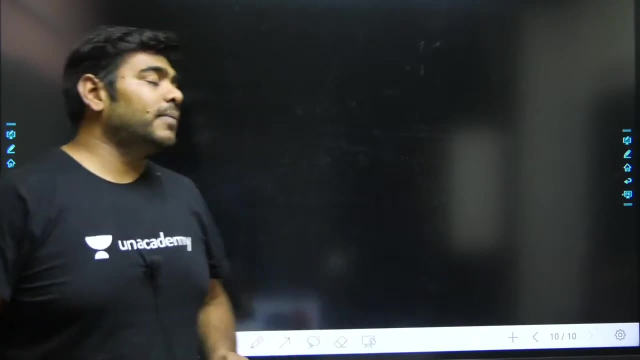 Manila, I had taught you space headway and time headway. So if I had taught you space headway and time headway, then I am talking to you about maximum traffic capacity. So, Manila, look here I am talking to you about maximum traffic capacity. 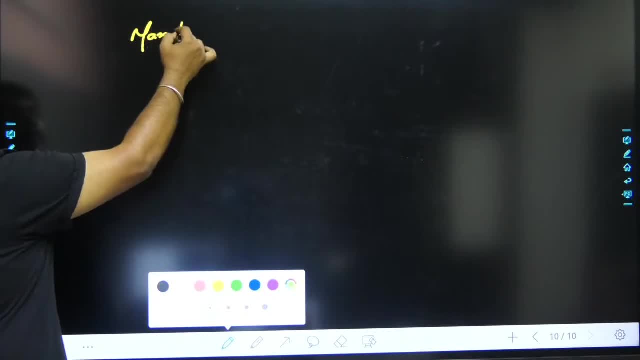 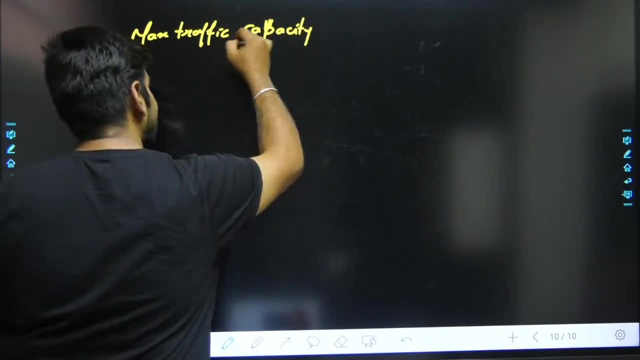 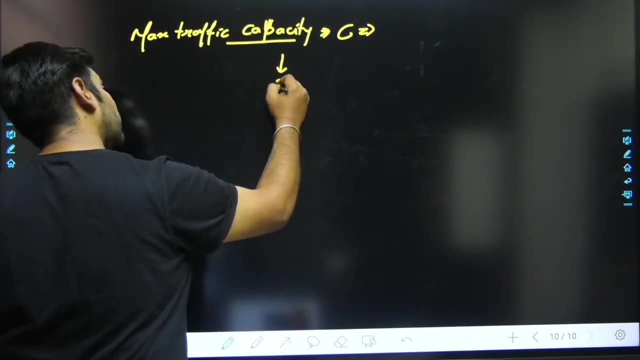 So look here I am talking to you about maximum traffic capacity, I am talking about traffic capacity. So if you want to find the traffic capacity C, you have to find the practical capacity C. So C means: does this traffic capacity mean Q? 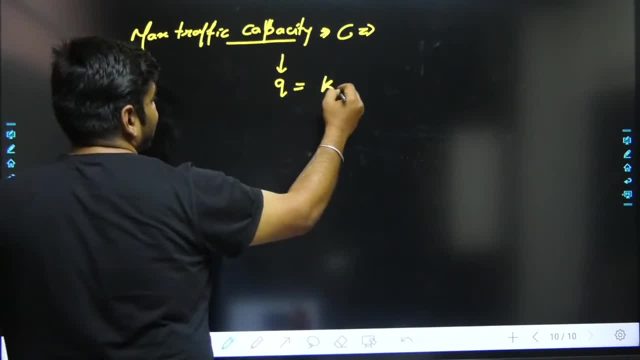 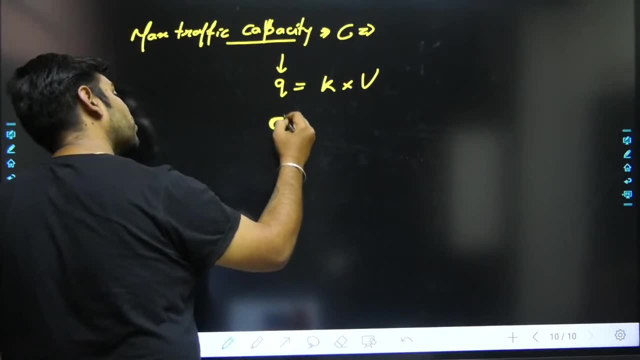 Say yes or no. So if Q is there, then Q is equal to what. It is equal to K into V. Q is equal to K into V. And you know what Q means. C, Who is Q representing The maximum value of the traffic volume is called capacity. 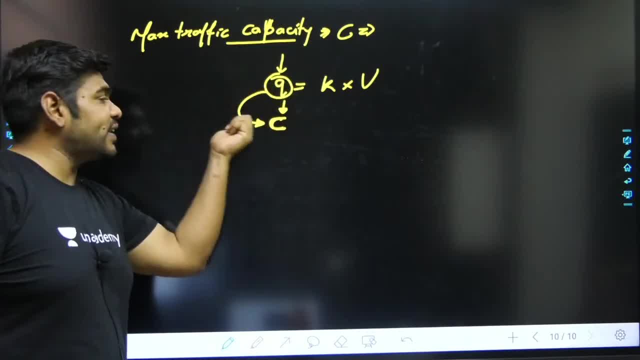 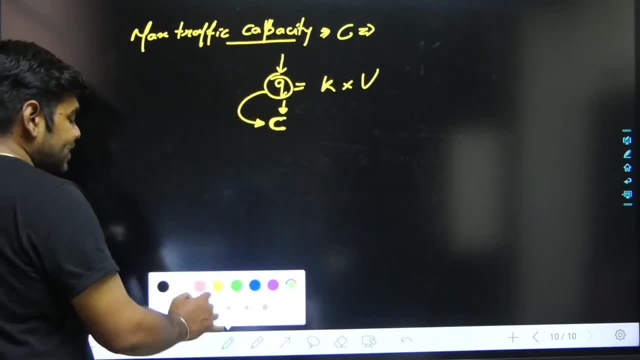 Say yes, I mean a special case of traffic volume in which you get maximum traffic volume. you call it capacity. What do you call it? You call it capacity. Okay, So you got this C value. So this C is equal to? what do you know about K? 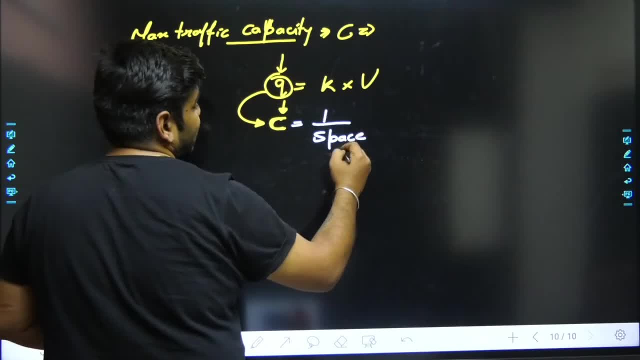 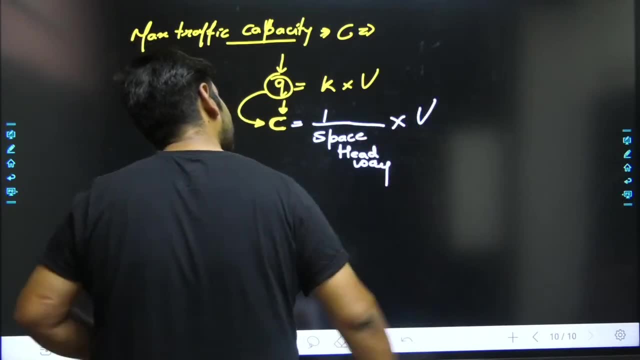 K is 1 upon space headway. Say yes or no. So what do you know about K? 1 upon space headway? So it is 1 upon space headway, you know? So okay, K multiplied by V, Okay, 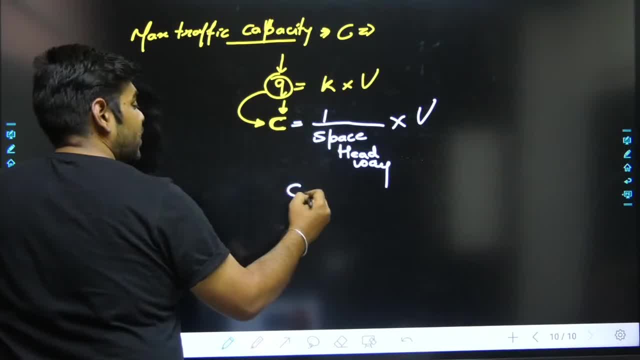 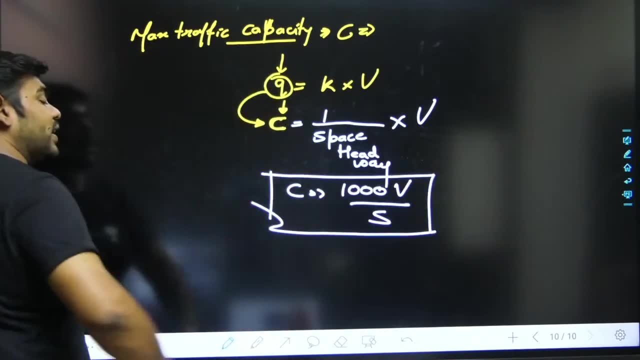 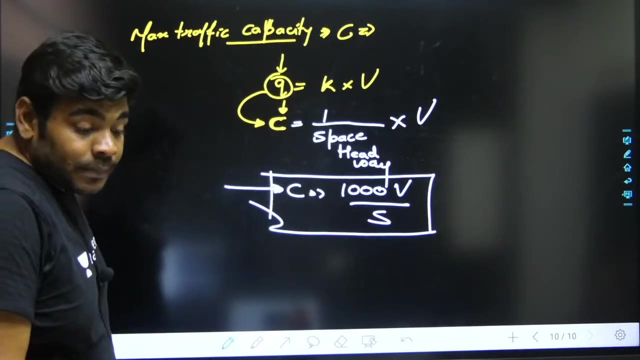 So I mean, if you convert space headway into this, then it says C is equal to 1000 V by S. So this is your capacity. If you are asked about practical capacity- practical maximum capacity is asked- then it is: C is equal to 1000 V by S. 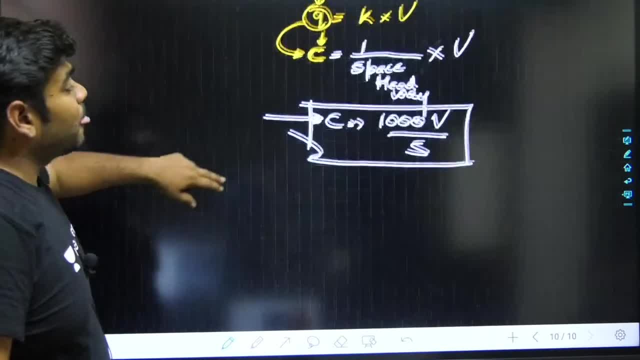 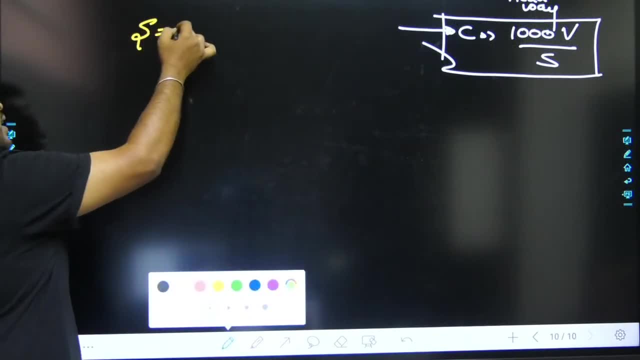 So I mean, what is this? equal to C is equal to 1000 V by S. Okay, If you understand this formula from here, then I will talk about the value of S. So what is S talking about here? So I mean. 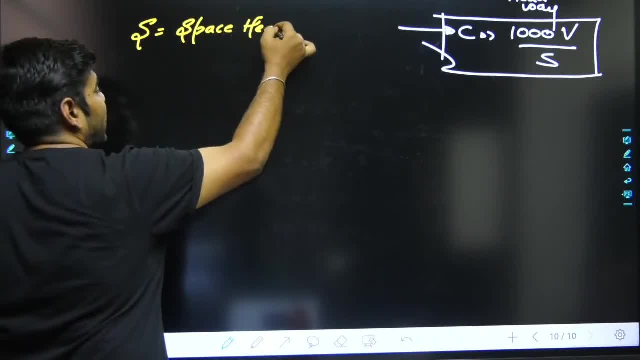 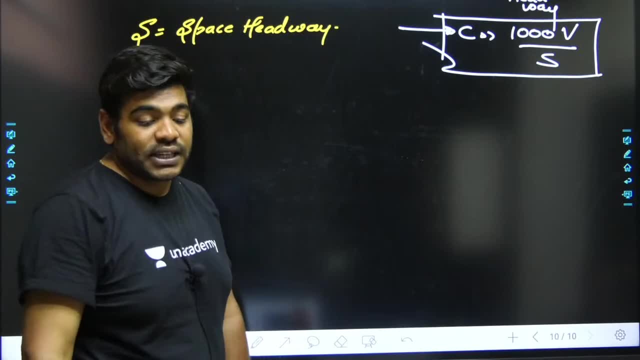 S is talking about the space headway here. I mean, who is this S talking about here? He is talking about the space headway here. I mean, listen to me carefully, listen to me carefully, I am going to connect something amazing. 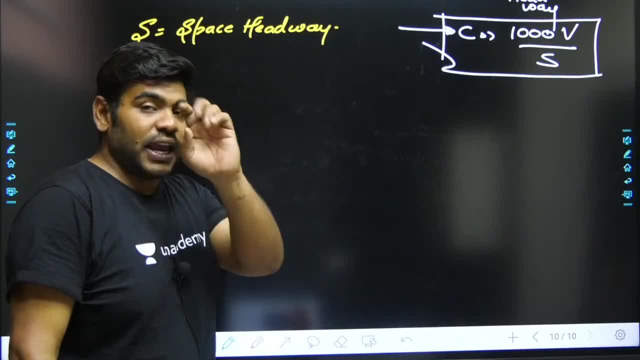 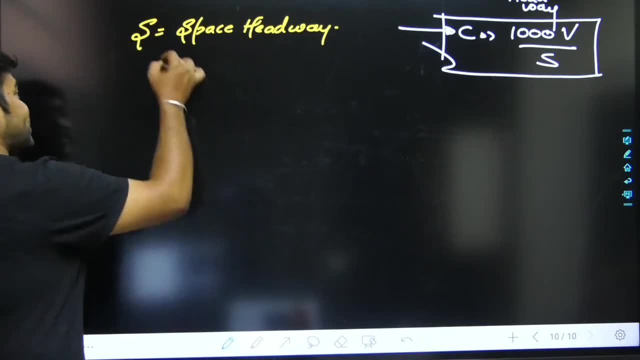 I am going to connect something amazing. just listen to me carefully. Listen carefully to each and every point, So I will connect you. I am going to connect you to a very good place. This S is talking about space headway. Okay, 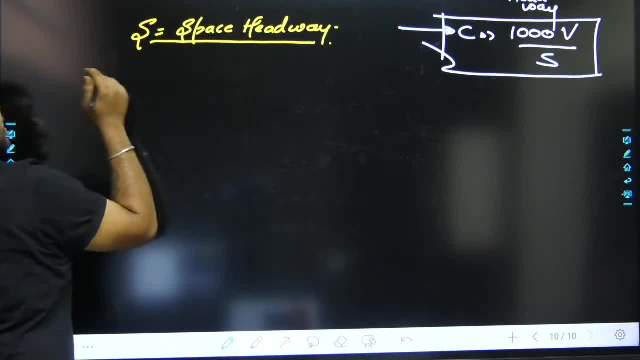 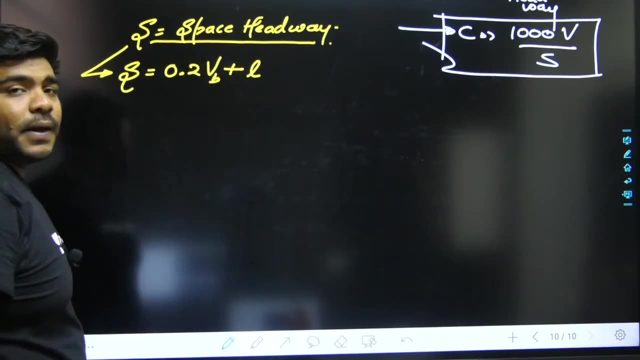 I mean this S. Watch carefully. I mean this S. If you don't have sufficient data given, then you know this S write it as 0.2 capital V plus length of wheelbase. Have you seen this somewhere, And what was the meaning of this capital V? 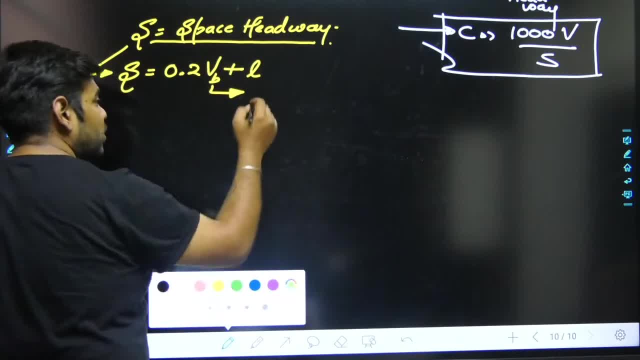 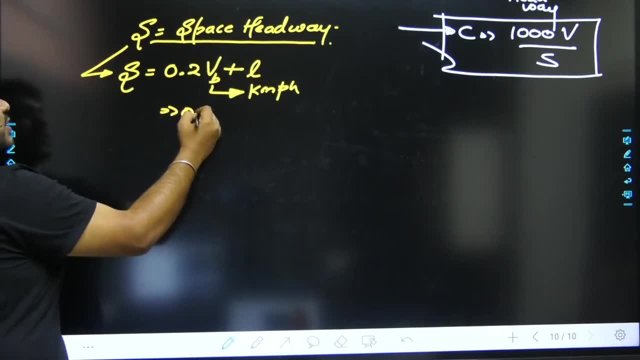 What was the meaning of this capital V? I mean this capital V means that its unit is in Kmph. I mean its unit is in Kmph. Very good, I mean you could have written this S as 0.7 small vb plus L. I mean this is in meter per second. 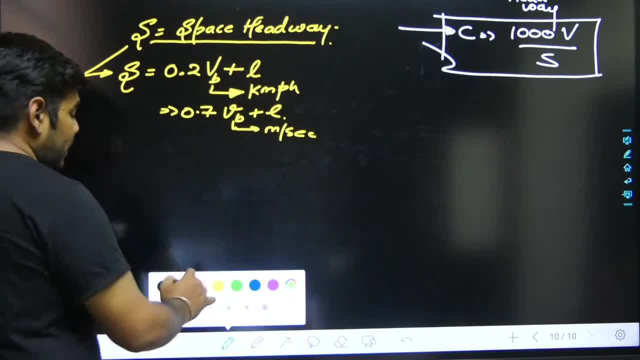 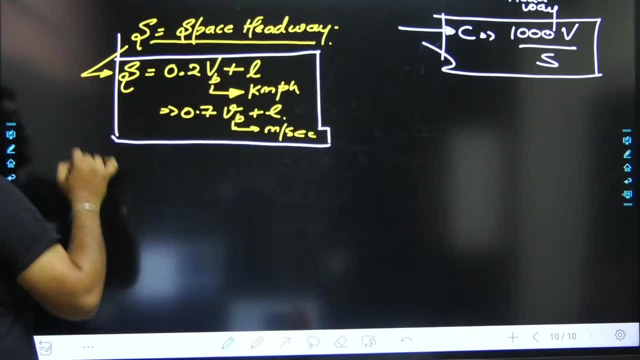 Okay, I mean, if it is like this, then I mean look here. I mean, if this is not sufficient data, then you will be using this value of S. If you have sufficient data available, then you will say: for S it is: S is equal to. 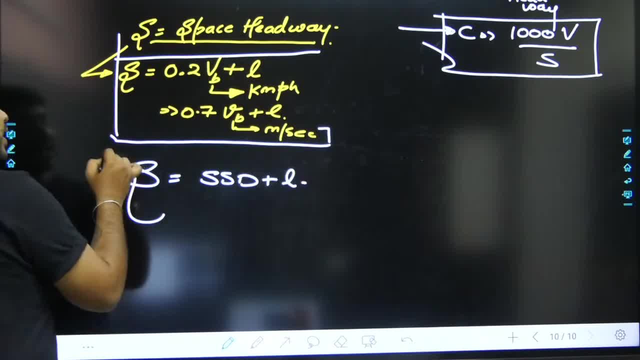 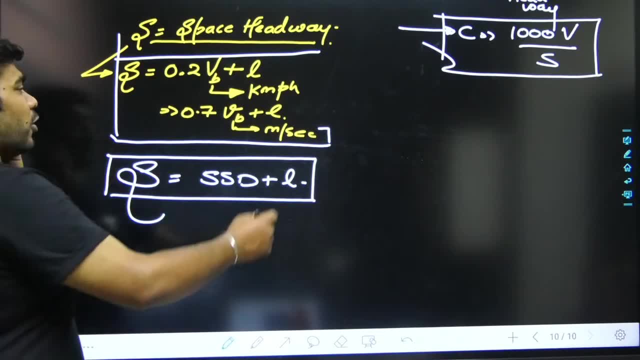 S is the plus length Length of wheelbase. I mean for S. you will say it is, S is the plus length of wheelbase. Okay, Now some people must be thinking: how, sir? I mean, where did you see this formula? 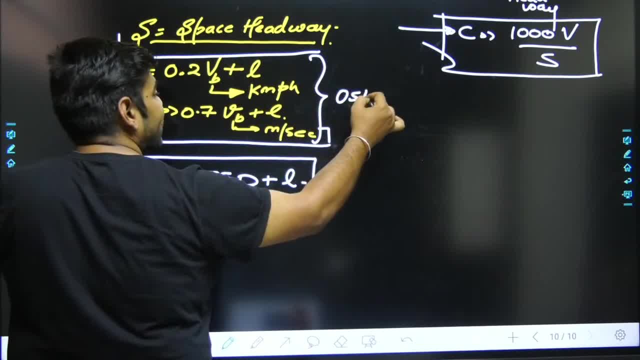 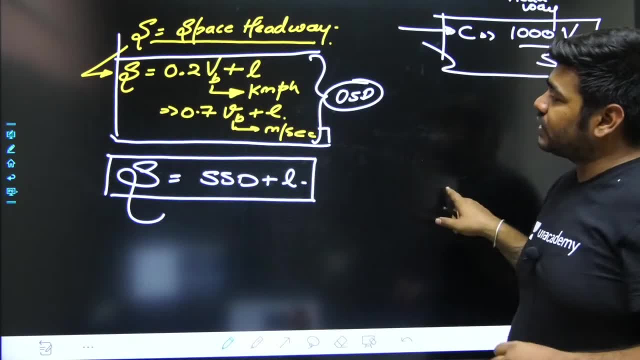 I mean, where did you see this formula? I mean you must have seen this formula in overtaking sight distance. Say: remember that day. Do you all remember that you have seen this formula in OSD? You have seen this formula in OSD. 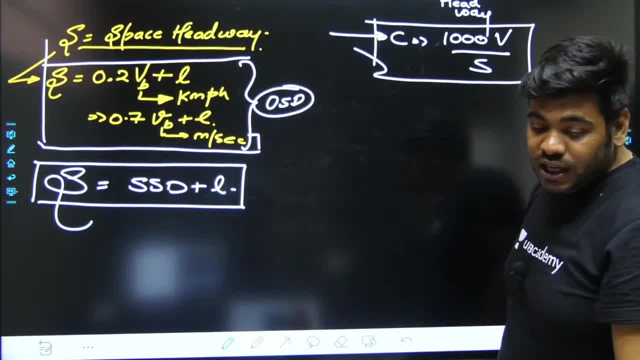 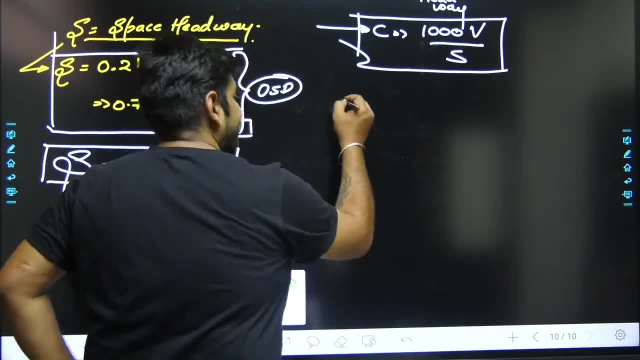 Okay, If you have seen this formula in OSD, then listen to me carefully. Try to understand. I am coming to the next thing. I mean: try to remember, So I will make OSD for you all. I mean I will make OSD for you all. 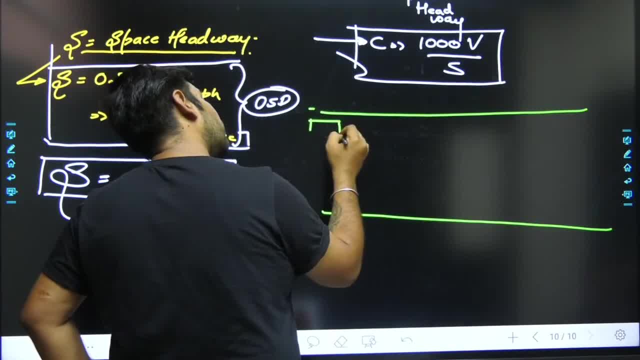 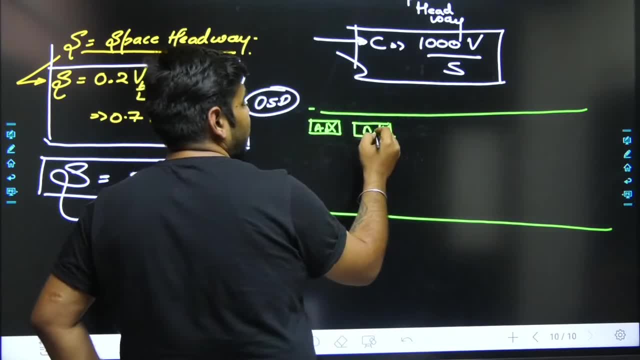 I mean, I am making OSD for you all. So I mean, see this Before overtaking. you used to see this vehicle A. Then this vehicle used to come here A. This was A1 position. This was A2 position. 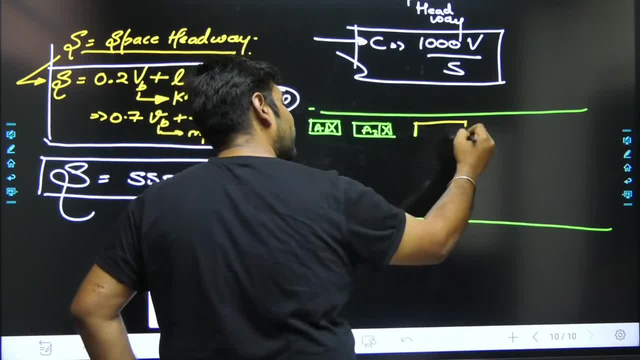 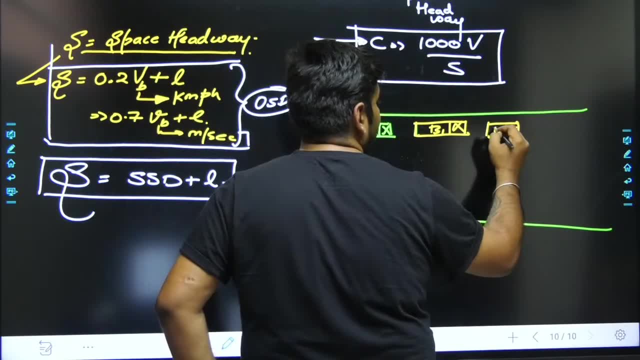 I mean he wanted to overtake this slow moving vehicle. He wanted to overtake this slow moving vehicle which you used to call B1.. Before overtaking: I mean after overtaking B2 position. Before overtaking B2 position: 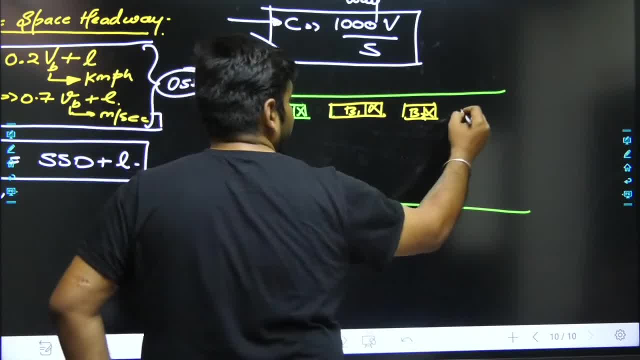 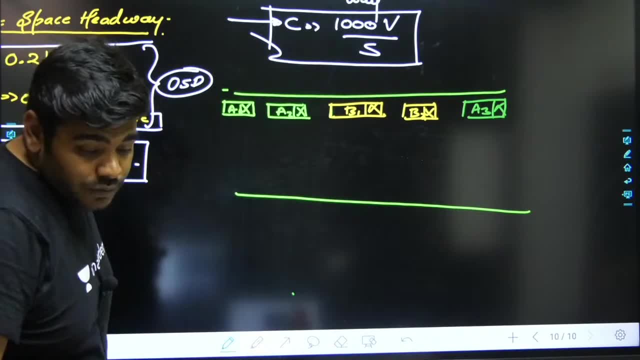 Before overtaking. I mean, at this same point of time, this position used to look like this, Which you used to call A3 position: Say yes or no. Say yes or no. Okay, If you remember this, if everyone remembers this thing, then I said that the S which you used to call. 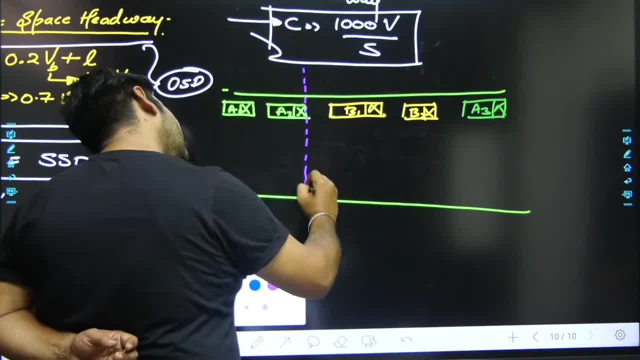 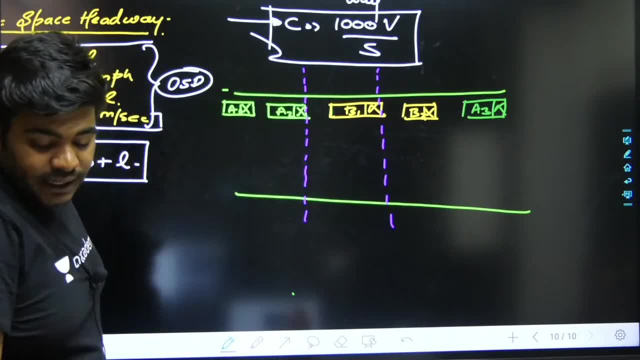 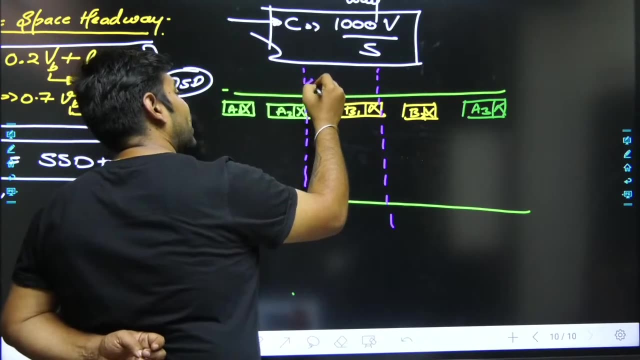 the difference between front to front. say yes or no. So safe distance maintained Before overtaking: Before and after overtaking: Say yes and no. This was safe distance maintained Before and after overtaking. Say ya, sir, You said it like this. 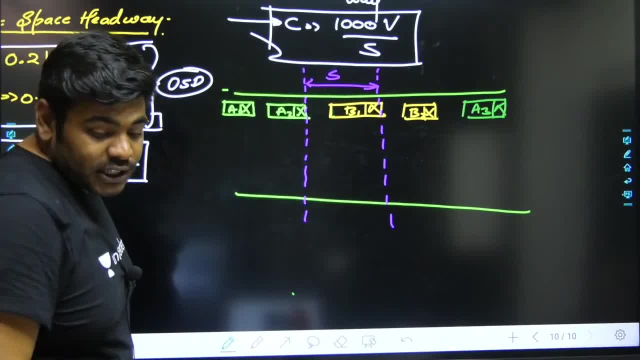 I used to call S. Say ya, bro. Say ya, sir. He used to call it as S. Say ya, sir. He used to call this S. Do you have a memory of this day That everybody remembers? This is what you would call, something like this. 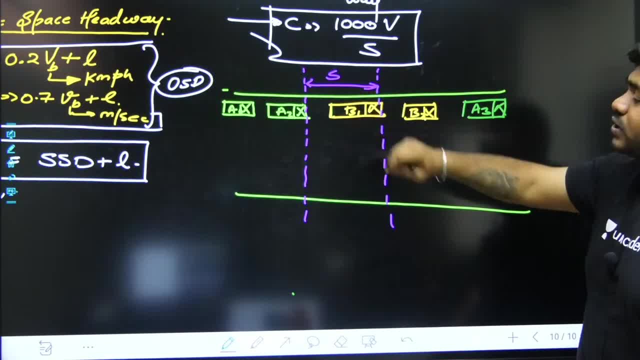 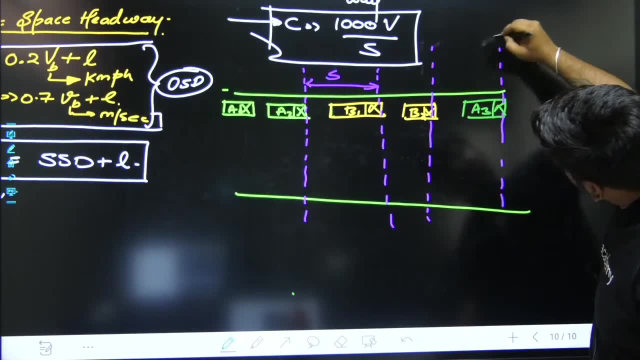 Before and after overtaking The distance you used to see. You used to call that S And I move here. see what you just saw. When we were talking, you used to call this part S, My stays healthy. distance After overtaking: 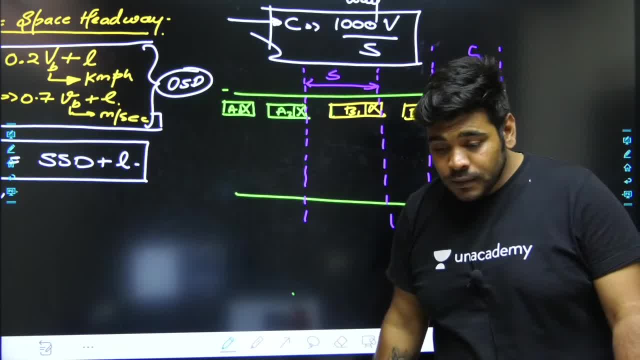 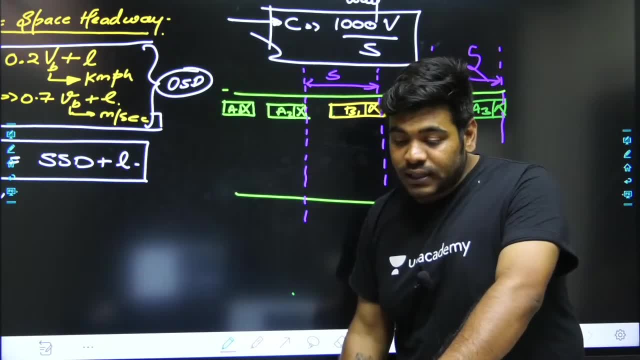 called it. You used to call this as S. did you remember everyone? did you remember everyone? if everyone remembered, if everyone remembered this thing, then I will see that it is so beautiful it is connected to OSD. it is so beautiful it is connected to OSD. if my words reach you. 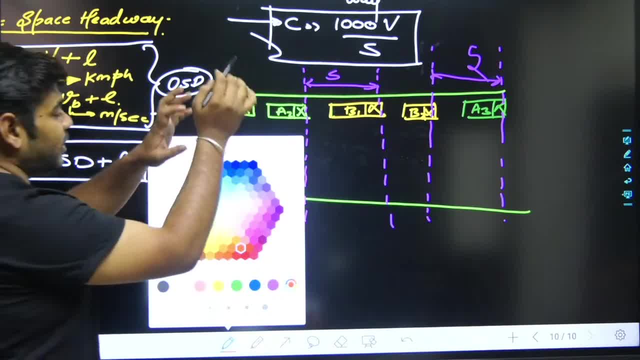 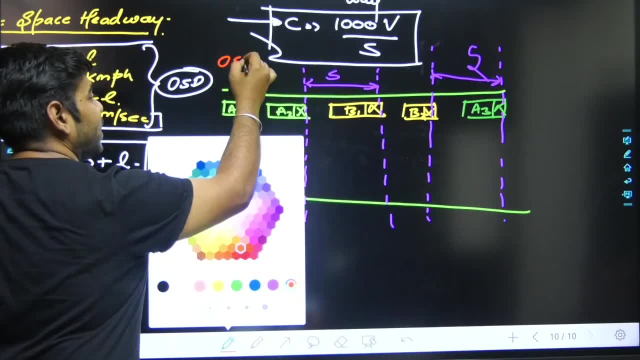 then tell me the way to tell. everyone can be different. if my words reach you, then you have to tell me that. yes, sir, we understood this thing. I said that I am talking about this. I said that this safe distance maintained before and after overtaking, I called it SSD. 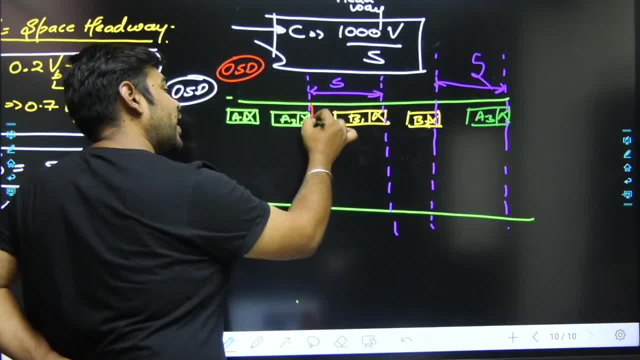 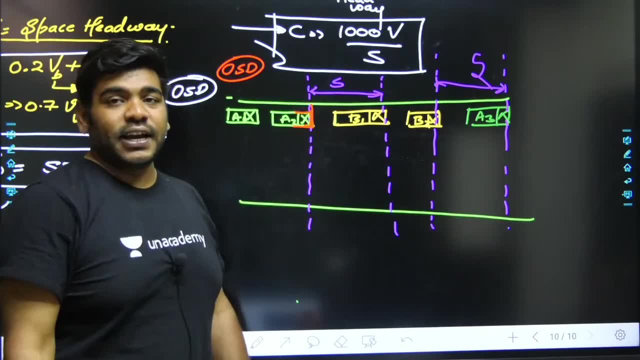 plus L. I said that see what is the meaning of SSD. what is the meaning of SSD if I am talking from its front? I said that no one will be talking in any book that the definition of SSD says that it will not connect like this. I said that all this is a matter of experience. 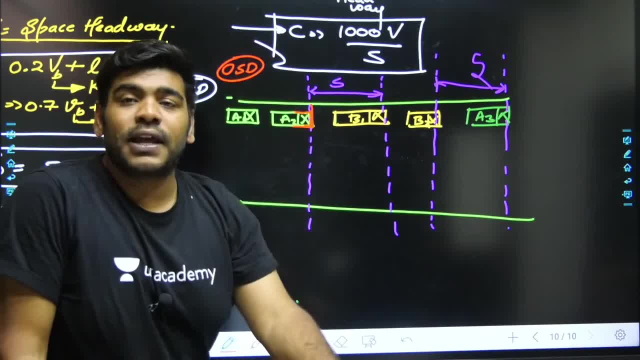 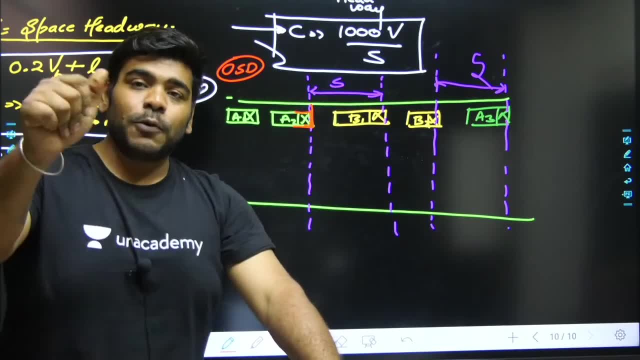 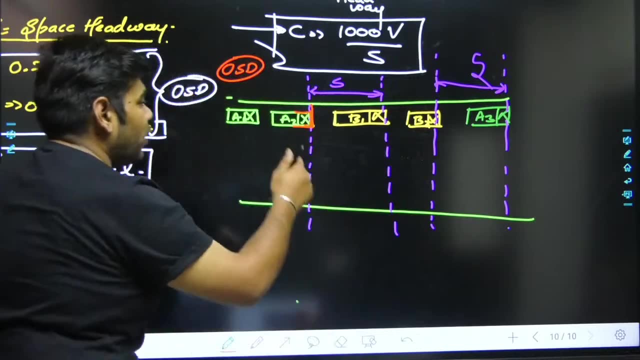 I said that. listen carefully. the definition of SSD says that it is the minimum length of road visible ahead to the driver. to the driver, To stop the vehicle just before the collision means SSD says that it is the minimum length of road required to stop the vehicle just before the collision. I said that is this. 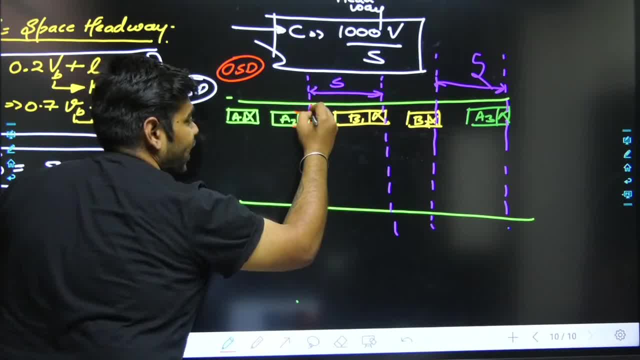 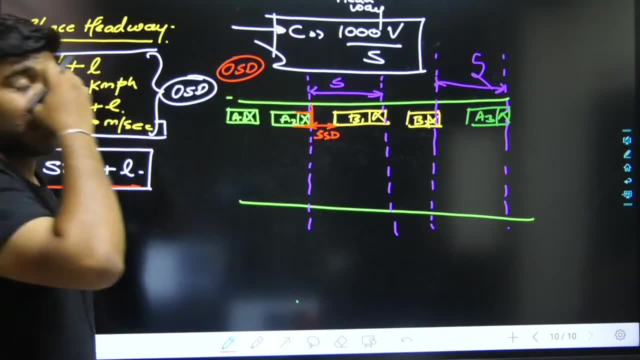 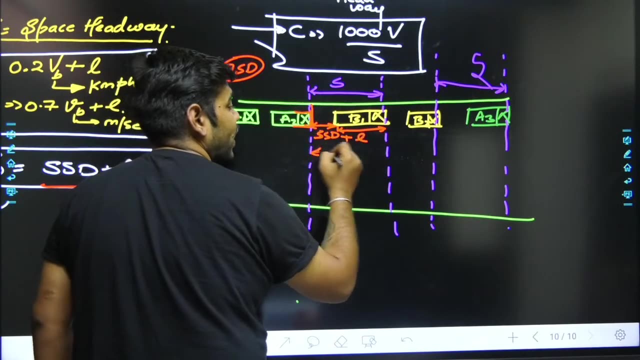 SSD. see this: before the collision: the distance required to stop this A2 vehicle from this B1 vehicle. it is your SSD, say yes or no. and I said that this remaining distance and I said that this remaining distance is the length of wheelbase. so you have written SSD. 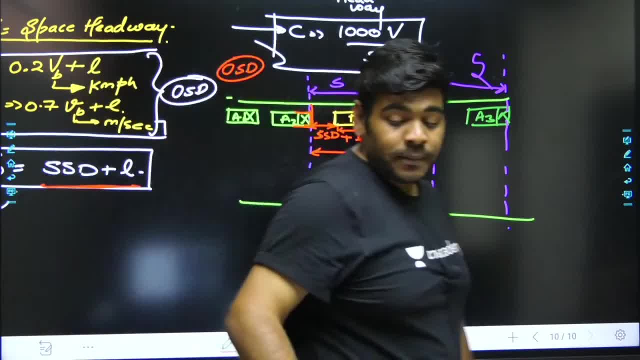 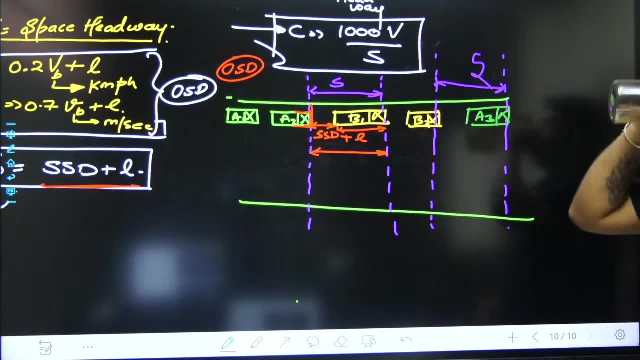 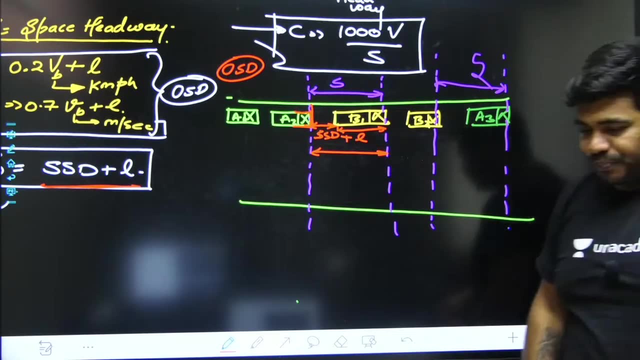 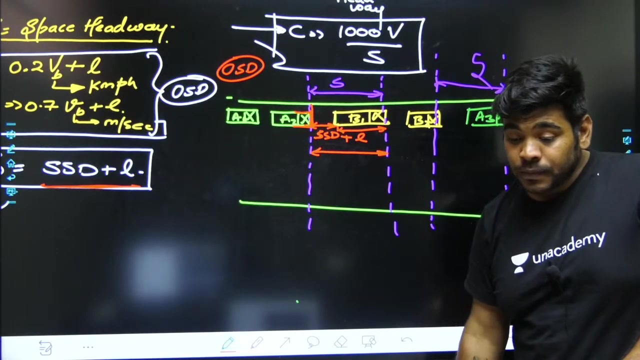 plus L. I said: is this my point? I said it reached to you or has not. I said that is this my point. I said that it reached to you or not. Will tell you quickly if everyone has reached me or not. is it? you Can reach up to everyone. 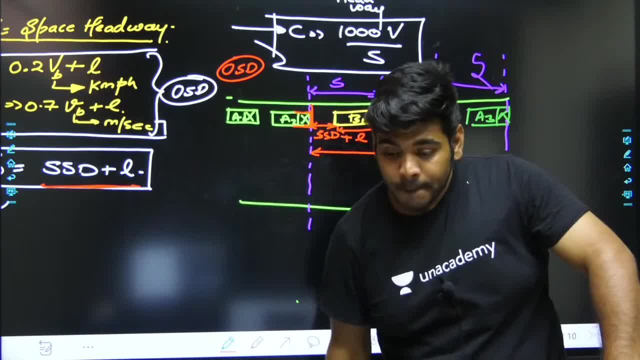 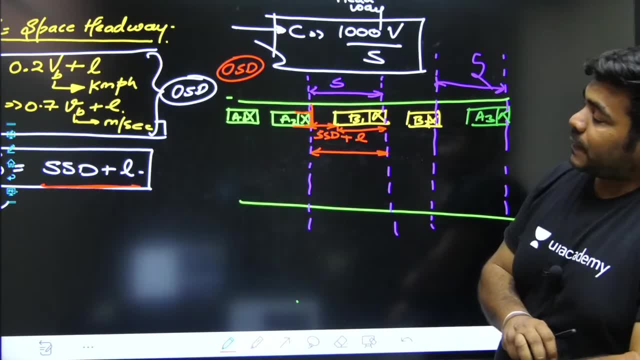 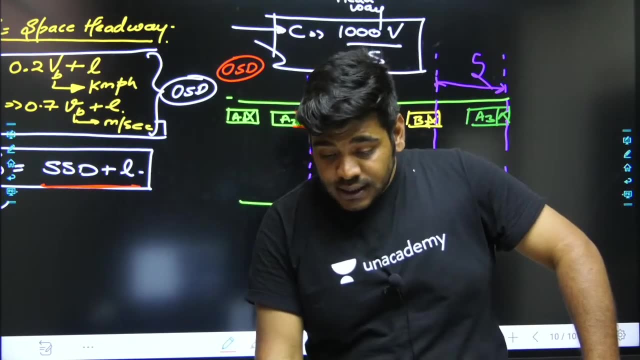 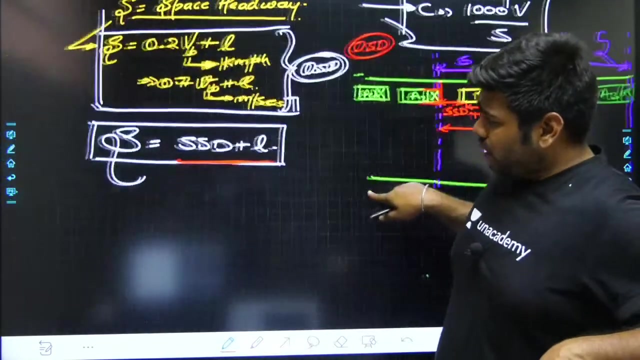 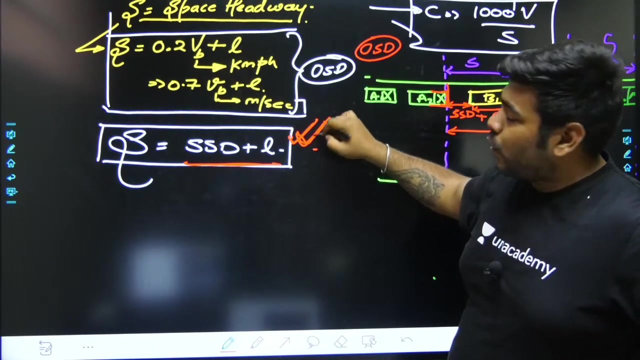 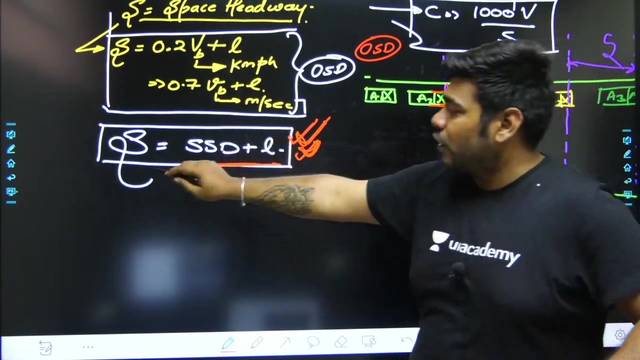 So I say this is equal to SSD plus L If both S obtain. which one is taken, This one is more preferable. Aman, this one is more preferable. If ever you are getting sufficient data, then use this formula, SSD plus L, to find the value. 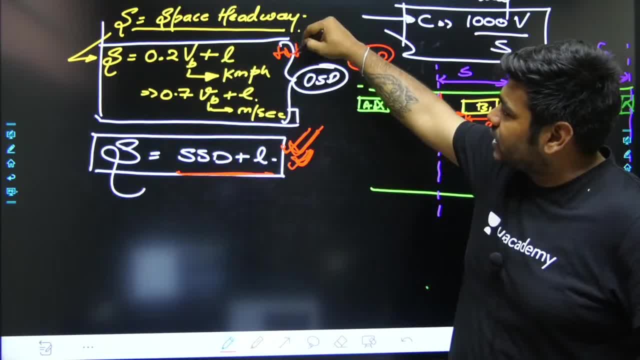 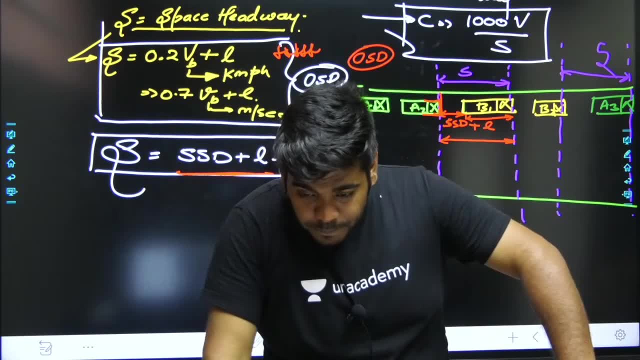 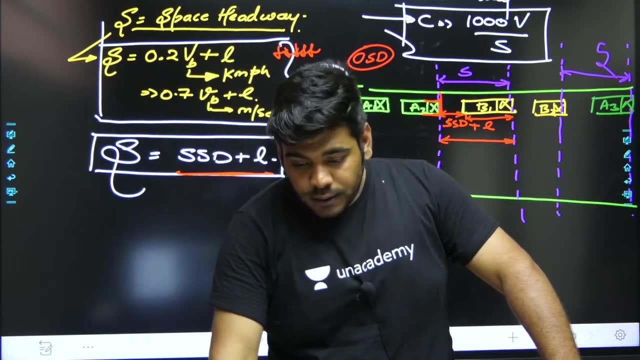 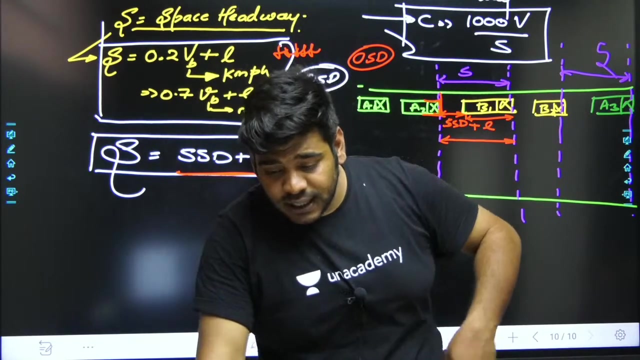 of S. This one is not favourable. we are using this when sufficient data is not given to us. When sufficient data is not given to us, ok. Ok, But isn't a dynamic problem where vehicle are moving to? Yes, vehicle are moving. 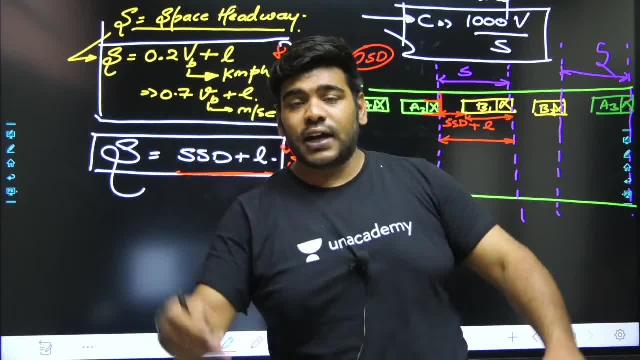 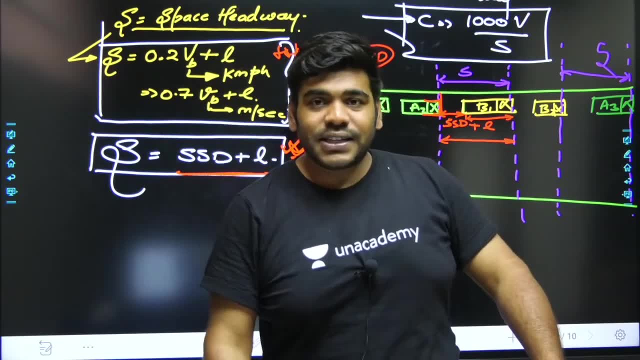 Yes, vehicle are moving. So what is the problem? We are considering that the whole like: listen to me, I am just listen to me very carefully, What I am considering here. I am considering an ideal case to find the capacity of a vehicle. 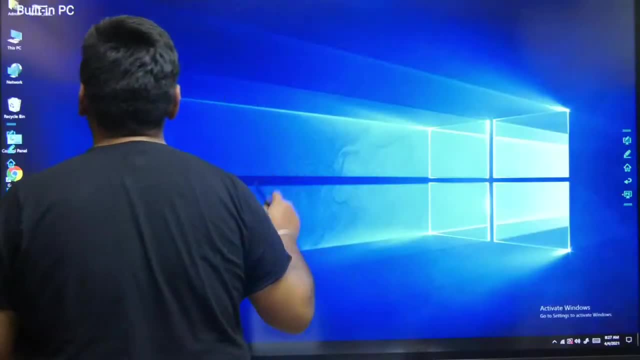 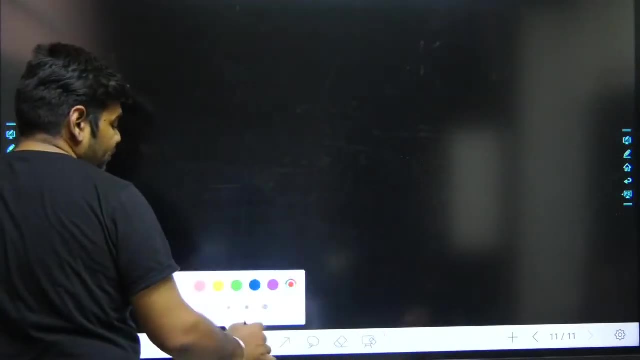 So if you are considering the capacity of vehicle, so what is happening over here? See here What is happening over here. Just see here carefully. What is happening over here. I am what is happening over here. Just have a look at this. 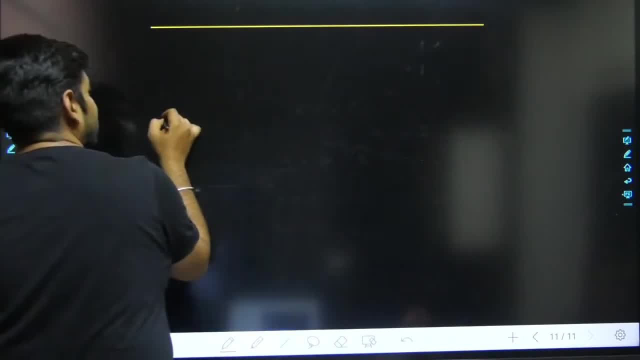 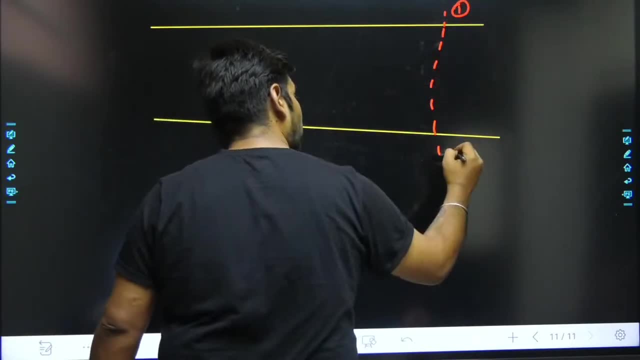 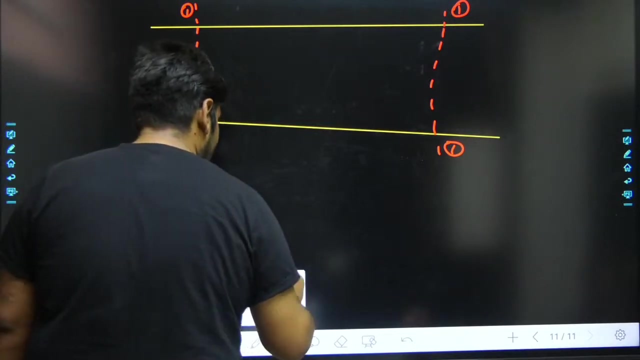 Maybe you understood this. I said: consider this section, consider this section. Now, this section is considered as one-one. I said: consider this section one-one, This is one and this is one. Consider this section one-one. We are considering the ideal case and, in ideal case, suppose four or five, how many number? 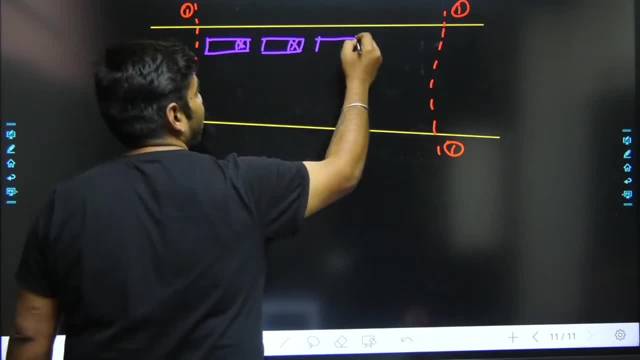 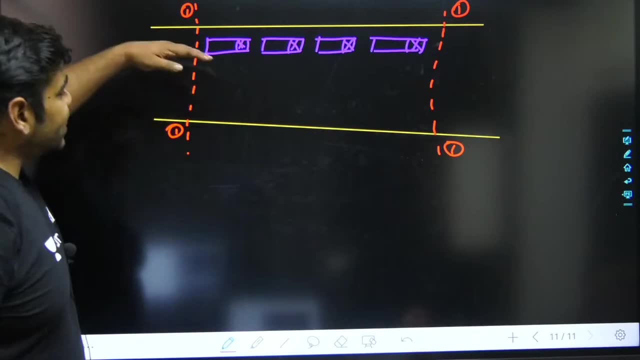 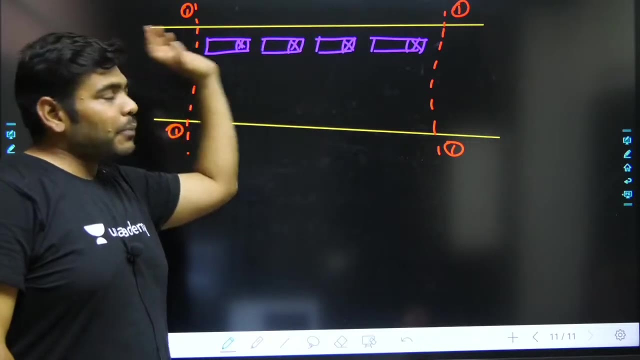 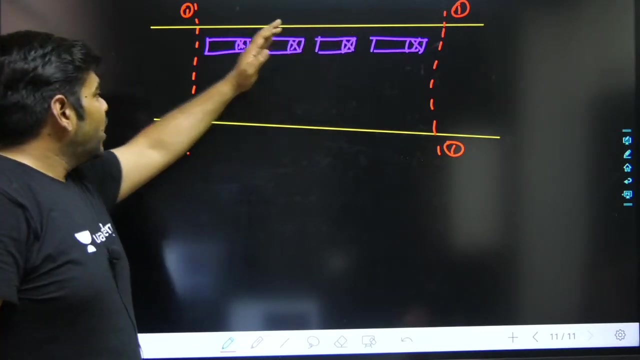 of vehicle- suppose I am considering an ideal case- and in a single lane maximum for vehicle can travel at a time in this section, in this particular section, now all are moving with the same velocity. yes, now all are moving with the same velocity. when all are moving with the same velocity, same velocity, now there. 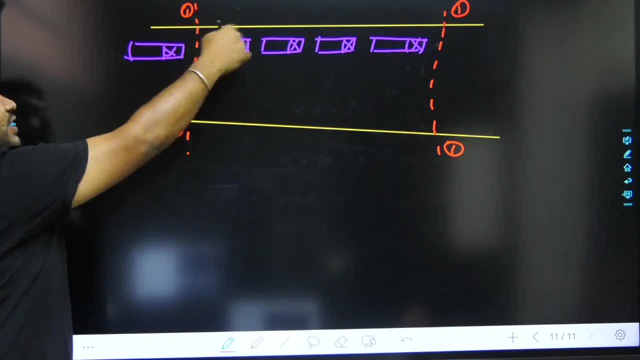 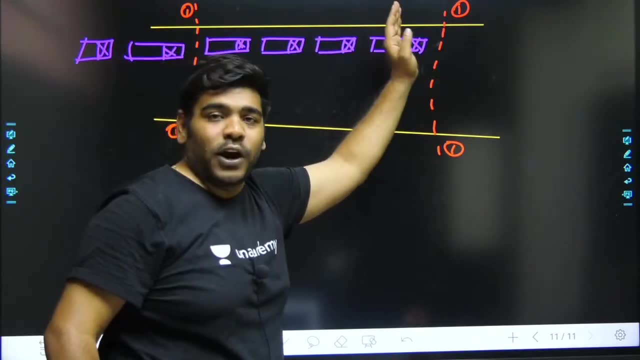 are more vehicle, there are more vehicle in this line, but we are considering the section one one, but we are considering the section one one. so in this ideal case, when one vehicle is crossing this, this point one one, so other point is entering from this one one. so each and every time when you are seeing this, you 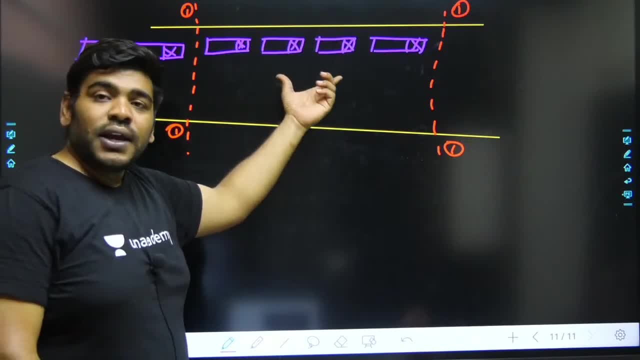 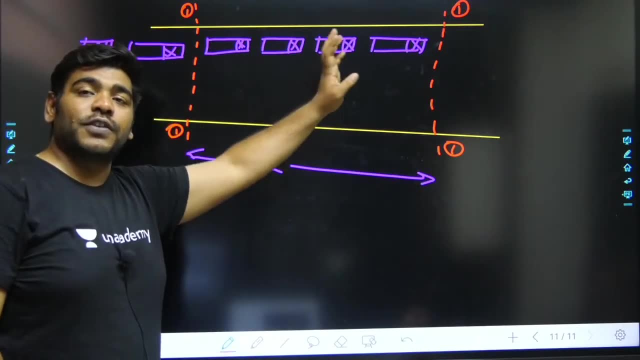 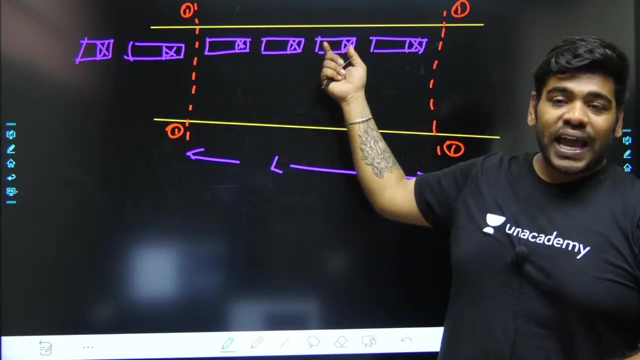 are not facing any change in in this section, in this particular section of length L, you are not facing any change when you are considering an ideal condition, when all the vehicle are moving with a velocity V abaya- someone may below huh Sonia to you, yes, it is a dynamic case, but we are considering the ideal situation over 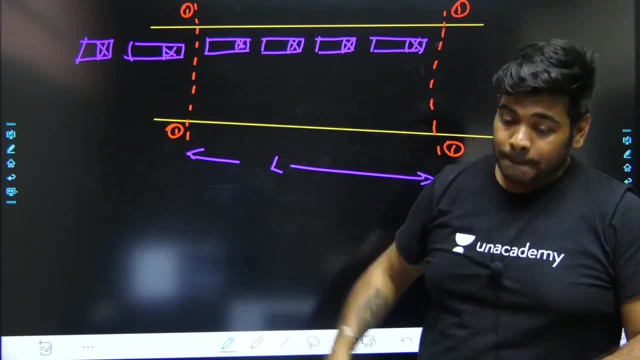 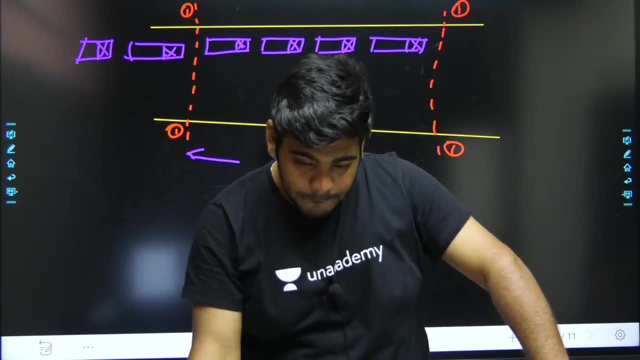 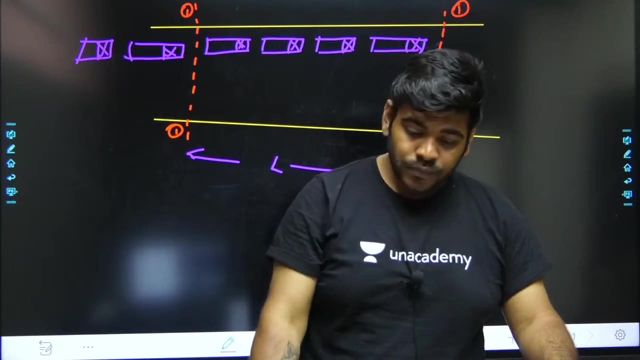 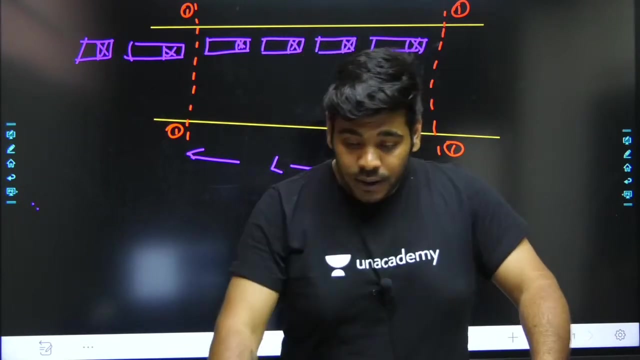 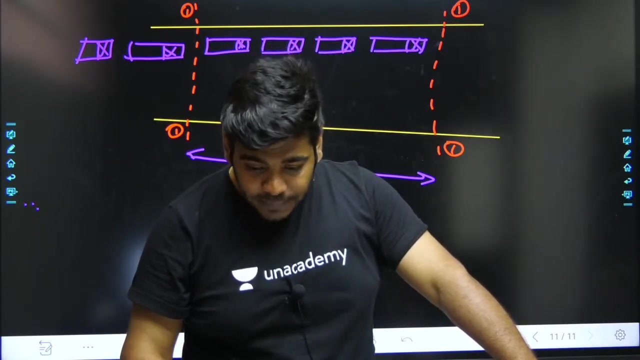 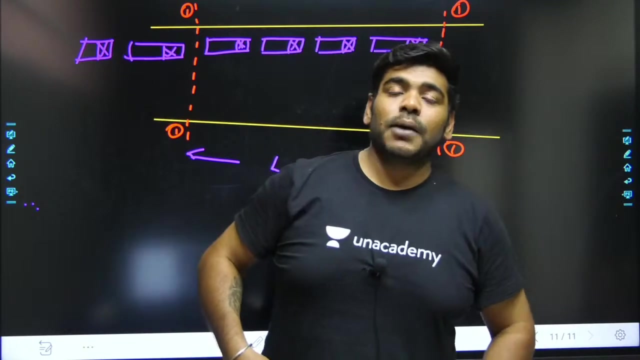 here to find the capacity of a particular lane. so now I guess I will go yes each and every time, whatever we are calculating, whatever we are calculating, we are considering the ideal conditions. fine to you. there are numbers of wheels that always look exactly the same and keep. 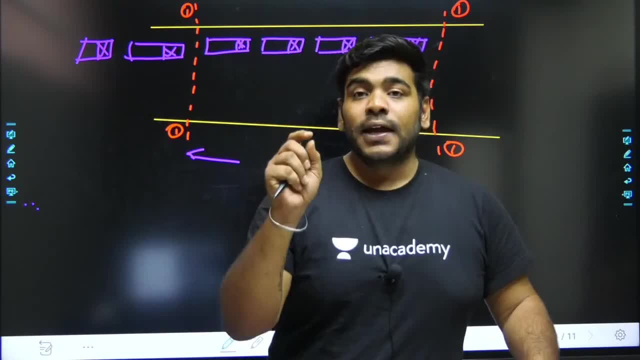 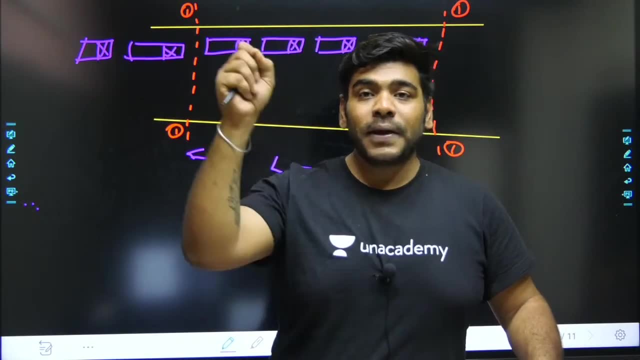 learning. possibly the particular vehicle will mapping enough ideal conditions here, much less we faster. anybody get multiplecakes. if you think that you are. Quincy means that now, if you choose traffic rate undernat the valley and product Referziałah, here you have quejas, VZ and capacitor meansAN else you are talking. traffic capacity means that here we have the two and the start data happening and qj means the MTZ and Capacity. 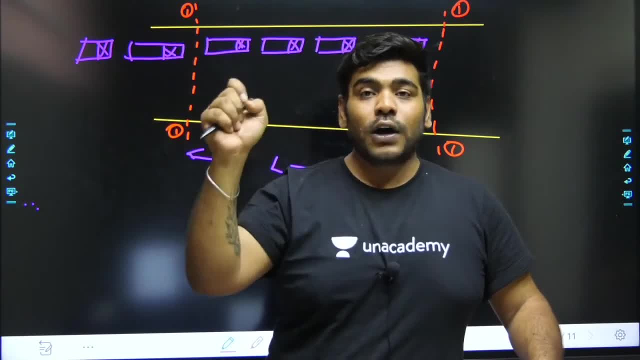 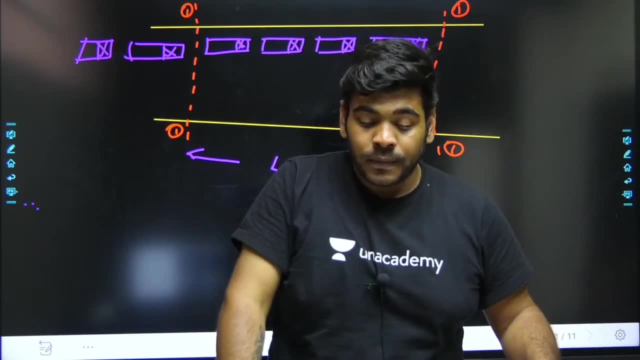 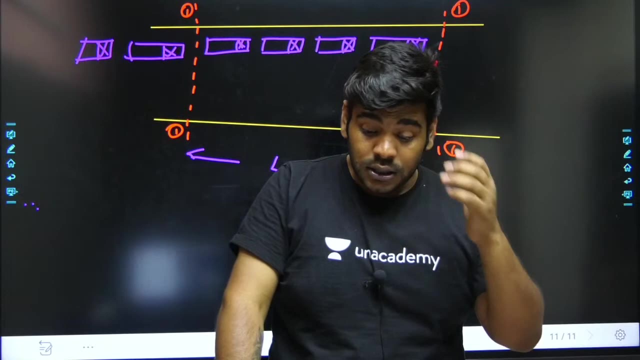 talking about capacity, then we are talking about r per vehicle, and when we are talking about kg, then we are talking about km per vehicle. This is the difference. Do you understand? Like the session quickly. You can't reach 100 by liking. What is the difference between? 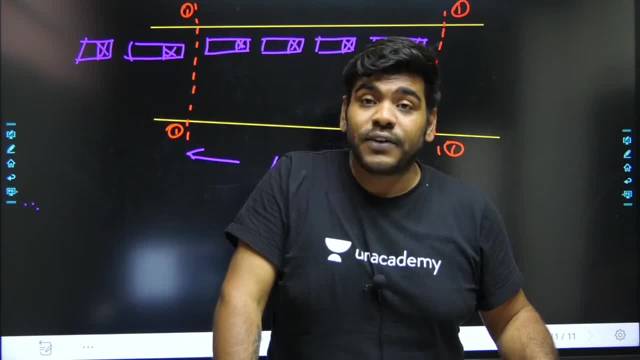 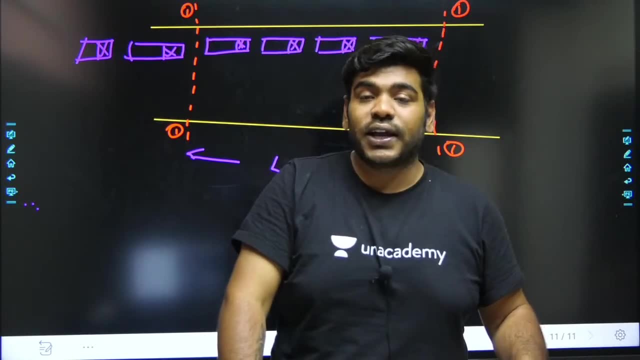 C and Qmax. There is nothing. There is no difference between C and Qmax. We call Qmax C. Qmax is the theoretical capacity. just listen carefully to what I am saying. Qmax is theoretical capacity and I am calling C practical capacity. C is practical capacity. 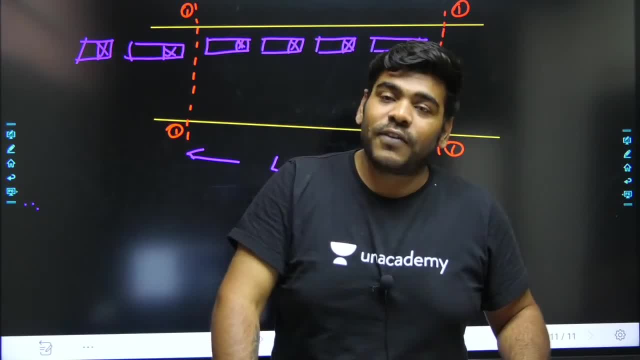 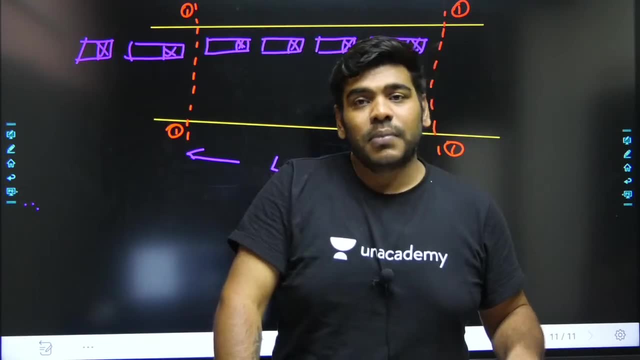 and that is why I am representing it with C. Qmax is also a maximum value of your flow. c is also the maximum value f curve and maximum capacity. C is always in practical capacity and what we can see is that I am calling Knowledge Qmax, Edward, Optimum as theoretical. 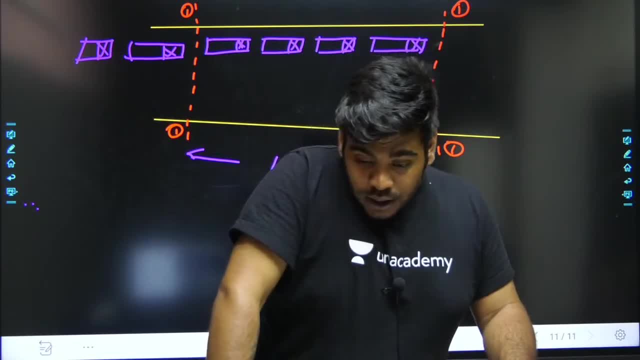 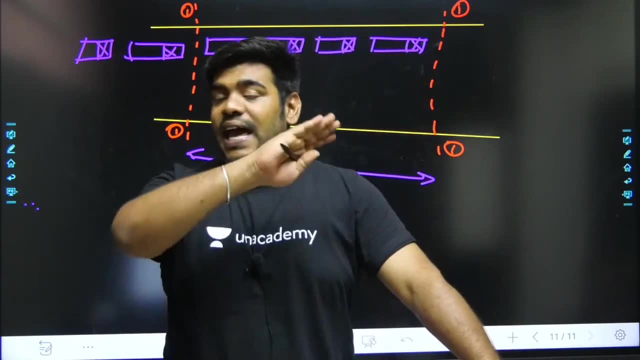 maximum capacity. capacity, theoretical maximum value: yes, we will keep it after 12 o'clock tomorrow, don't worry. don't worry, we will keep it after 12 o'clock tomorrow. even if everything is clear, tell everyone yes or no. even if everything is clear, tell everyone to like. 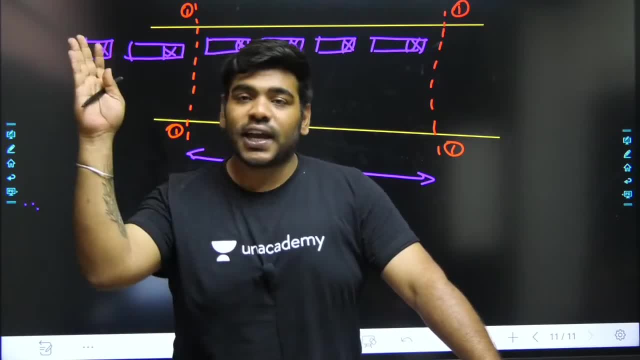 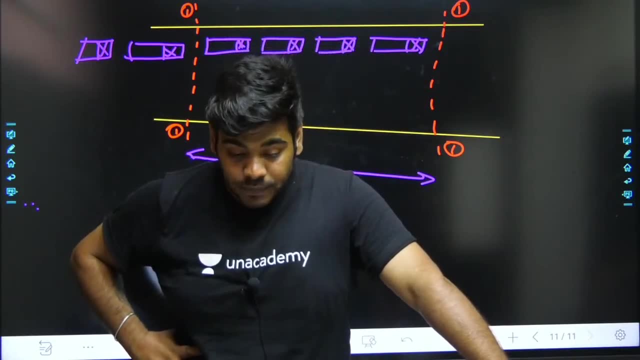 the session quickly. like the session quickly. everything is clear. whatever has been told till now, everything is clear. if anyone has any doubt, then you can ask me once else. we go to see a new concept or we finish today's class here. from tomorrow we will see. 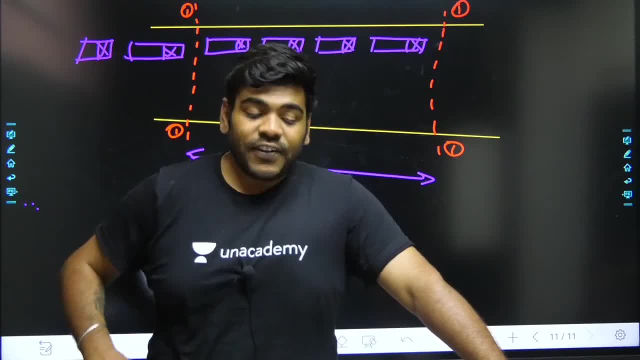 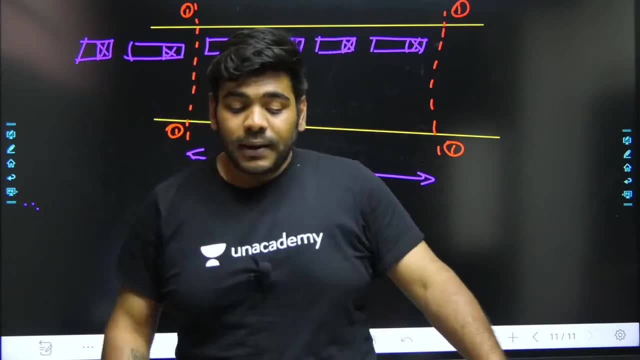 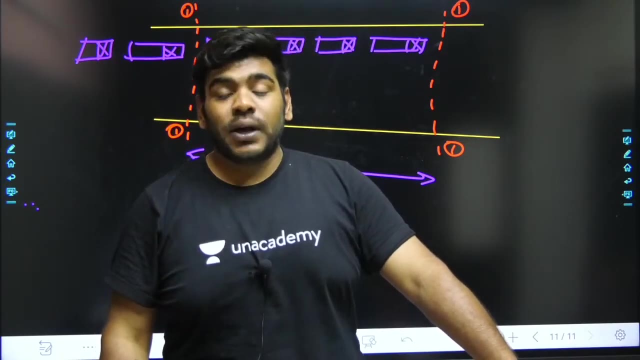 I said: you have seen the traffic characteristic. when you spoke about traffic characteristics, listen carefully, listen carefully what I am saying. I said: listen carefully to me, listen carefully to me. what am I saying, listen to me carefully what I am saying. 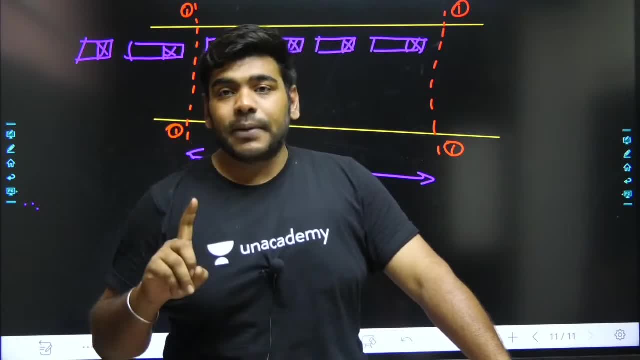 listen carefully to me. I said once you said what you have learned till now. I saidَّ, talking about this traffic, what we have seen in traffic engineering. I said we have divided traffic engineering into three parts. In our traffic landscape, there is one characteristic think in terms of today's company: what you 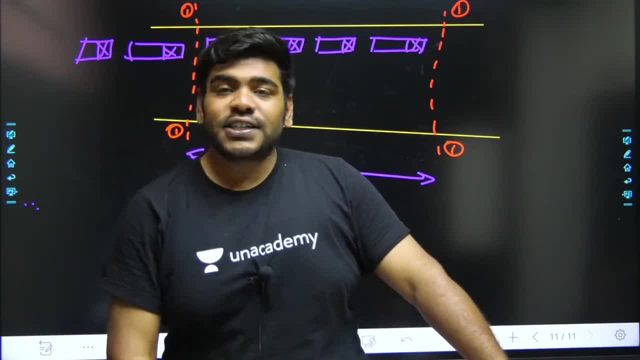 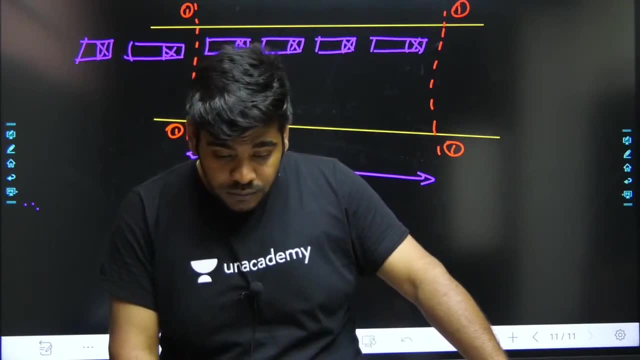 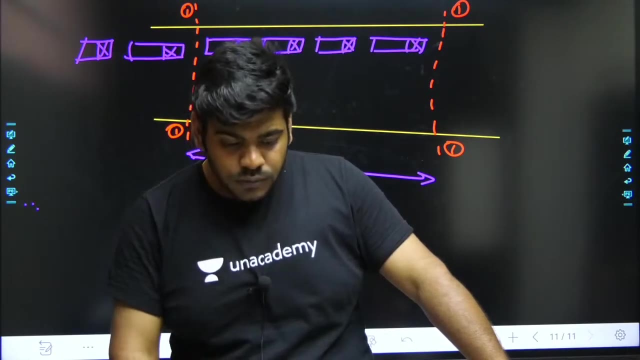 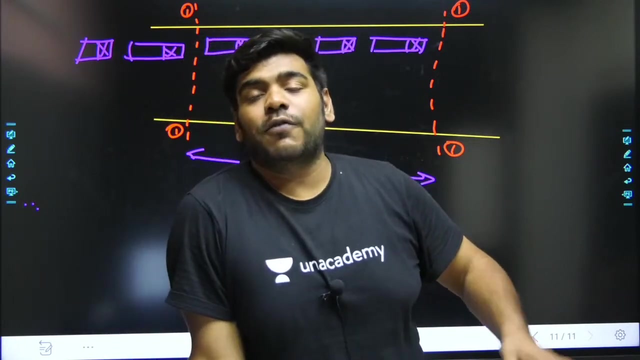 The first part was about the traffic characteristics. so what did we talk about in the traffic characteristics? So the first thing I said was I said look carefully here. I said when we talk about traffic capacity, sorry, I said when we talk about traffic characteristics, I said what are the various characteristics, those who are going to use? 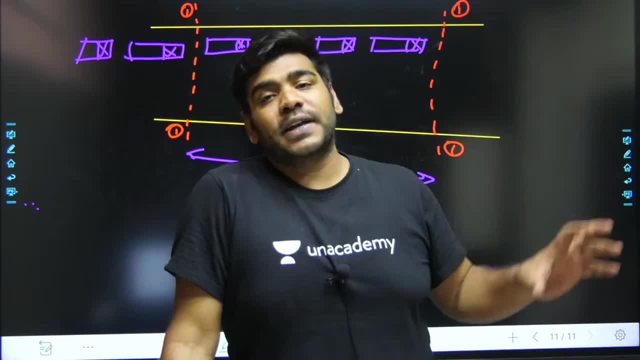 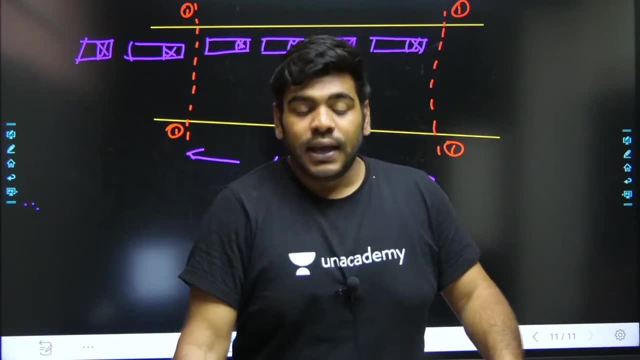 those who are going to use, those who are going to become the part of the traffic. so which part were going to be made? I said your vehicle part was going to be made and your human part was going to be made. that's why we talked about road user characteristics and we talked about which. 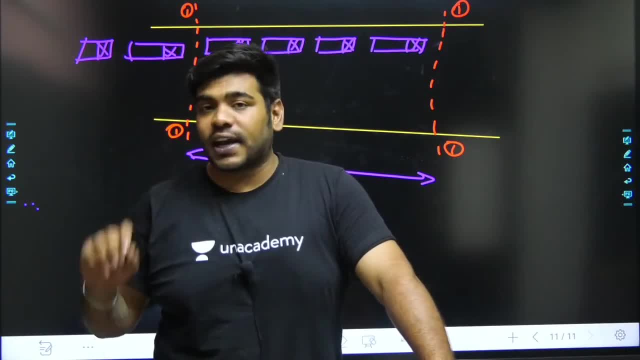 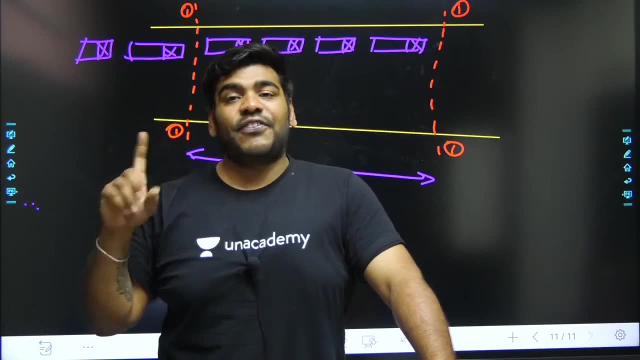 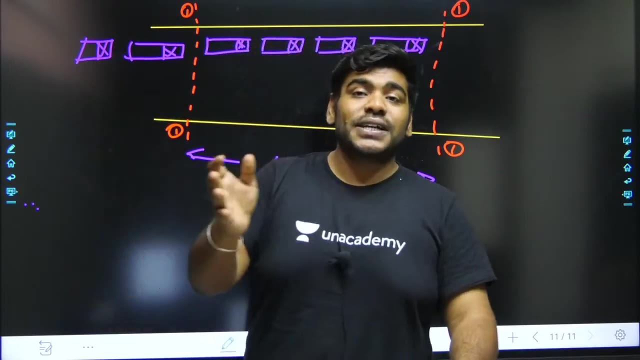 We talked about vehicular characteristics along with it. so this is the whole traffic characteristic. then we talked about which. We talked about traffic speed and analysis. so here we talked about various speeds and did various analysis that at what speed our vehicles will be moving and how their speed will be judged. 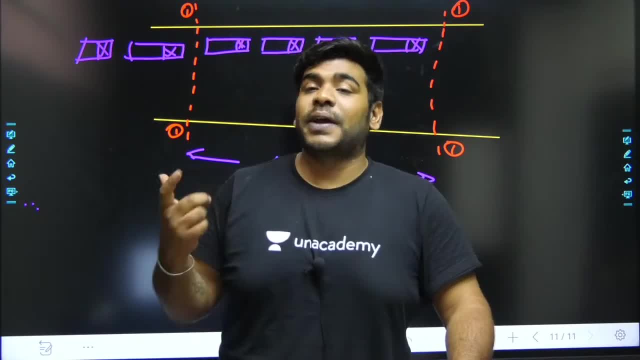 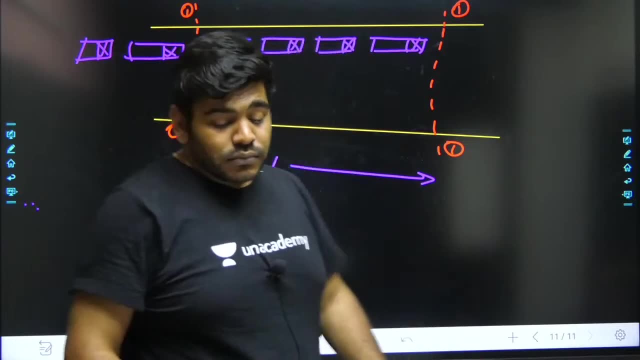 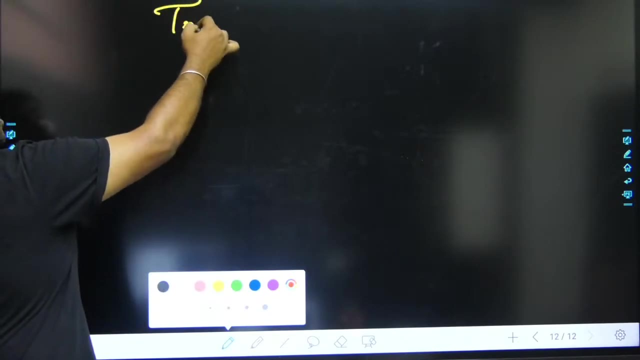 can there be maximum traffic volume, maximum traffic density, maximum velocity? you did all these things. next, the topic which is going to start from tomorrow. the topic which is going to start from tomorrow: we will talk about traffic control and devices. next, we will talk about traffic control and devices. 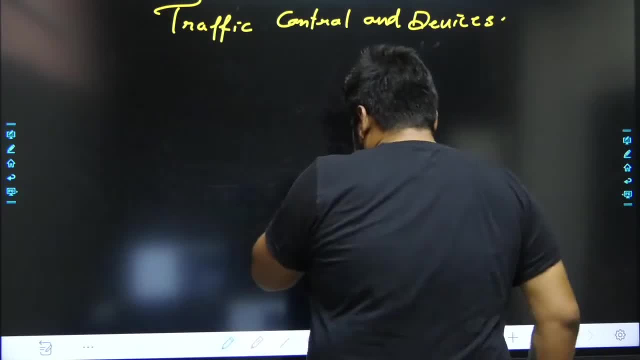 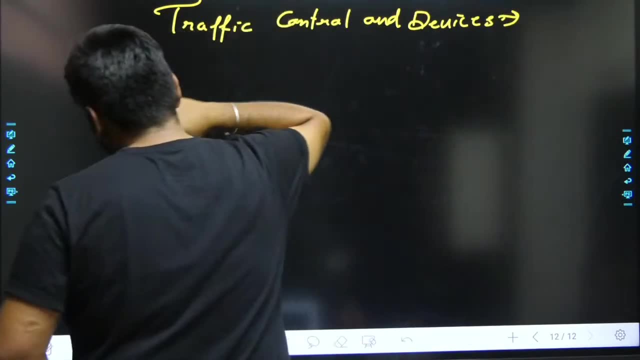 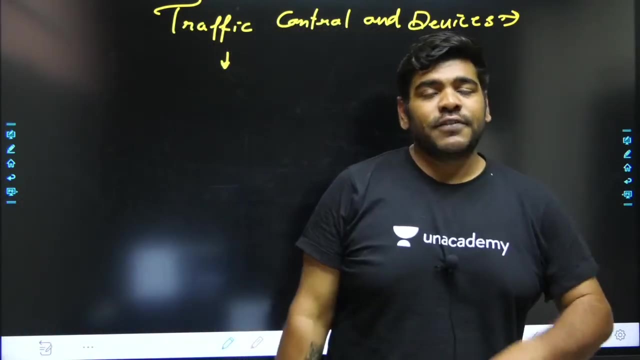 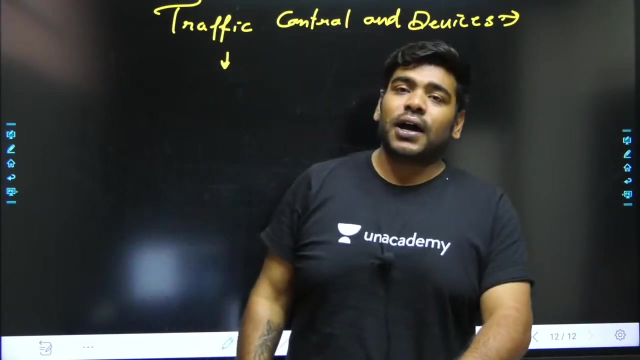 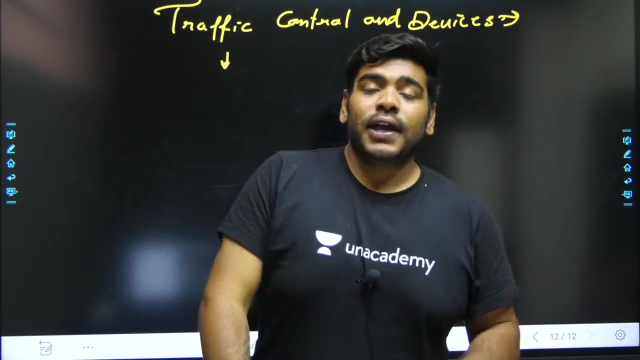 we will talk about traffic control and devices. ie, we will talk about traffic control and devices. what are the various devices which are used to make traffic more soothing, to make traffic? How do we design signals? and I am telling you that now you will love traffic engineering. 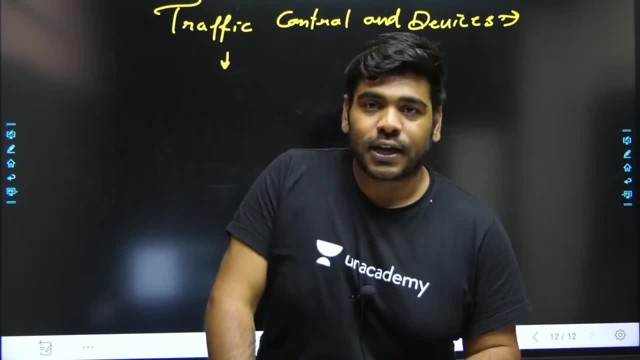 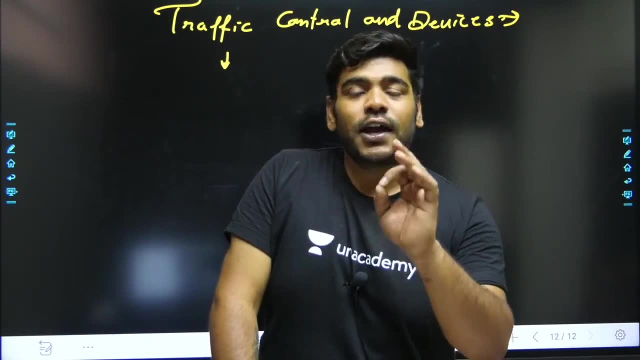 I told you that you will fall in love with Geometrical Design, and you fell in love with Geometrical Design. I told you that tomorrow you will attend two classes and the day after tomorrow you will attend two classes And you will start saying that when you go out on the road you will say thank you every time. 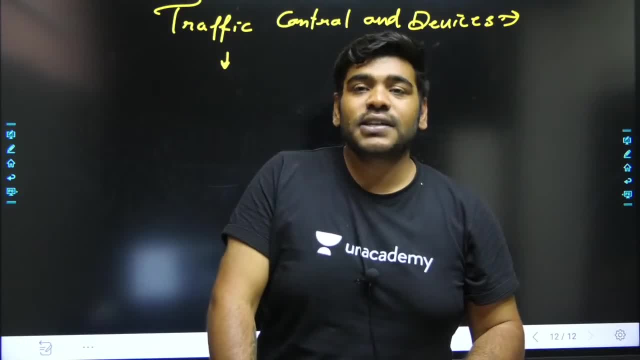 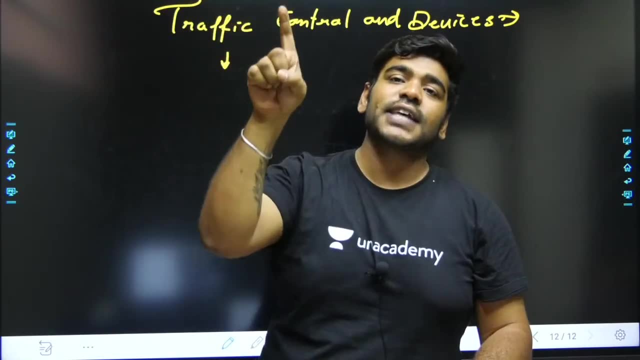 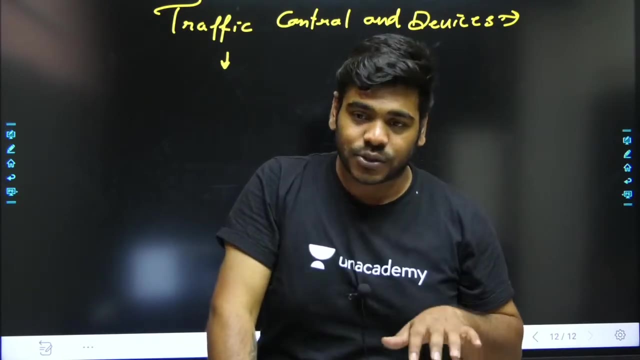 Sir, I will tell you how to design a signal. Every time when you will see a signal, you will remember that to design a signal, is this cycle running properly? Is this signal cycle running properly? Should this be red time or should this be green time? Every time, you will be saying that I will take traffic control and devices to this level. 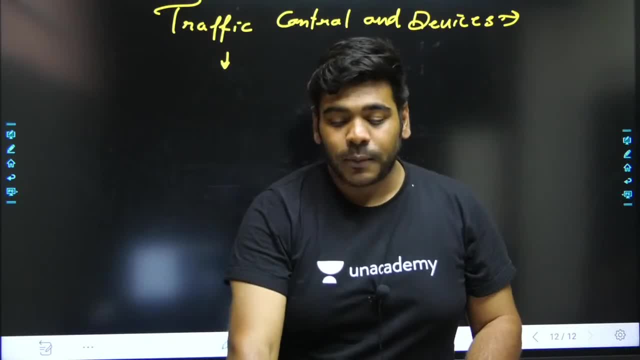 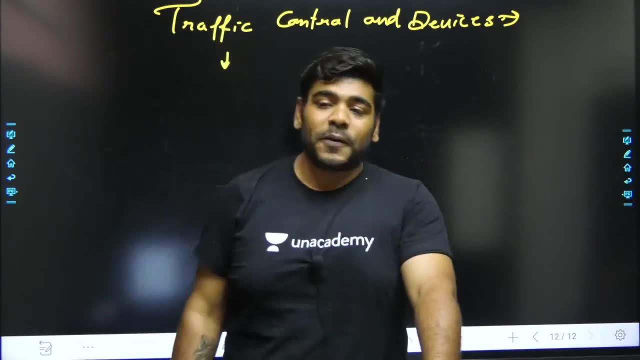 Okay, so stay with me. One student asked that, sir, has this thousand flexible pavement design been done? No, flexible pavement design has not been done yet. Pavement design has not been done yet. After this pavement design will start. I said that. one student asked that, sir, why thousand has been multiplied. 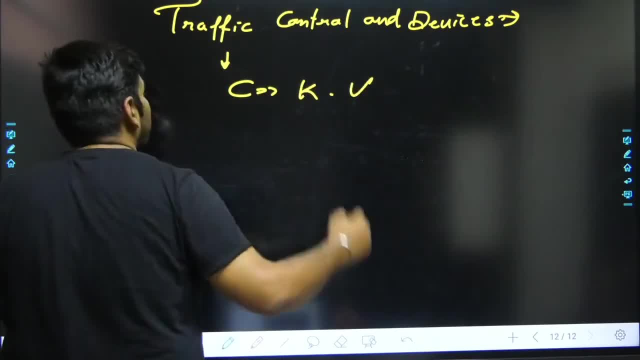 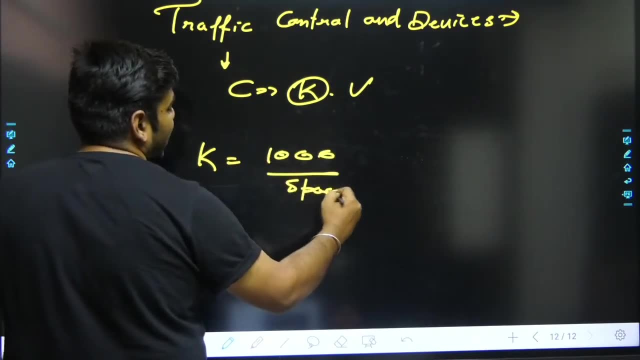 I said that: see here, c is equal to what is k into v. I told you k. I told you that k is traffic density. You always say thousand divided by space headway, Because here space headway was available in meters. That is why I talked about it. 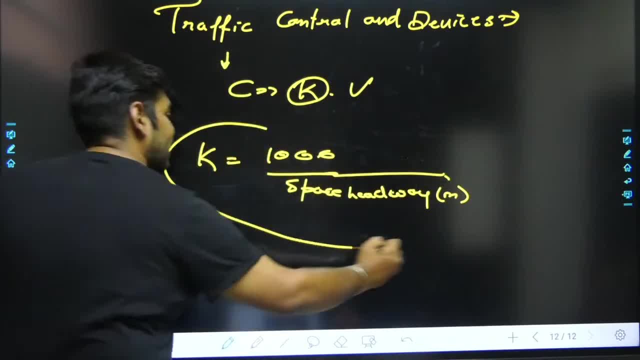 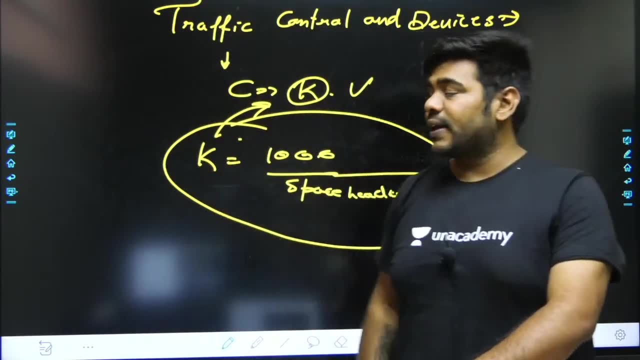 I mean, space headway was written like this, only So. we have written it like this, only. Nothing else is written Instead of k, thousand divided by space headway has been done. Aman for you. Okay, that is why thousand has been multiplied Thousand by space headway. 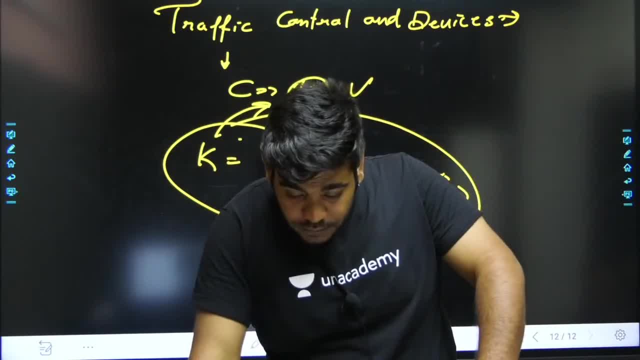 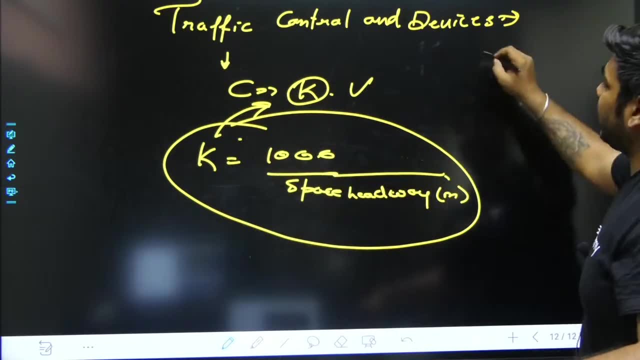 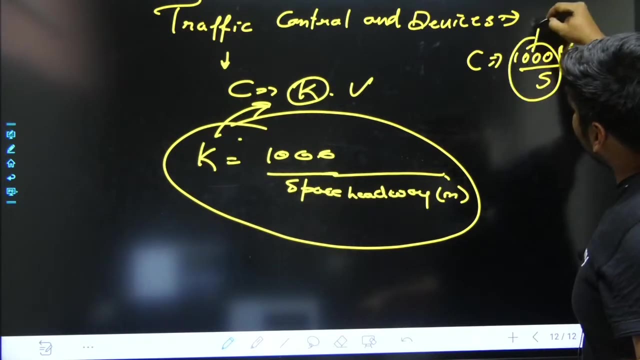 Space headway was in meters, I had to convert it in meters. Thousand k by s is not written. Thousand v by s is written. C is equal to thousand v by s. What is this? This is exactly k. only Say yes. So what is this capacity? 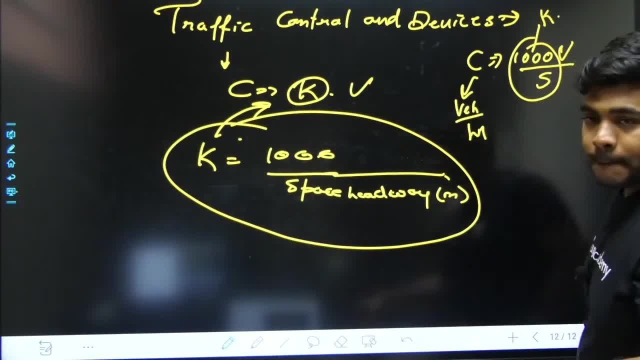 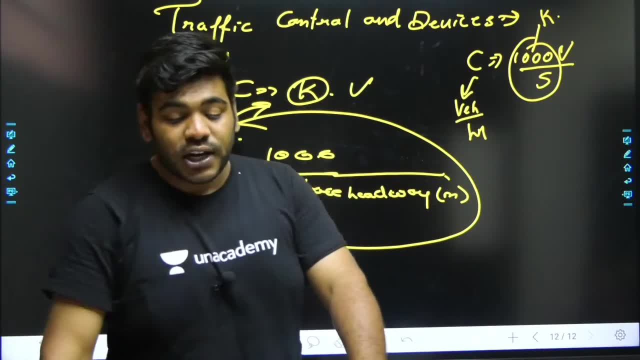 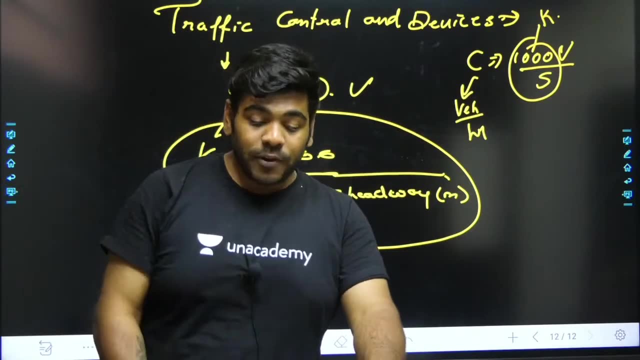 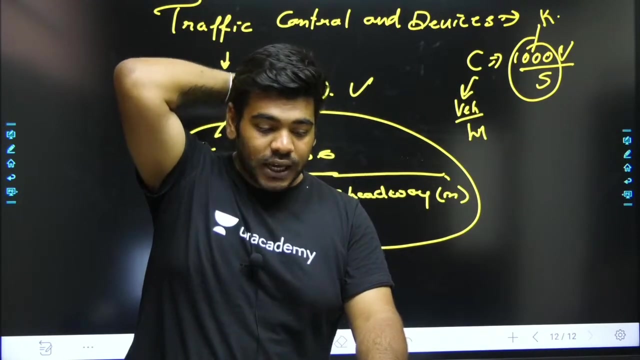 This will come on vehicle only. Whatever happens, Make it environmental. Environmental is going on. Environment is going on. Environment is already going on. Okay, so let's finish today's class here. So let's see what we will study from tomorrow. From tomorrow, we will study traffic designing. We will study traffic control and devices. 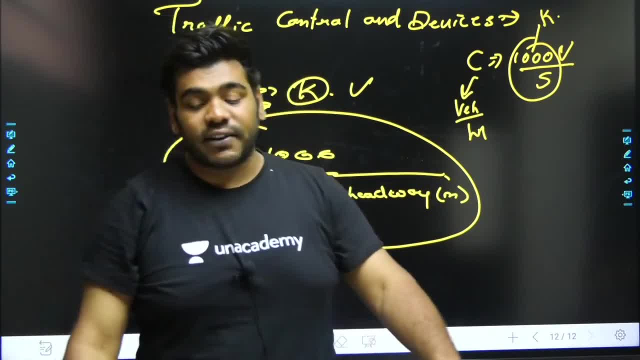 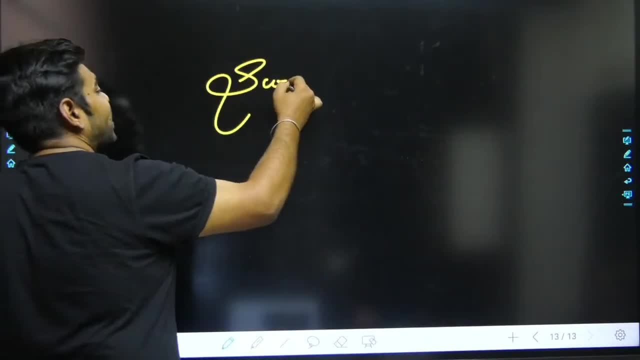 So let's meet you all Tomorrow. I am going to give you a practice session of surveying- Those who are watching for the first time. Let me tell you one thing: We will see surveying here. You can see surveying on PlanetGate channel. We are reading: surveying on PlanetGate channel. 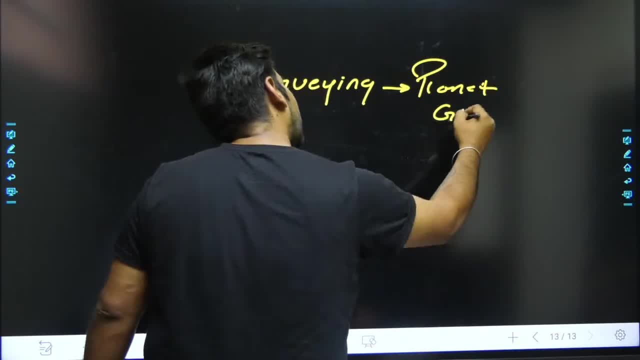 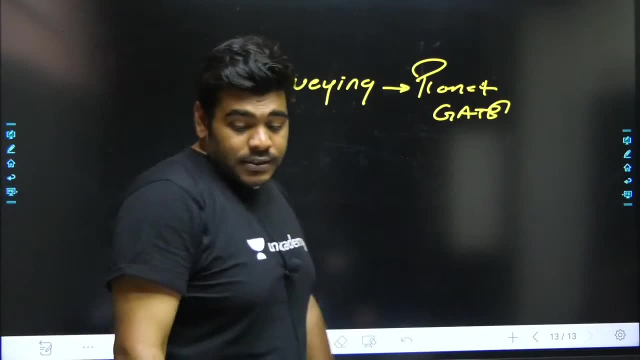 So you guys go there and subscribe to that channel And, at a different level, we are seeing surveying there. We are seeing surveying in a lot of depth, So you can see surveying on PlanetGate channel. Okay, Okay, So okay, guys. thank you so much.